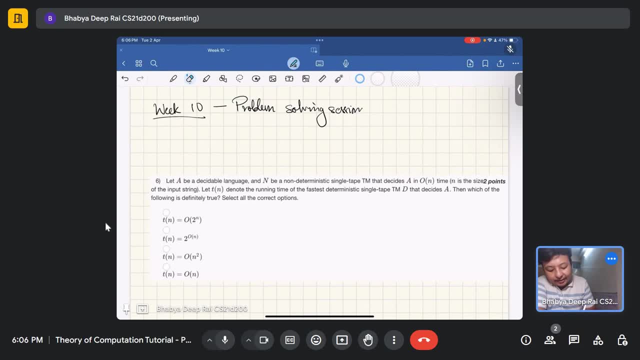 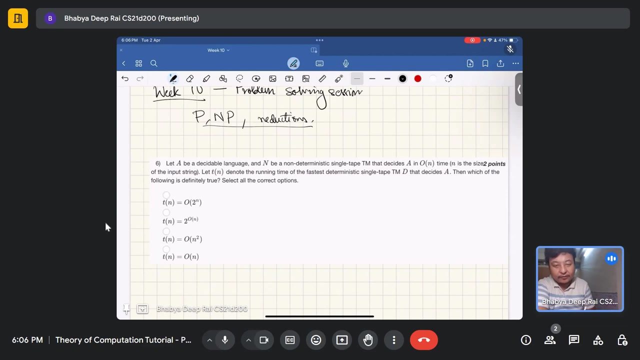 What we'll do now is actually in week 10 we focus on the classes P, NP and talk about reductions. We'll go into detail later on. We'll solve a few questions on this. But before we move on that, we shall first solve a few questions from the assignments of week 9.. 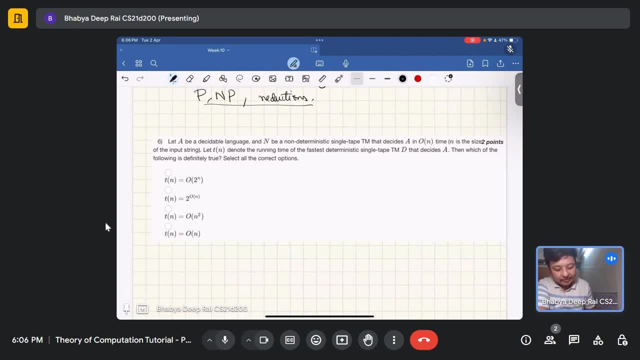 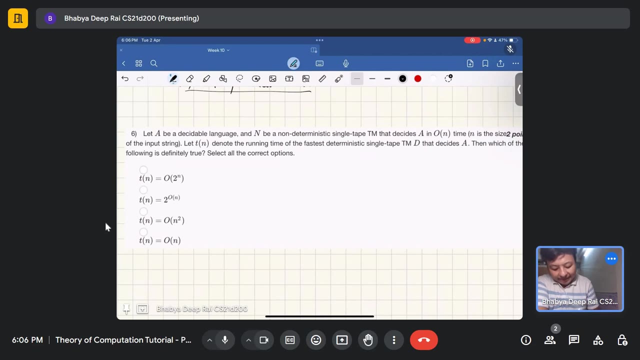 So here are a few questions from assignment of week 9 which I've handpicked, which seem to be on the tougher side, So let's begin. So this is question number 6 from assignment 9.. It says: let A be a decidable language and N be a non deterministic single tape Turing machine that decides A in linear time. order n- time. 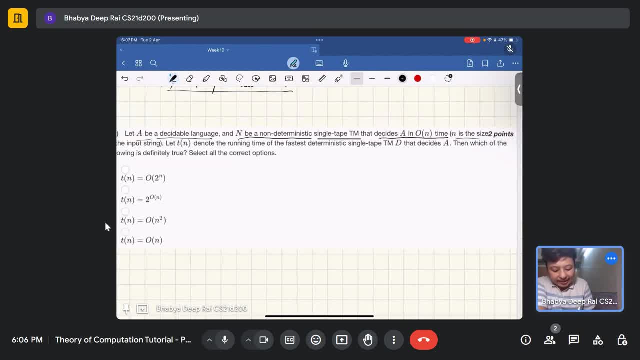 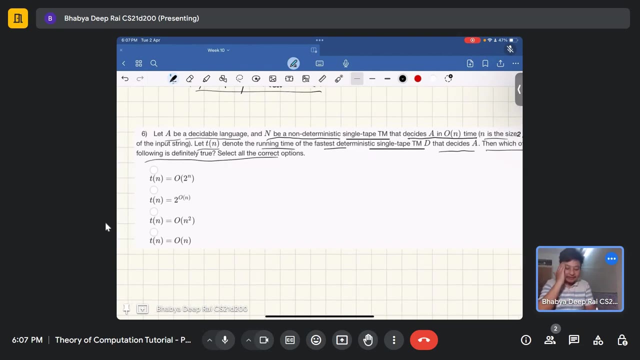 N is the size of the input. Now let Tn denote the running time of the fastest deterministic single tape Turing machine D that decides A. Then which of the following is definitely true? That is what it's saying. So firstly, let's break it down. 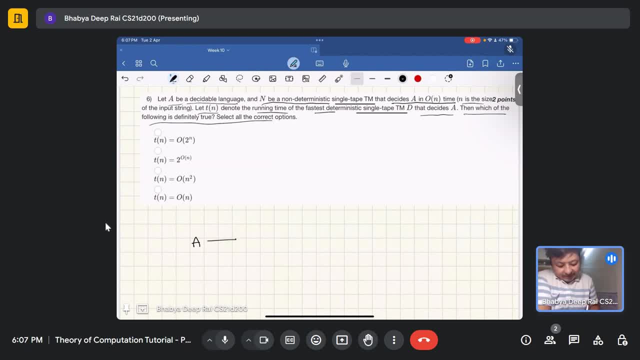 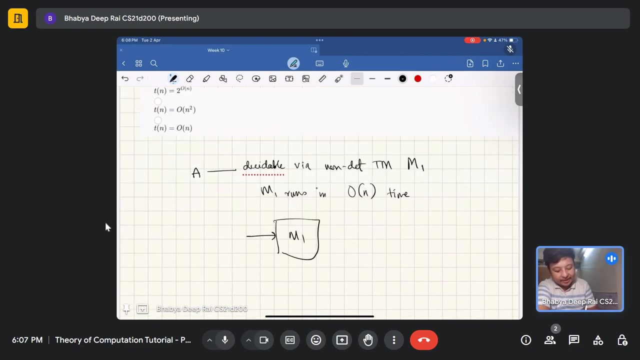 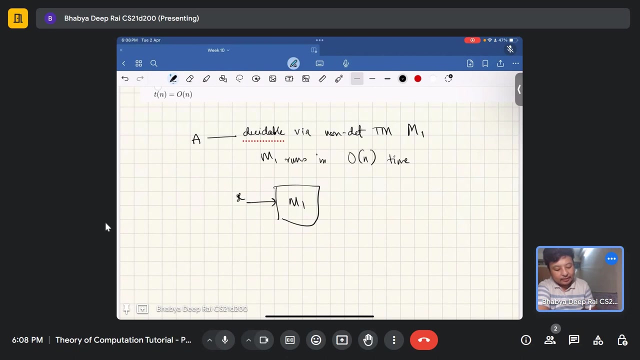 So A is a decidable language And A is decidable via a non deterministic Turing machine And let us call it M1.. M1 runs in order n time, linear time. This is some M1.. Takes an input x And M1 takes a run time equals order n. 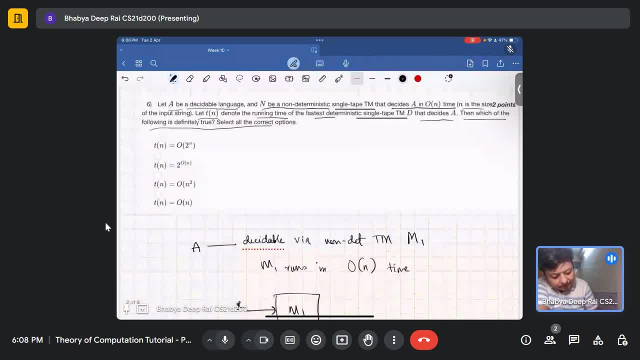 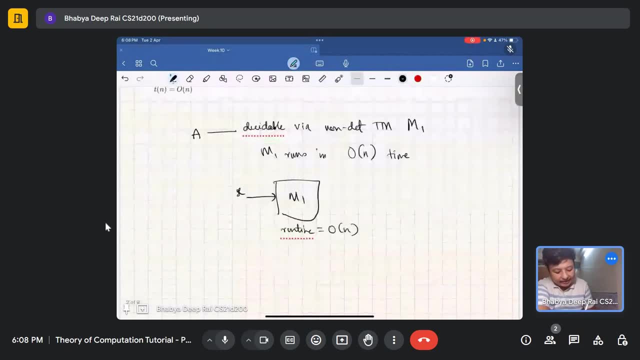 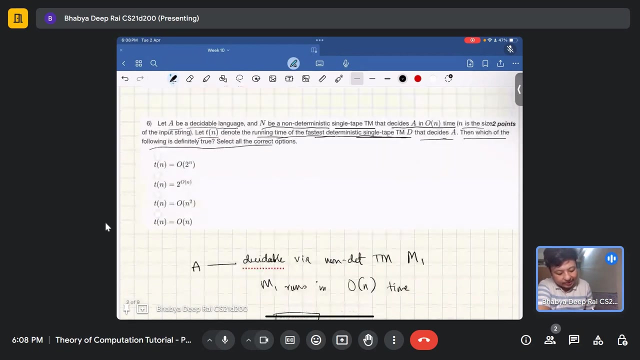 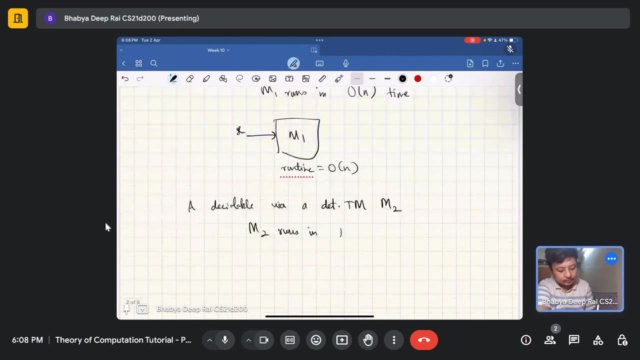 Next we are saying fastest deterministic single tape Turing machine that decides A. A is decidable. It's run by a deterministic Turing machine. Let me call it M2.. And how much time does it take? M2 runs in Tn time. 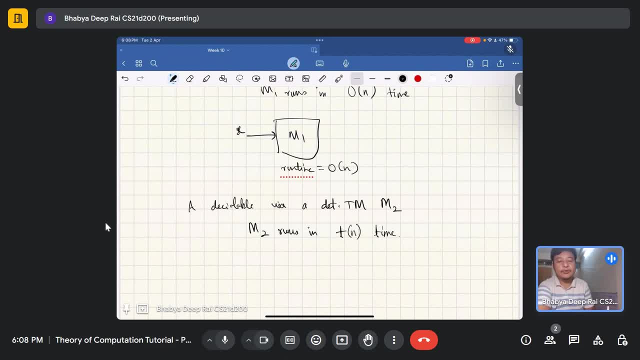 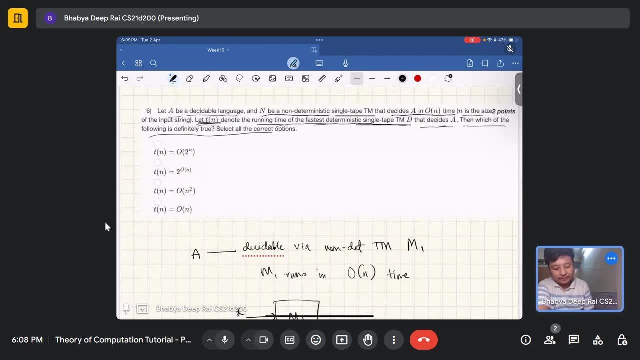 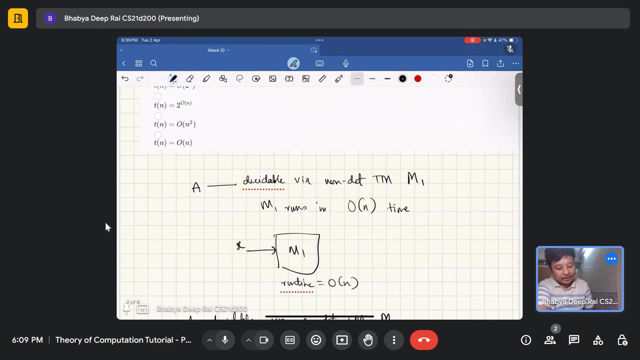 M2 runs in TnM. M2 runs in T of n time And it says which of the following are definitely: T of n is order of 2 to the n, T of n equals order 2 to the order n, and so on. 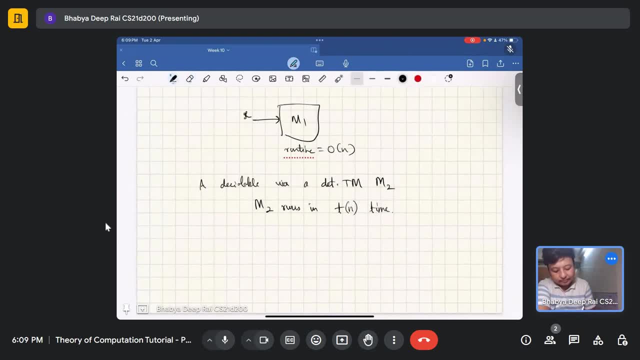 So what the idea is? given a non-deterministic Turing machine that decides A, I can give a deterministic Turing machine that decides A. I can give you an equivalent deterministic Turing machine. Okay, So given that what I mean is it decides the same language. 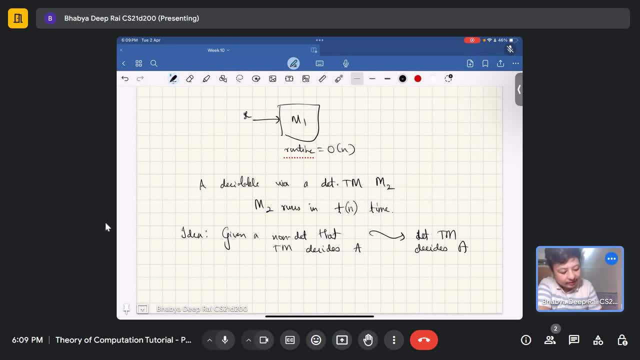 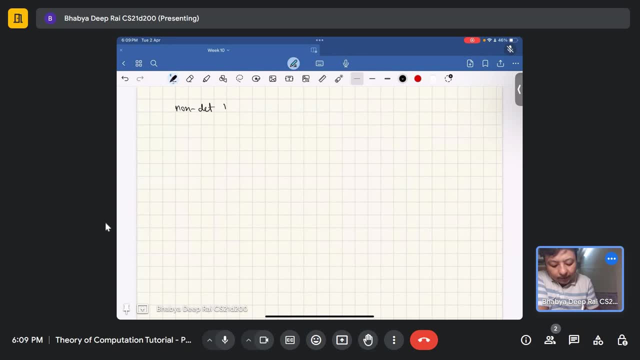 How does it do that? So how does a non-deterministic Turing machine function? That lies the process. So, non-deterministic Turing machine, it makes choices, which we call non-deterministic choices or guesses on the way. Okay, So suppose I say: 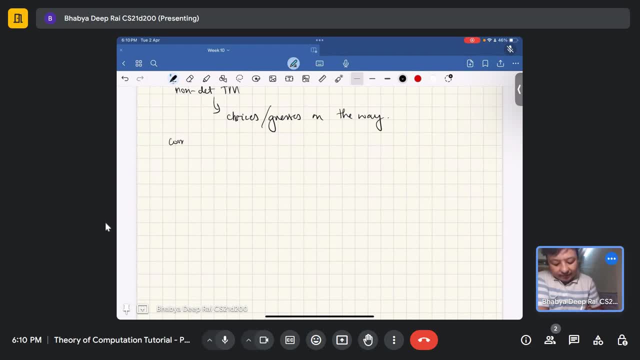 This is the working of M1,. okay, So M1 works as follows. So this is how I will represent it. okay, I am in a start configuration, So now my machine can move to various states. right, So I can move to various states. okay. 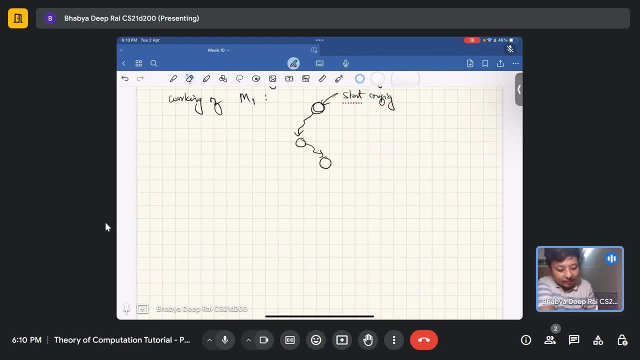 And what I can do is I move from this configuration to this configuration on the input. okay, So what does the configuration look like? The configuration talks about the state we are in. okay, The state, the head position: okay, And tape content. 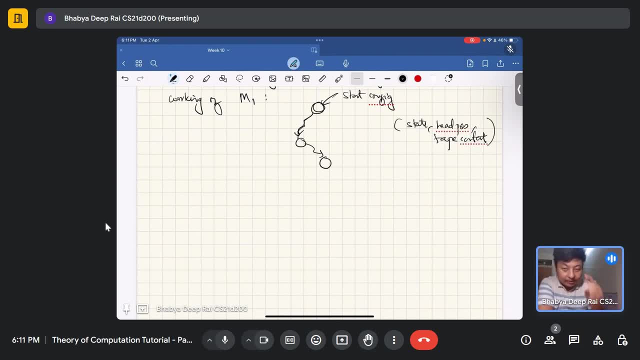 So my machine moves from one configuration to another configuration. But what? The typical thing about non-deterministic Turing machine is that it is a non-deterministic machine. So what does that mean? Non-deterministic Turing machine is it makes guesses on the way. 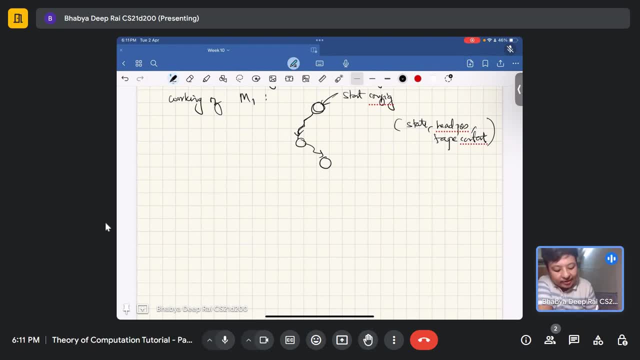 It tosses coins on the way, in other words: Okay, So it guesses, it makes a guess whether to move on. So if the coin toss caused a zero, then it will move to this, or the coin toss caused a one, I can move to this. 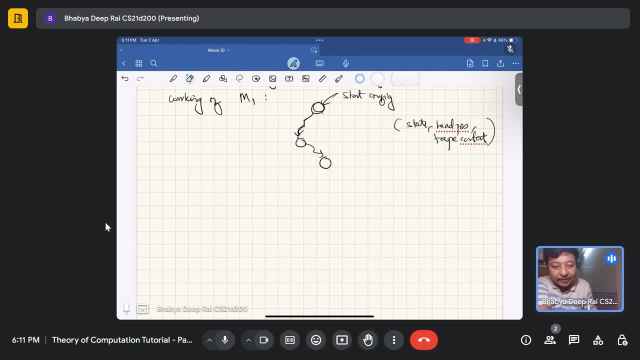 Something like this: Okay, It may not toss a coin, also that is fine, It may not make any guesses. and instead, here it may make a guess. So here, it may not make any guesses. So here it may make a guess, a guess. So in the first step it did not make a guess. Next step: it made a guess, So there. 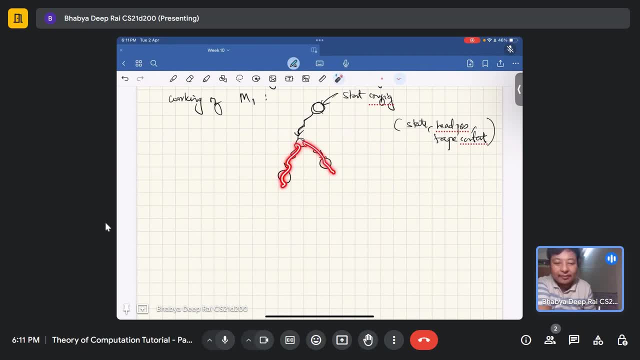 are two possibilities. It may explore the left branch or the right branch, And this is how it goes, and then it keeps making guesses on the way, and there are so many possibilities. Out of those possibilities, even if one of them is accept, leads to a final state one. 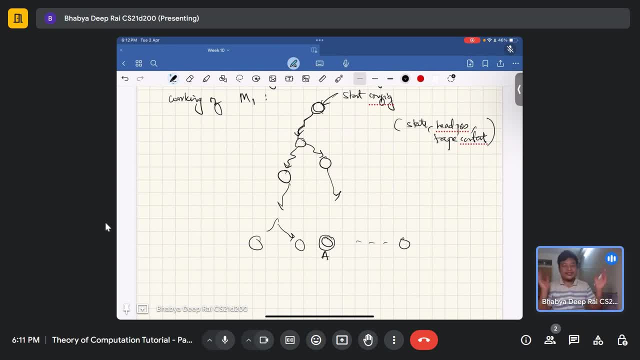 of them leads to a final state, then it is said that the entire machine actually accepts that input. That is what it means. Now, of course. what is the most amount of non-determinism that you can add? What is the biggest? what is the hardest kind of non-deterministic Turing? 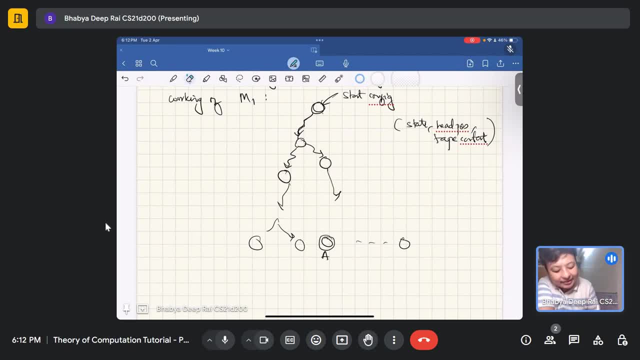 machine you can simulate is that. let's see the worst case. In the best case, what happens is- I don't have non-determinism at all, I mean, I don't make guesses on the way at all- So this is what it looks like. So this is what a deterministic machine looks like, And 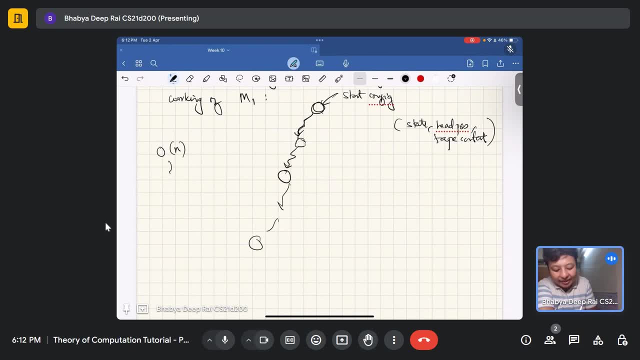 if I have a non-deterministic Turing machine and if I have a non-deterministic Turing machine that runs in order and time, then it means that I have a deterministic Turing machine also that runs in order and time because my non-deterministic machine is behaving in this. 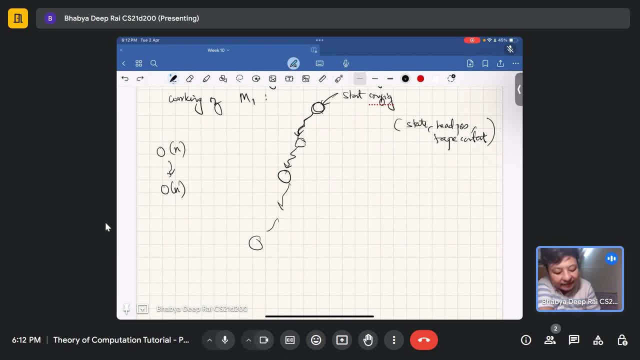 way. But this is not how it may always behave. My machine may not always behave this way in a very deterministic fashion. It may move in a highly non-deterministic fashion, by which I mean on every step of the Turing machine. The machine is making non-deterministic guesses, And next step, And next step, and so on. Right, 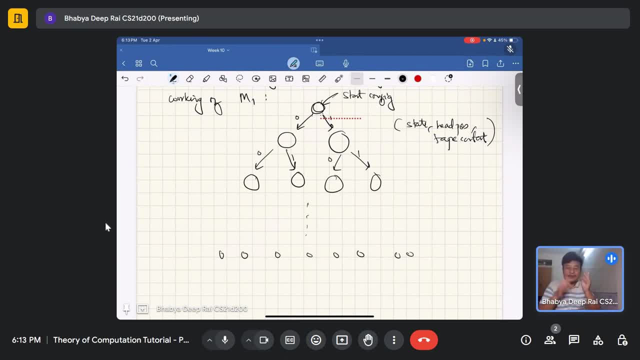 This is the worst case. in that sense, This is the most non-deterministic- loosely to call it. we'll call it the most non-deterministic way a machine can behave. Now. what happens Now? what we'll do is the running time of the machine. is how much The running time? 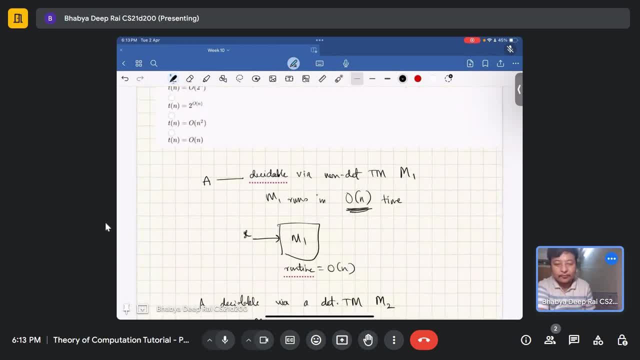 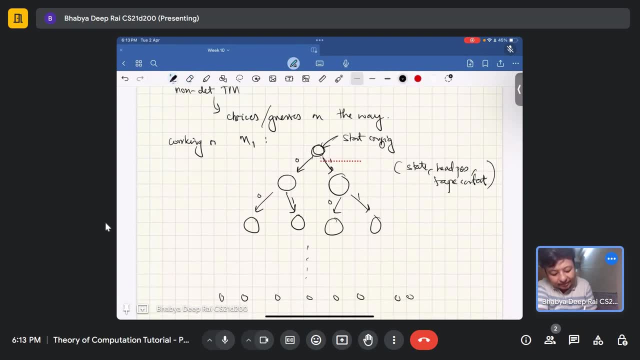 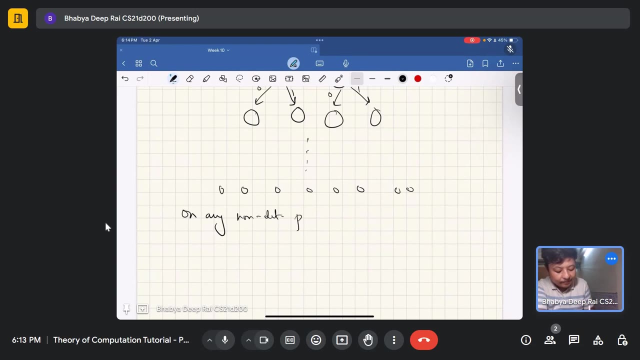 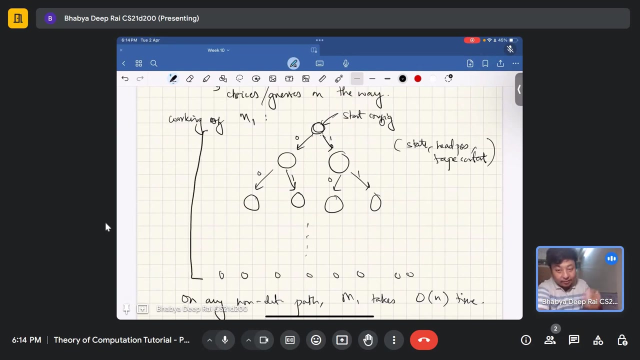 of this machine, M1, is order n. The running time of this machine is order n. So what does it mean? It means: on any non-deterministic path, M1 takes order n time. So on any non-deterministic path, this longest path from root to leaf. So my machine may. 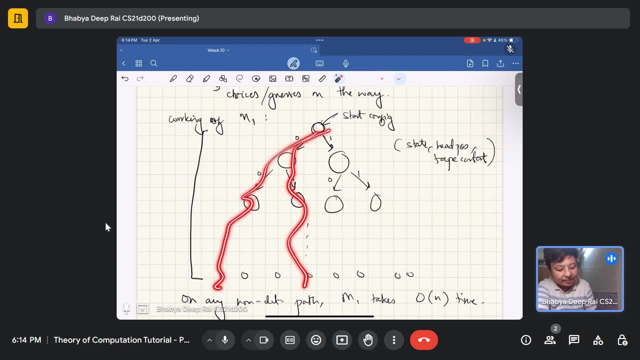 work like this. It may go from this way or it may take this way or this way, But what is the longest part possible? It is the running time of the machine, because exactly this arrow represents the steps of the Turing machine. Longest part of the machine will be, at most. 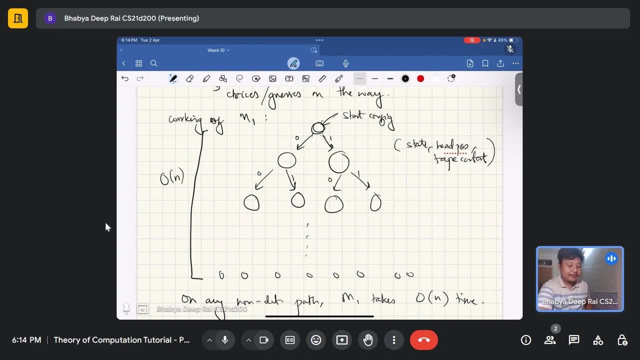 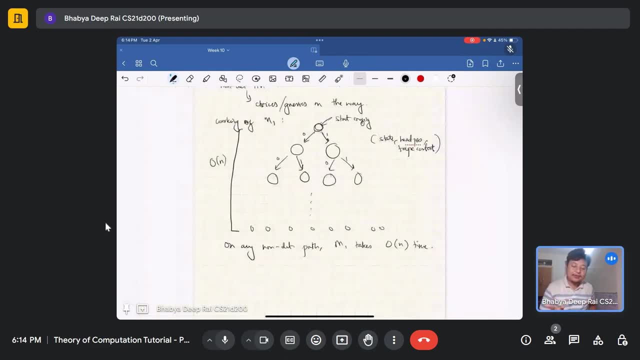 order n On any non-deterministic path. M1 takes order n time. Now, if we recall from the lectures, if I want to convert this non-deterministic Turing machine to a deterministic Turing machine, if I want to convert this non-deterministic machine to a deterministic Turing machine, 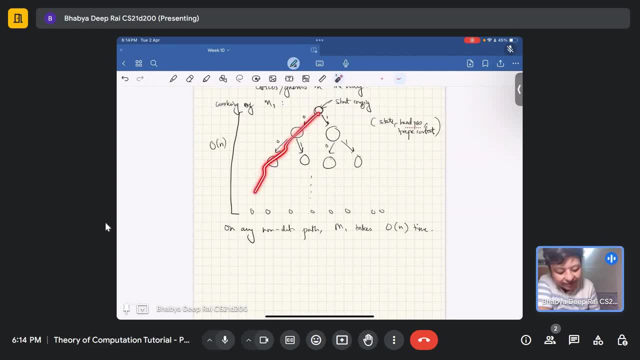 what do I do is I explore each branch. I explore each branch. I can either go in a depth for such manner, Or I can go in a breadth for such manner. Both are equivalent. But in total, how many paths do I need to explore? Here is one path. Here is another path. Here is another path. 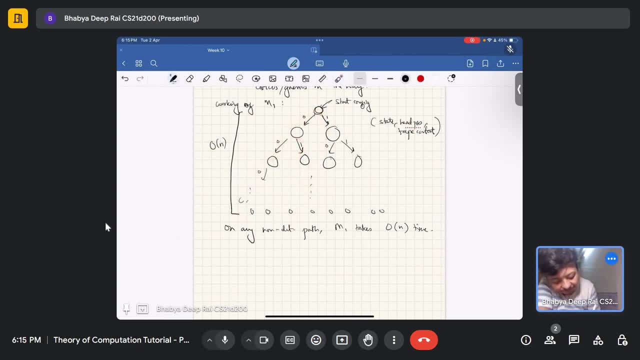 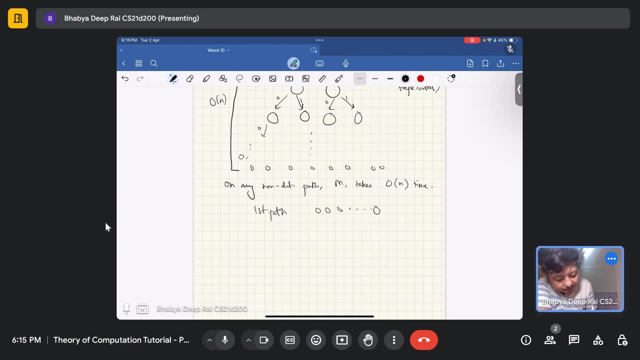 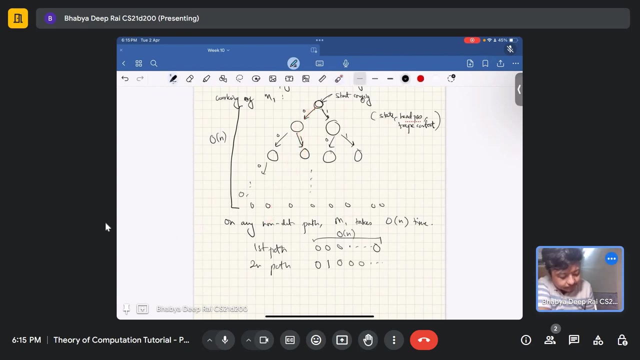 So this path corresponds to all zeros. This next path, first path, is like all zeros whose length is order n. Second path is: first I take order n. second path is: first I take a zero, then I take a one. First I take a zero, then I take a one, then I take all zeros. 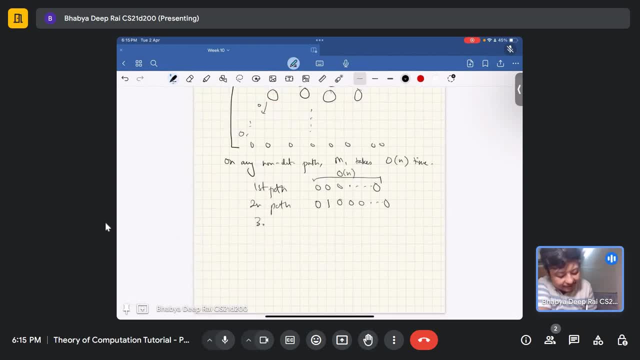 And similarly all so. third path: this is zero one, then I take a one, then zero, zero, zero. In other words, it's all possible. Order n: length: binary strings. Now, what does this mean? How many such strings are there? How many? Two to the order n by. 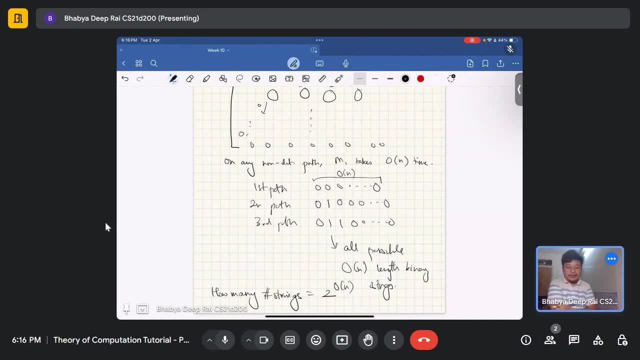 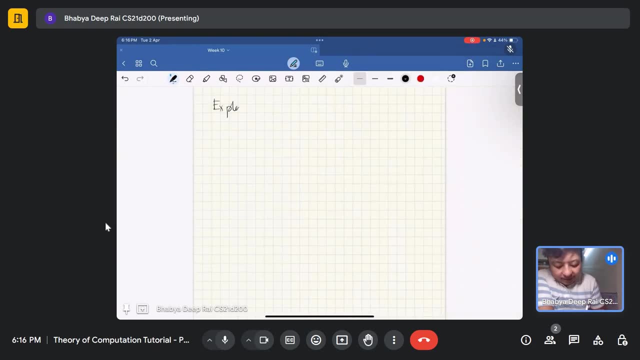 a simple combinatorial argument, Right? So what does this mean? What is the key takeaway Exploring? So my deterministic Turing machine would look like this. So here is my deterministic Turing machine deciding a For each y in zero. one power two to the order n. 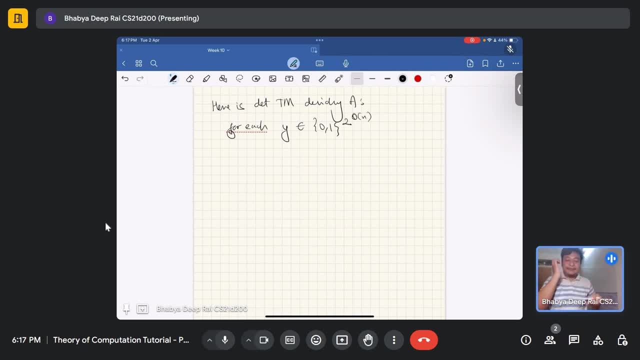 so I am going across each order n length binary string And simulate machine m one, that non-deterministic machine on path y, Yes, On path Y Y. So m one accepts, m one takes, then then accepts. 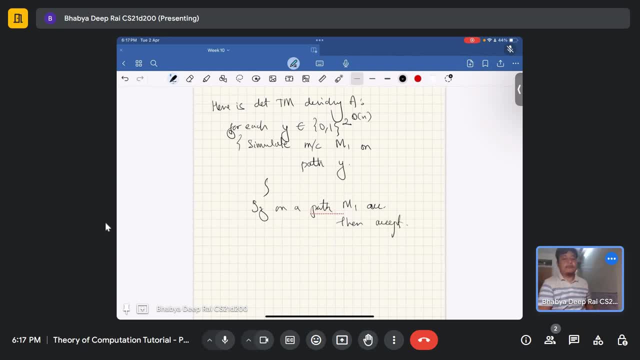 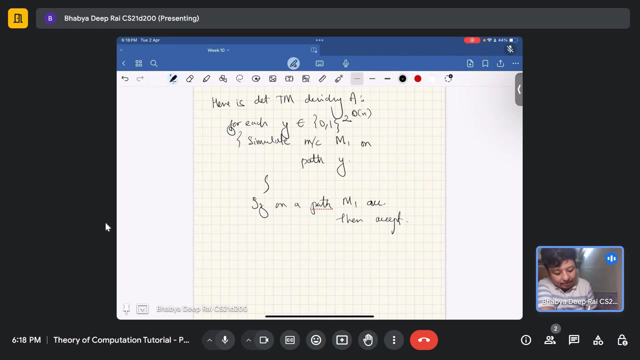 So what I'm just doing is I'm exploring all possible paths. If it accepts, then accept, And so taken by this machine. what is the time taken by this machine? so yeah, so for each of the two to the order n. I am taking some order n time for each of the. 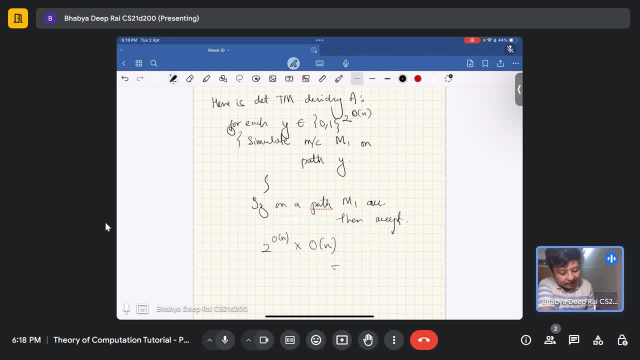 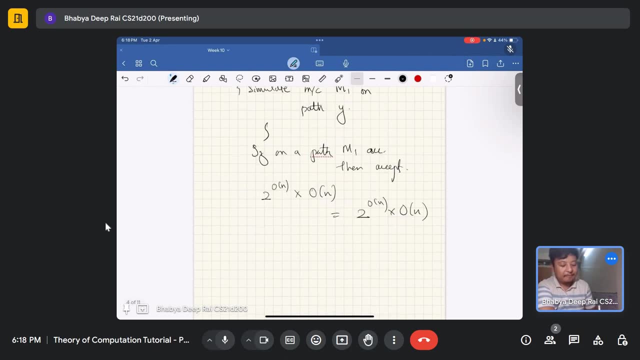 two to the order n paths. I'm taking some order n time, so it's 2 to the order n times, order n right now. because of order notation, we know that this is the dominant term here. right, and I can always give another 2 to the bigger I. 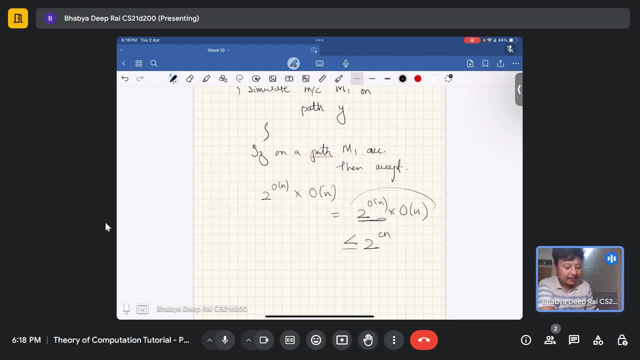 can always give 2 to the CN such that this is greater than 2 to the CN, is greater than this term. so this all times order n does not matter much. so this is again 2 to the order n. so what does this mean? if I have the fastest Turing machine and see, m2 is the? 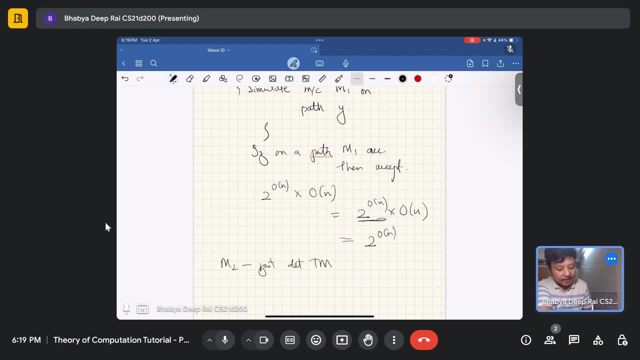 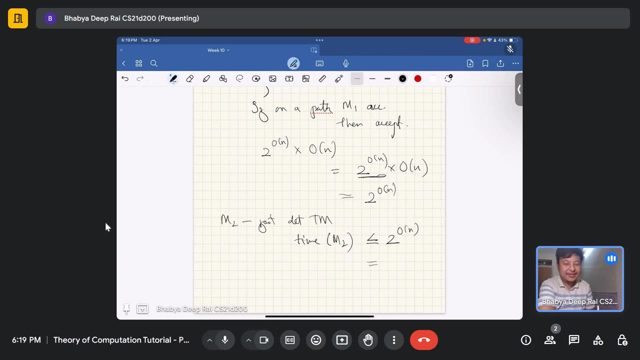 fastest deterministic Turing machine. this should always be less than time running. time of m2 should always be at most 2 to the order n. but since we are talking about order notation, we can change it with equal to, because equal order notation already means at most. okay. 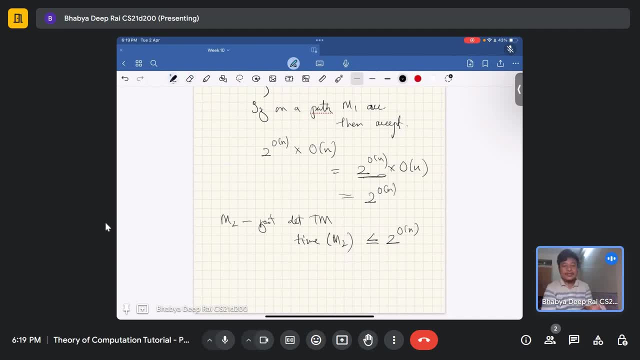 so, yeah, so running time of m2 is at most 2 to the order n. why? because if this was not the case, okay, and let's say running time of m2 was greater than 2 to the order n, running time of m2 was greater than 2 to the order. but then I said, okay, I gave you a. 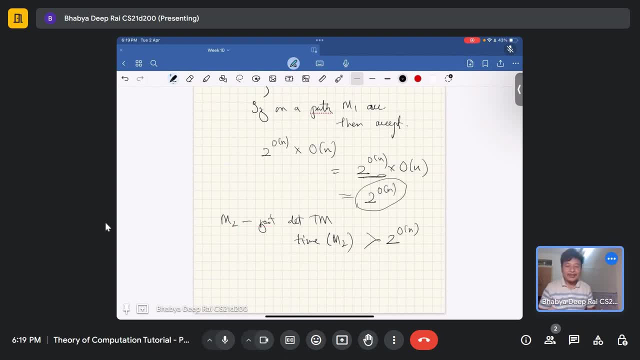 Turing machine that computes the same language, which takes only 2 to the order n time, and your fastest, your supposedly faster Turing machine takes more than 2 to the order n time. but how can it be faster that way? how can it be the faster Turing machine? wait, oh sorry, I don't think i can undo. 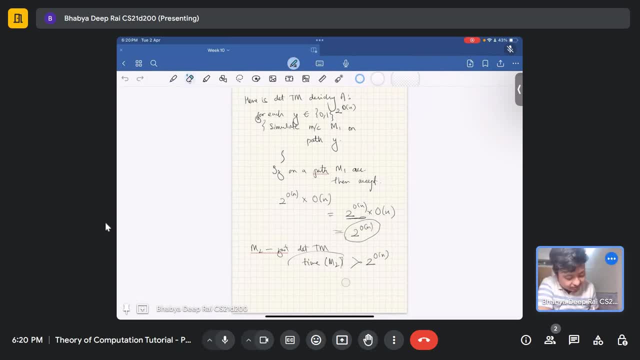 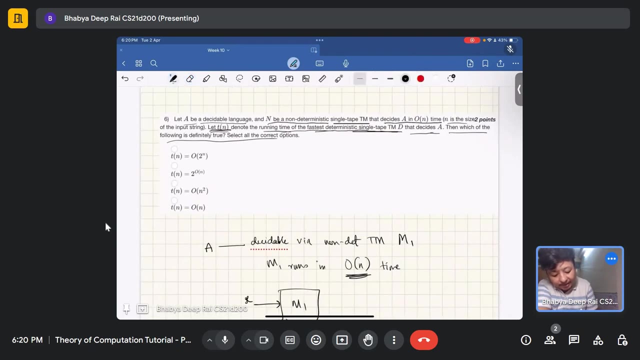 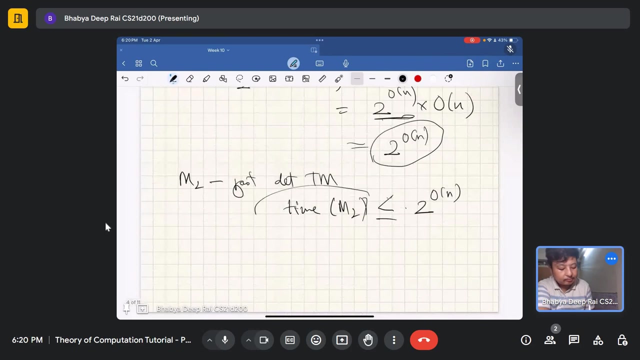 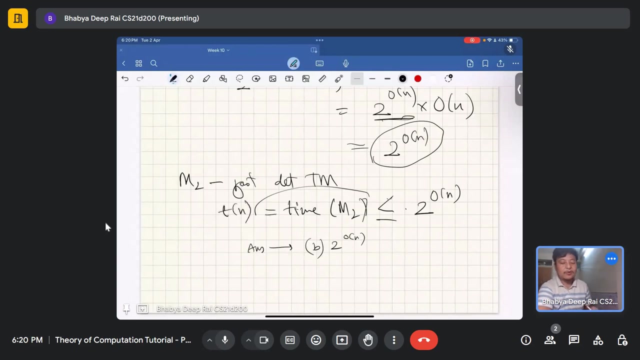 now. so what I'll do is: yeah, anyway, this this holds. Therefore, yeah, therefore answer. what is the answer? so, Tn takes order 2n. Tn takes 2 to the order nTx, so on, so and so, but the is 2 to the order n. Answer is b. tn takes order n. This time is nothing but t according. 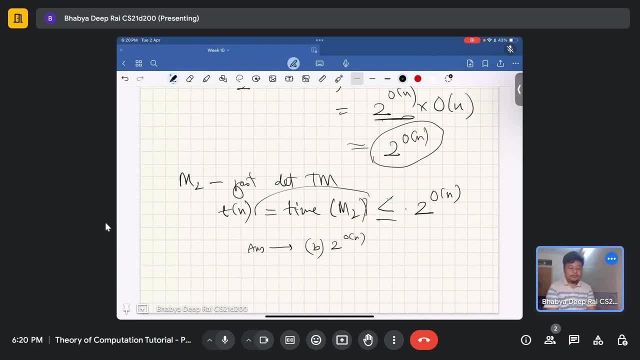 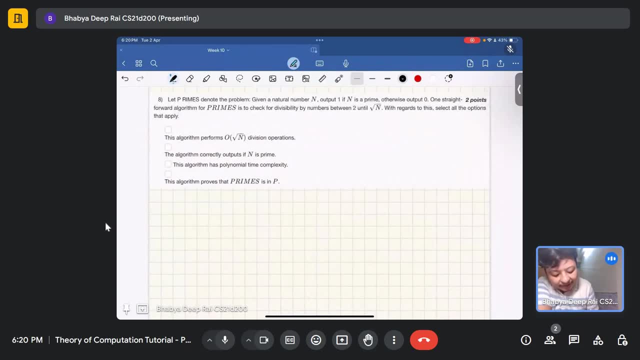 to the question. Okay, good, So let's look at the next question. Question says: let primes denote the problem. given a natural number, n output 1 if n is prime, otherwise output 0.. One straightforward algorithm for primes is to check for divisibility by numbers between: 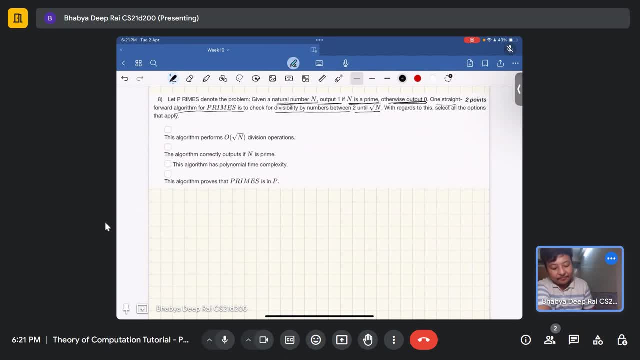 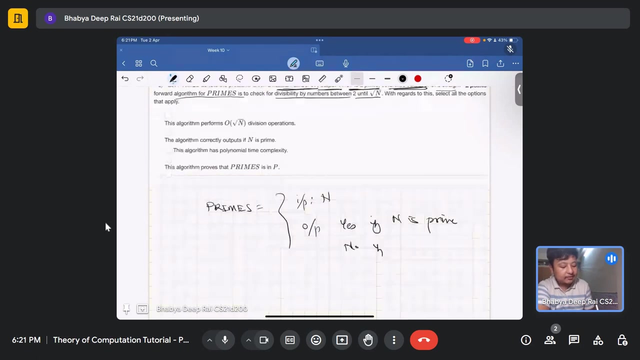 2 until root n. With regard to this, select, all that apply. So what it says is so primes: okay, so primes is given a natural number: n output: yes If n is prime. no if n is not. it's not prime Output: yes if n is prime. no if n is. 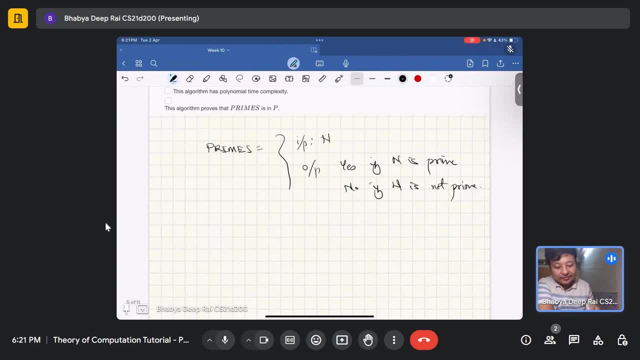 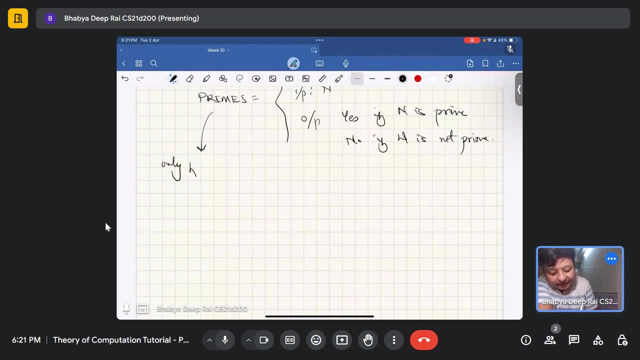 not prime. So what is the high school method of doing it? So what is prime? Prime is only factors. are 1 and n? If n is prime, 1 and n will divide a prime, divide a prime. Okay, So one algorithm is: 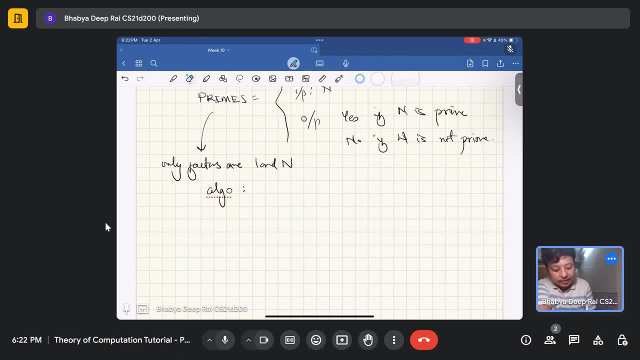 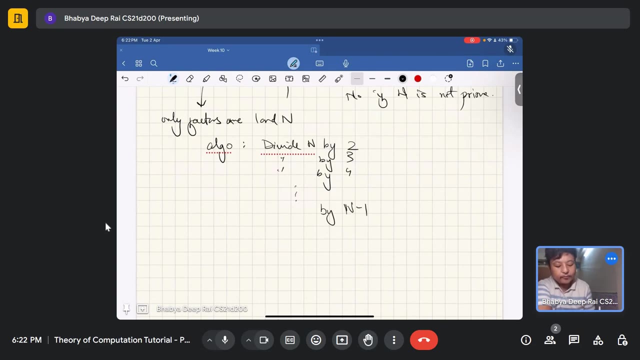 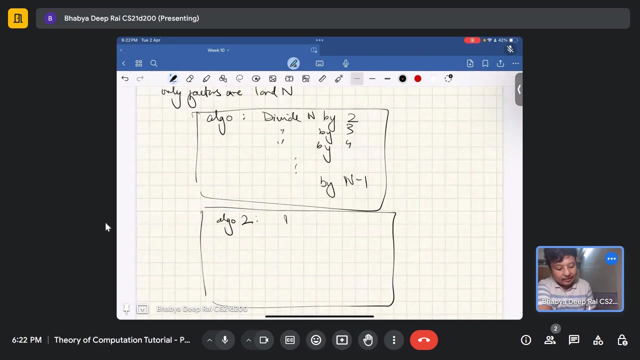 one possible algorithm is divide n by 2, then by 3, by 4, and so on till by n minus 1.. Okay, this is one algorithm. another algorithm. okay, another algorithm, slightly clever algorithm, is divide n by 2, by 3, by 4, and so on until by root n, and then stop. 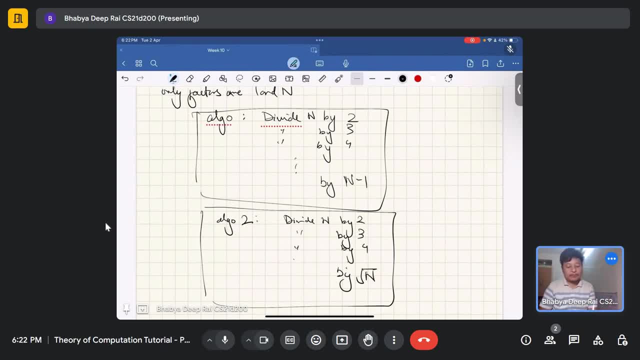 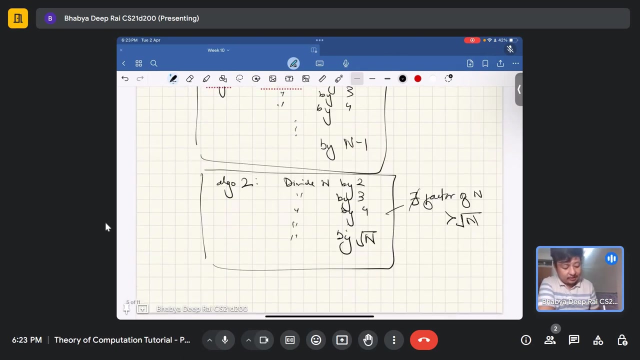 why? because there cannot exist a factor of n which is greater than root n. there cannot exist a factor of n which is greater than root n. why? because uh, if there exists a, because root n itself times root n is equal to uh n. right and uh, if i increase this root n. 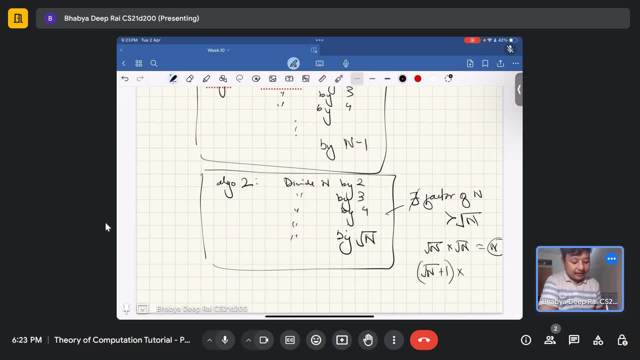 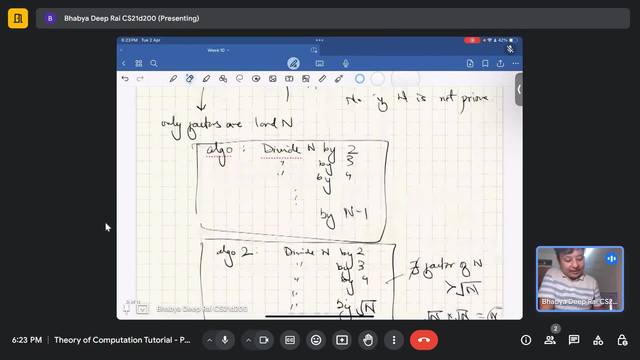 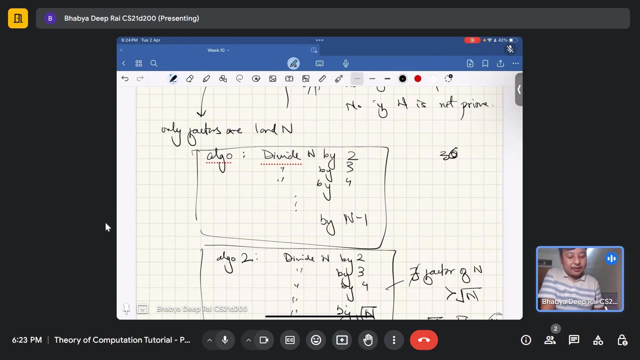 plus one times something, then i cannot get anything else because this needs to be very small. whatever is here needs to be very small. uh, it needs to be something smaller than root n, but this is not possible now the uh. so like, for example: um, if i want to check whether 36 is a prime or not, i need only to check until uh six. okay, 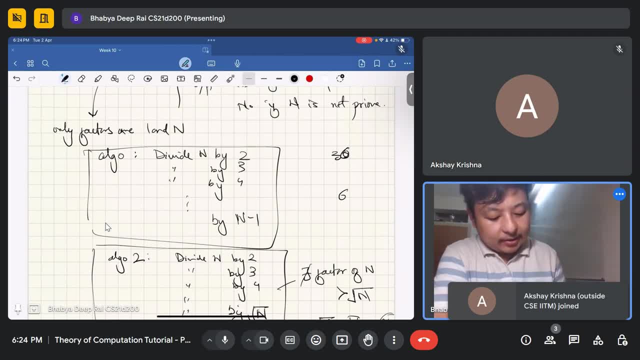 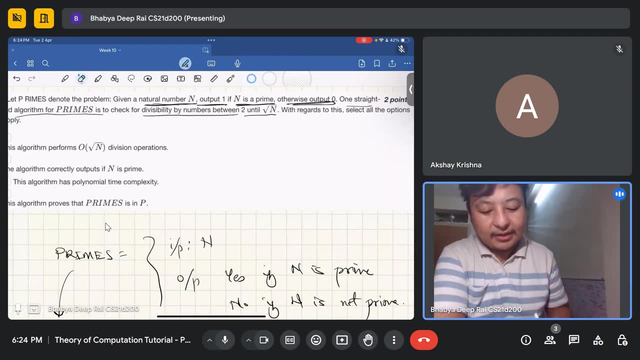 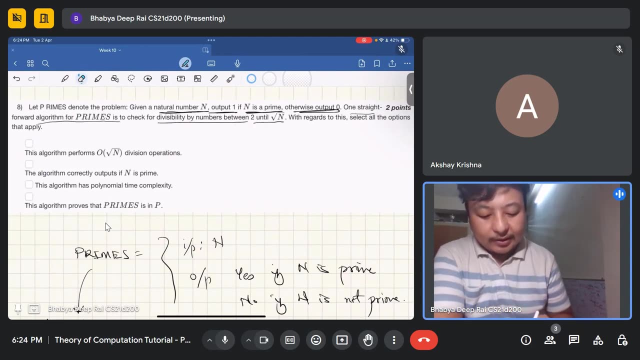 right, oh, hi, okay, so uh, yeah, i'm doing this question okay, from the past assignment, uh, which talks about times. okay, so, uh, the question is: given a natural number, okay, output one if n is prime, otherwise output zero. one straightforward algorithm for primes is to check divisibility by numbers. 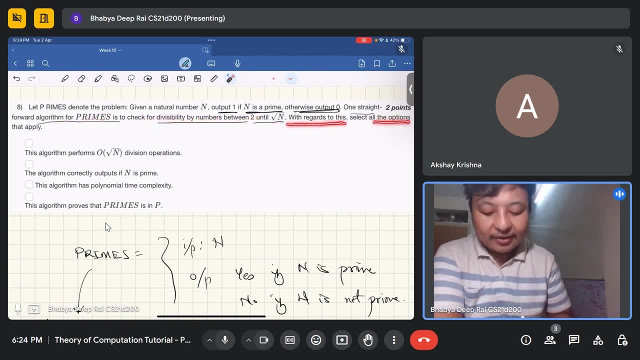 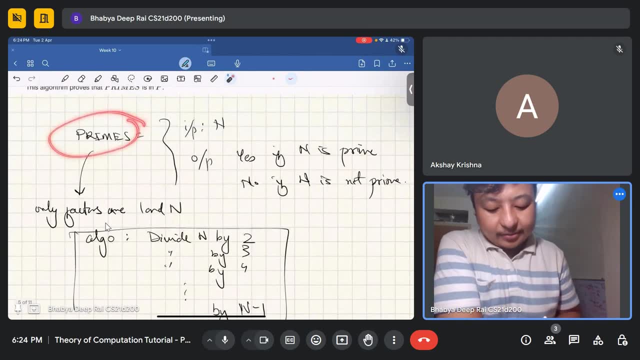 between 2 until root n. with regards to this, select all the options that apply. okay, now, uh, primes, uh, what is the language? primes: if the input is n, then the output is yes if n is prime. or in the question it says one and output is one if it is prime and output is zero if n is not. okay. 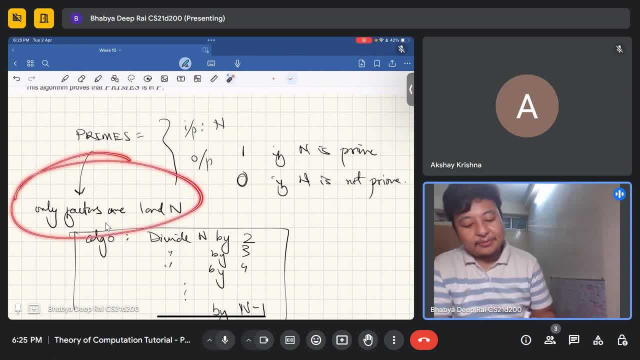 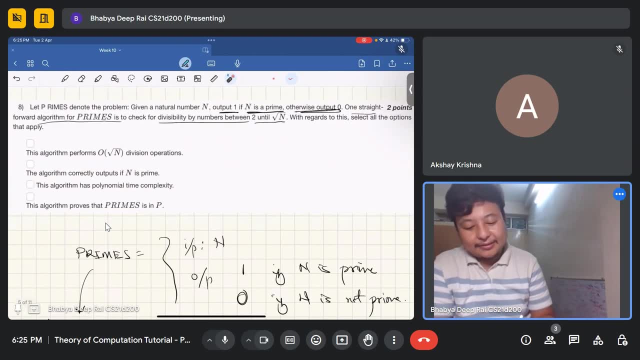 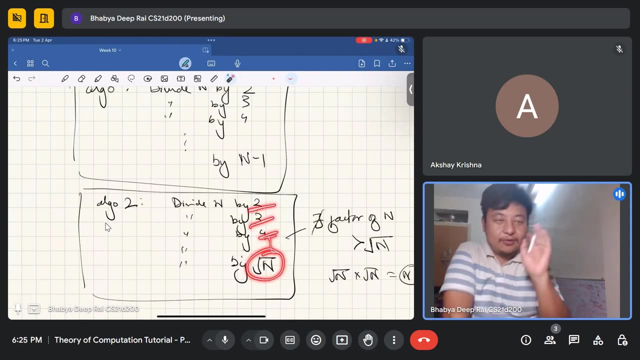 now, what is the prime number? a prime number is a number whose only factors are one and n. okay, now what the question is saying is this: uh question is saying: what you do is you divide by 2, 2, you divide by 3, you divide by 4 until root n? so this is a normal high school method to do it. okay, 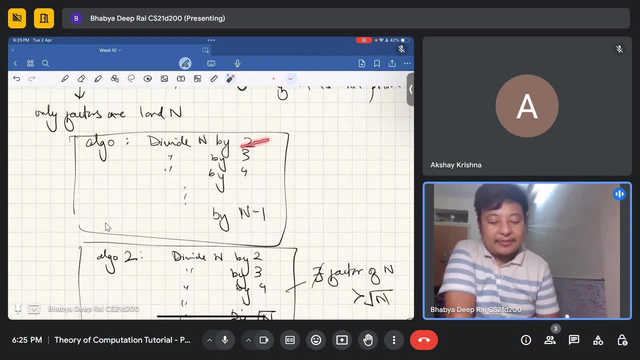 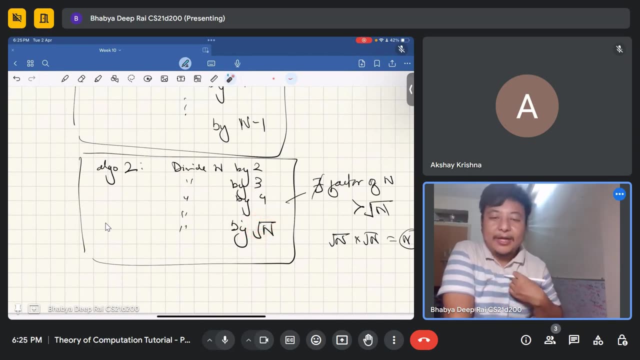 a simpler algorithm obviously is: you know, divide by 2, 3, 4, 5, 6, 7 until n minus 1, and if none of them divide the number, then the number is prime. but we can make the number, we can make the algorithm slightly, slightly more efficient by only going until root n okay, it takes only root n time. 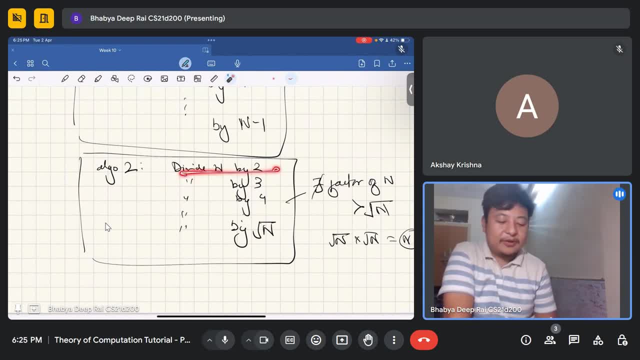 how you go till you divide by 2, 3, 4 and so on, until you go till root n. and if root n also does not divide, then any other number after it will be a factor of one of these. so if none of these numbers actually divided that number, divided number n, then obviously these multiples of 2. 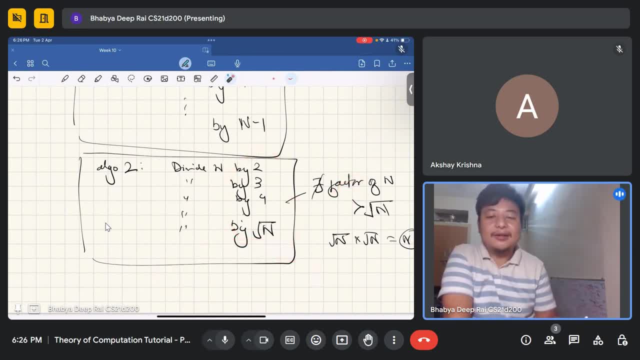 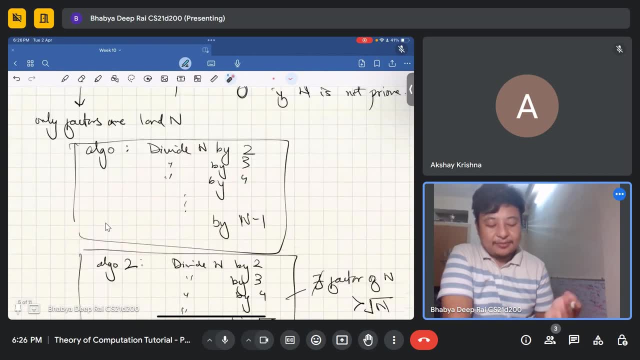 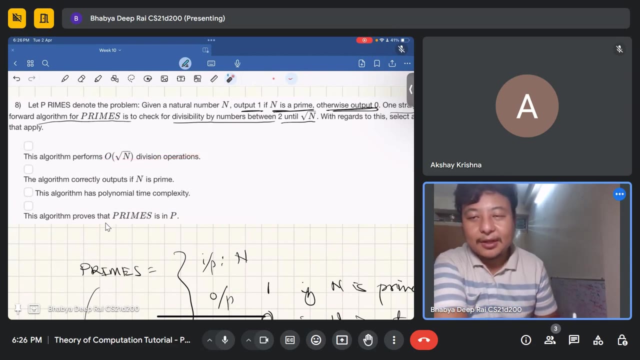 3, 4 until root n will also not divide the number n, right? so that is the idea. so, uh, you, you go only till root n, and so this algorithm looks good, right? so the question? the question says the algorithm performs order root n many division operation. this is true, we divide order. 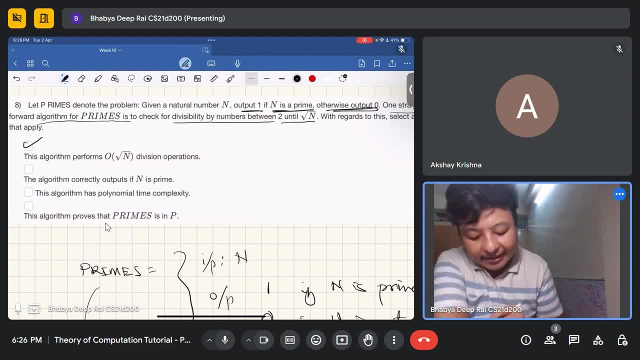 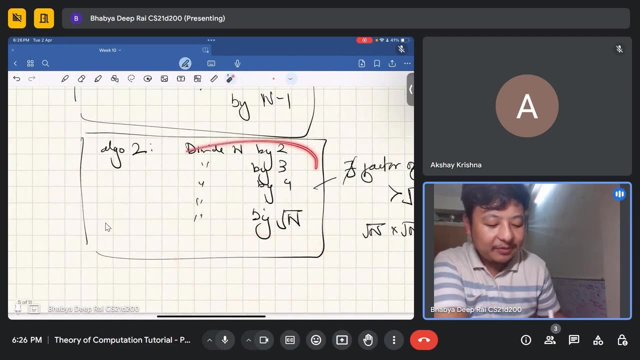 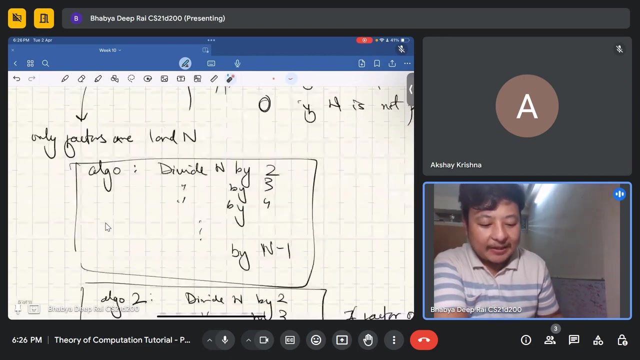 n order, root n. many times we are only going till root n. right, the algorithm correctly outputs if n is prime. this is also true. so, because we just saw that any number that is after root n is a multiple of these or some combination of these. okay, so, uh, yeah, so so going until. 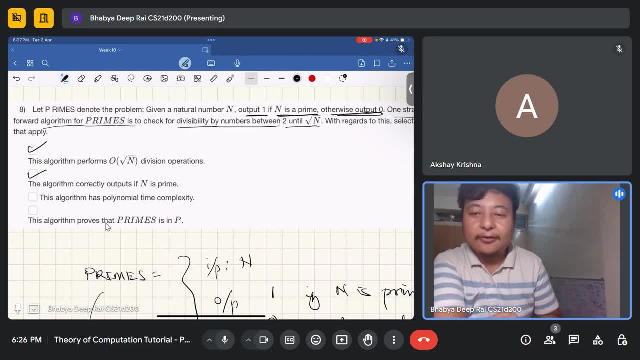 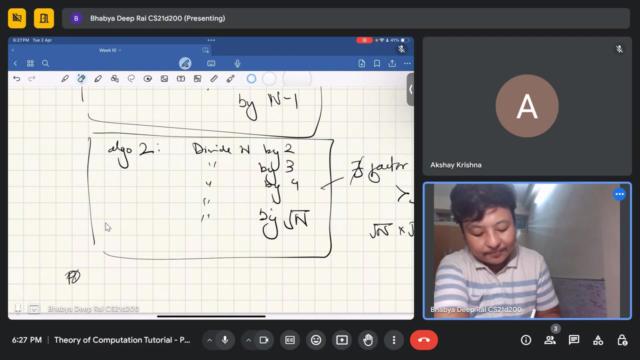 root n is fine, we are happy with it. so the algorithm correctly outputs if n is prime. uh, now this algorithm has polynomial time complexity. now here is the tricky part part. The problem here is actually as follows: The problem or the catch, it looks like it. 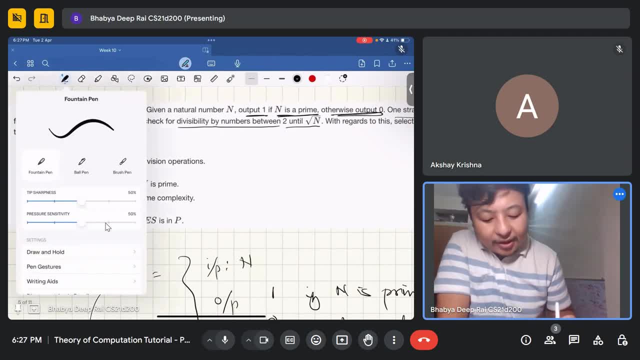 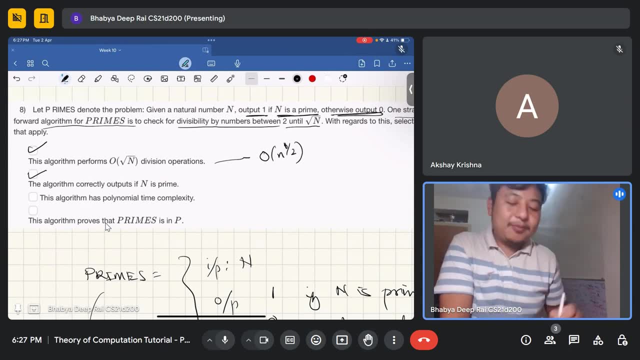 takes polynomial time. It takes only order root n time. So what is order root n? Order root n divisions, right Order root n divisions, which is order n to the half. So this is still polynomial. Actually, this is actually slightly better than polynomial in some sense. It takes 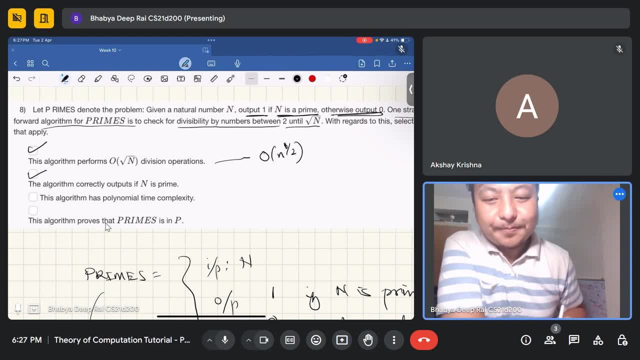 only some sublinear exponent, n to the half, And this looks like it takes polynomial time, But actually it's not taking n to the half, It's taking n to the half, capital n to the half. What does this mean? I'll tell you This. n is given as input. 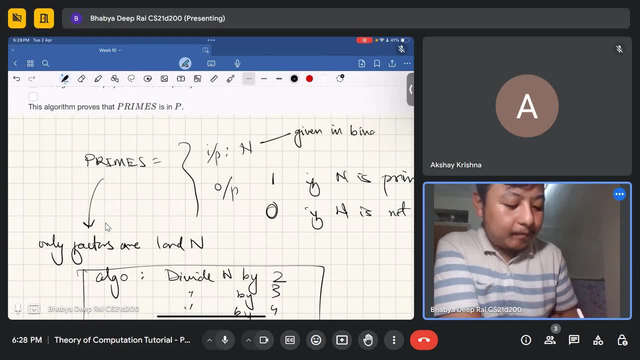 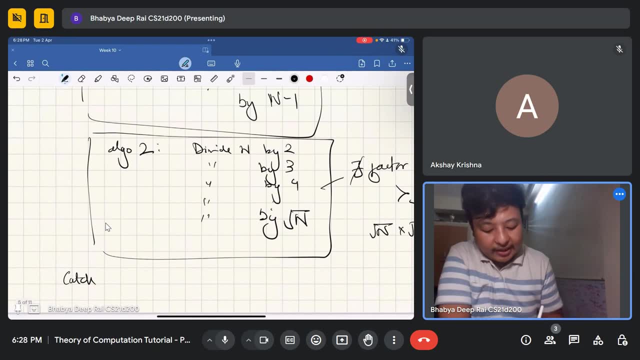 In binary. So what does it mean? Catch is n is given in binary. So what does it mean? Number of bits to represent n is log of n. Okay, Number of bits to represent n is actually log of n many bits. So input length that: 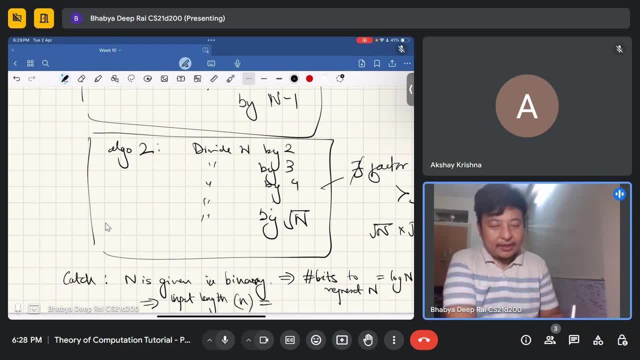 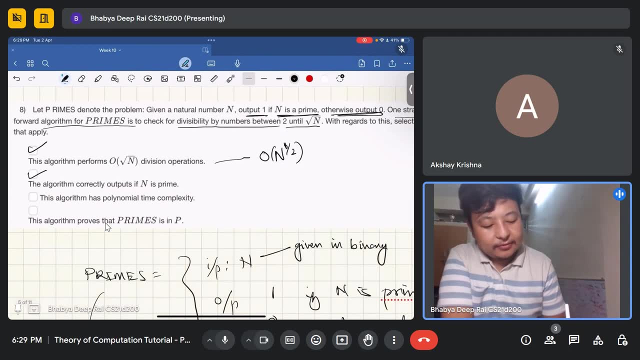 is n. okay, is actually log of n. Getting it So and n, like I said, n n is actually log of n. So by property of log you have that capital. n is nothing but 2 to the n. So what does this mean? This is equal to order of 2 to. 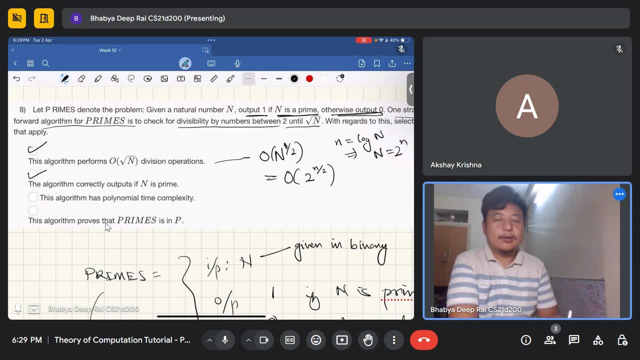 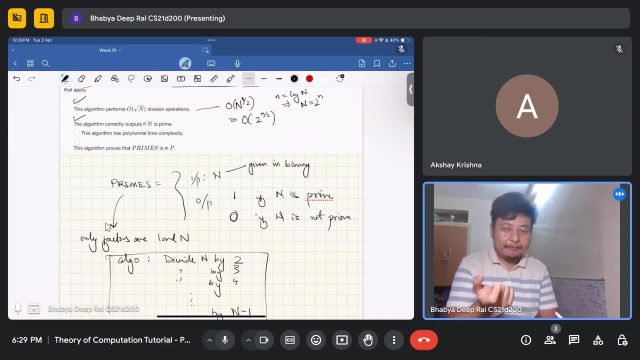 the n by 2. Getting it. So this is the catch. actually, The input given to us is given as binary. The number n, capital n, is represented in binary. If it is represented in binary, what is the length of the input? Log of capital n. If the length of the input is log of capital. 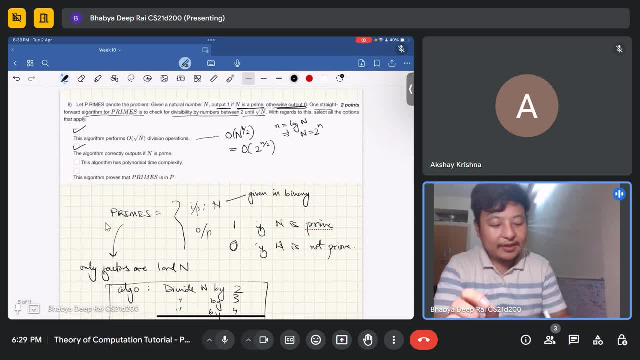 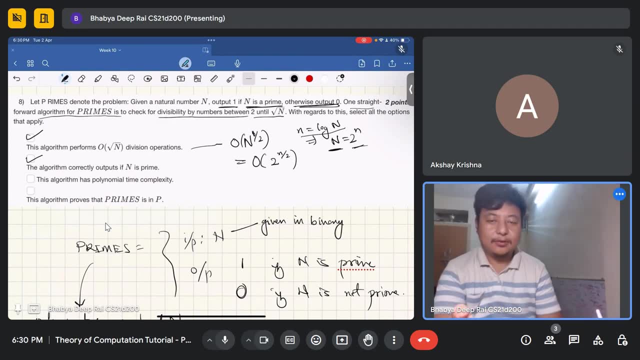 n, okay. length of the input is log of capital n. So what is capital n actually? 2 to the n, Okay, And the number, the amount of? sorry, the algorithm performs order root n, many division operations, right. Order root n is nothing but. order n to the half, There's nothing but. 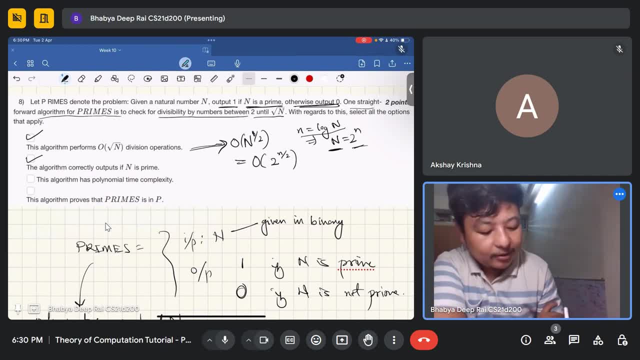 order n to the half. But what is capital n? It's 2 to the n. So we have order 2 to the n, 2 to the n by 2.. What is this? This is exponent in n, Which is the input length, Which is the actual input length, Because people may, this is a. 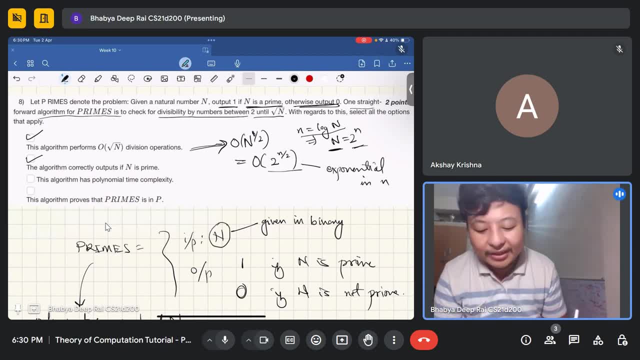 good exercise because people may mistake capital n to be the actual input length, But actually the input length is small n Getting it. So this algorithm has polynomial time complexity. that is clearly false. This algorithm proves that prime is in p is also false Because 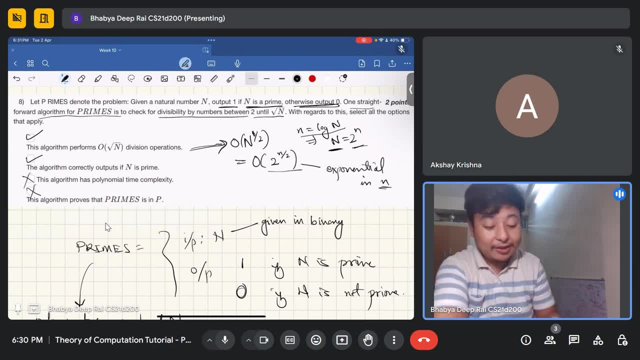 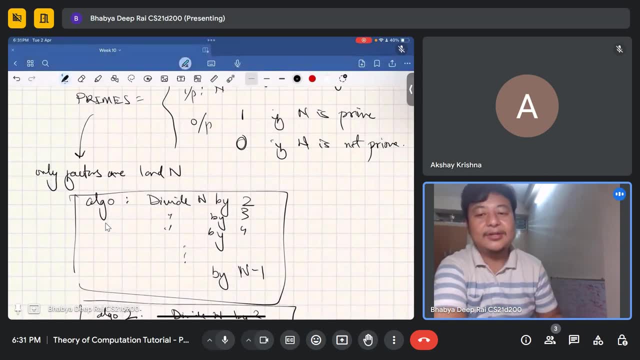 this algorithm is actually an exponential time algorithm which looks like a polynomial time algorithm. this high school method Looks like a polynomial time method, time algorithm, but actually it's an exponential time. So yeah, So did you get it. Akshay, I'm audible, right. 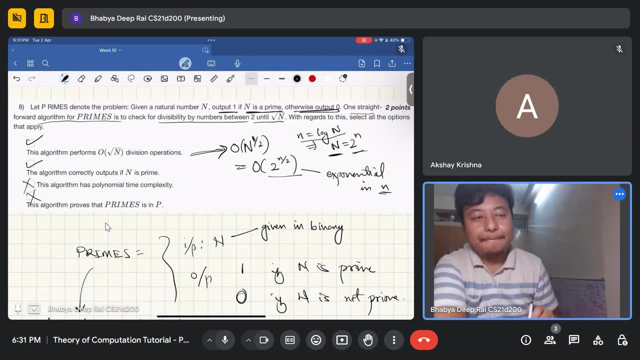 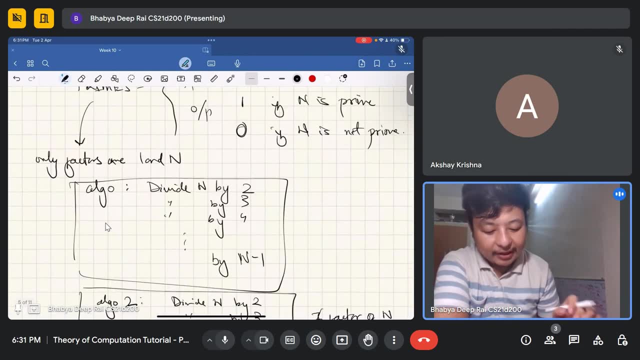 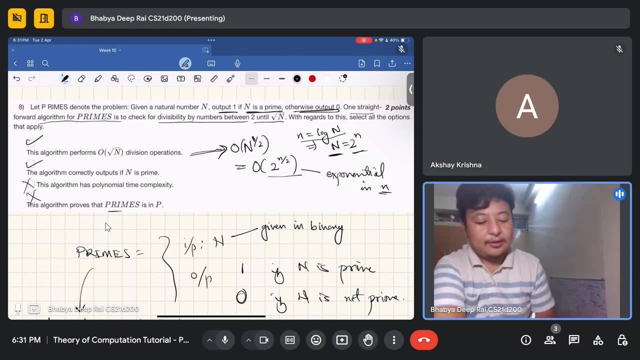 Yes, sir, Okay, So this is fine, right. Yes, sir, Okay. So yeah, A quick more addition to it. Actually, this in the field of complexity theory: primes. It was not clear whether primes is in p or not. People were not sure. People thought 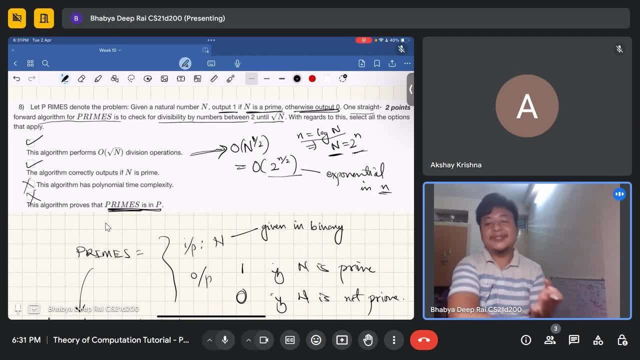 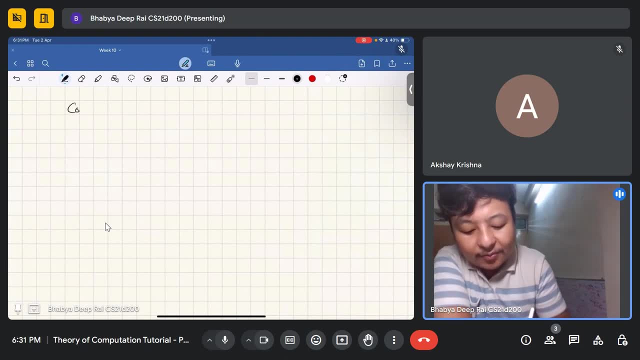 that primes is somewhere between p and np. Some people thought that primes is also in np, But actually and composite, if you try composite- is in np. That has a nice np characterization And primes is in p or not. This was an open question. 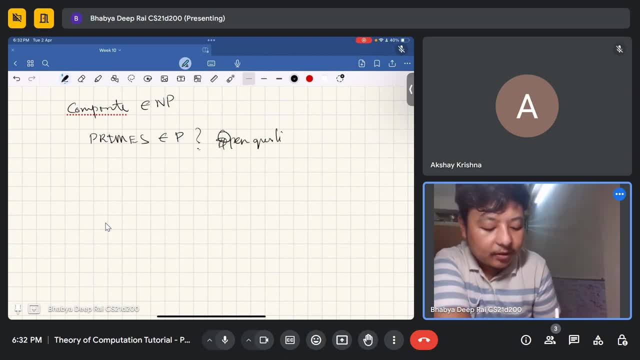 This flew inside and …. Yes, Open question until 2006.. And in 2006, this is the famous result called the AKS result. AKS: Primality And a stands for Agarwal. Kayal Saxena, Nitin Saxena. 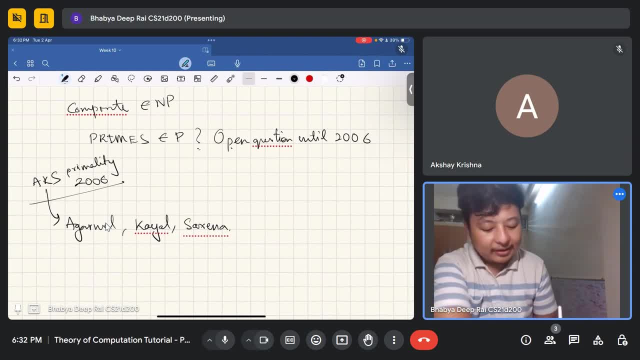 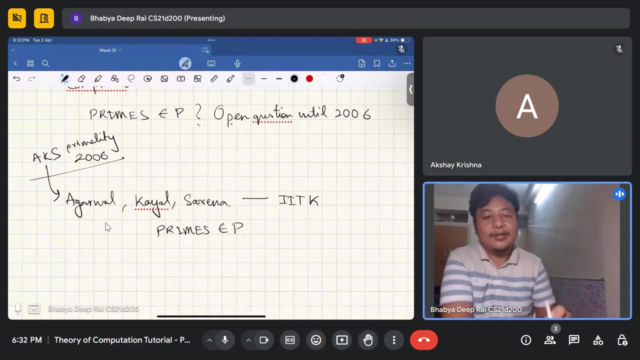 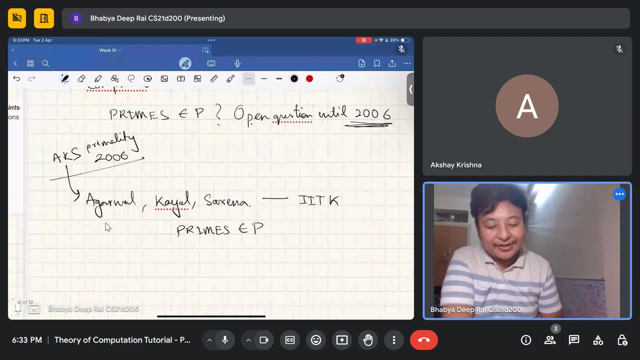 Sena Kayal and Manindra Agarwal and from IIT Kanpur actually came up with this result that ES primes SNP. So this was a huge result and this is only resolved in 2006.. So what? the main thing is that this particular high school method actually kind of gives us the 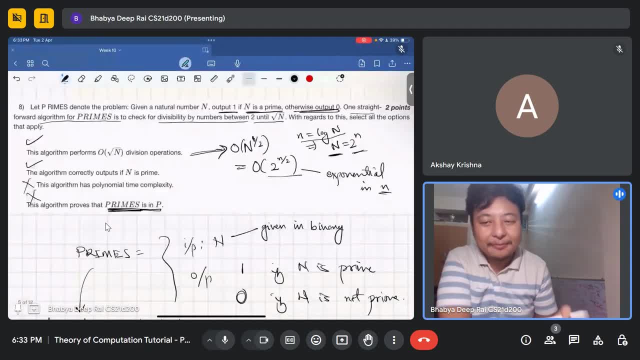 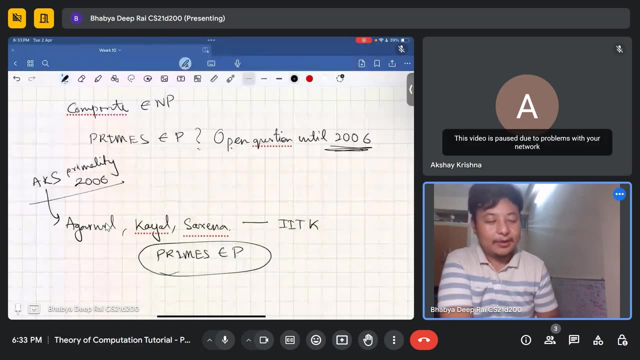 misconception that primes is already in P. It can be solved in polynomial time, but actually it is not the case. It took a lot of development in mathematics and computer science to finally declare that primes is in P and I think this won the Godel Prize in 2006 also. this result. 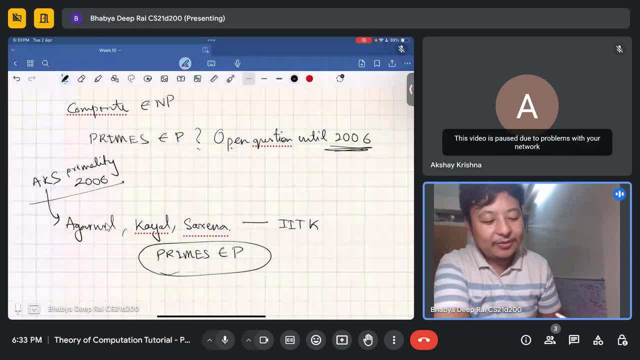 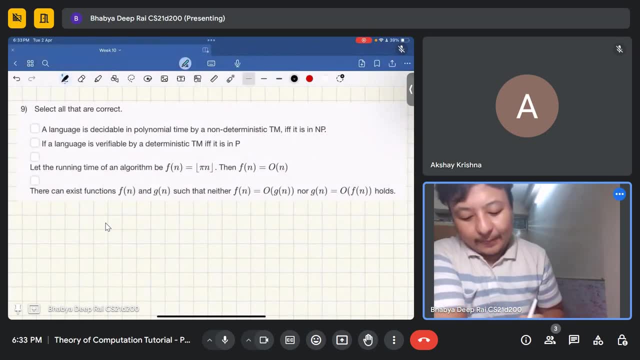 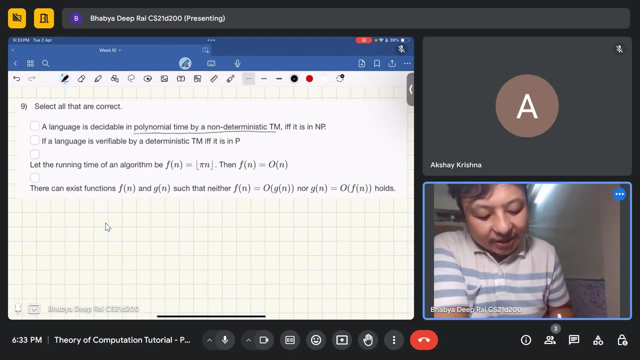 Anyway, just a quick addition. Now we will move on. So here is another question. from assignment Select- all that are correct- A language is decidable in polynomial time by a non-deterministic machine if, and only if, it is NP and if a language 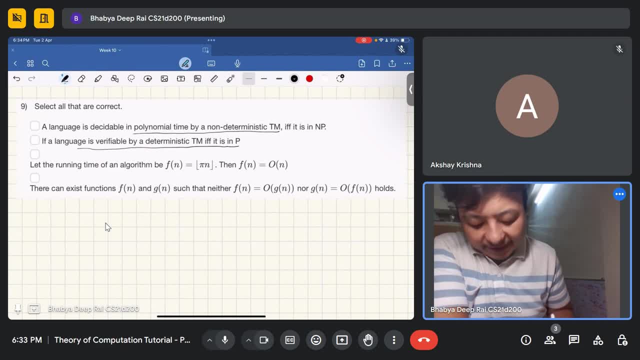 is verifiable by a deterministic Turing machine if, and only if, it is P and so on. Let's tackle them one by one. A language is decidable in polynomial time by a non-deterministic Turing machine if, and only if, it is NP. 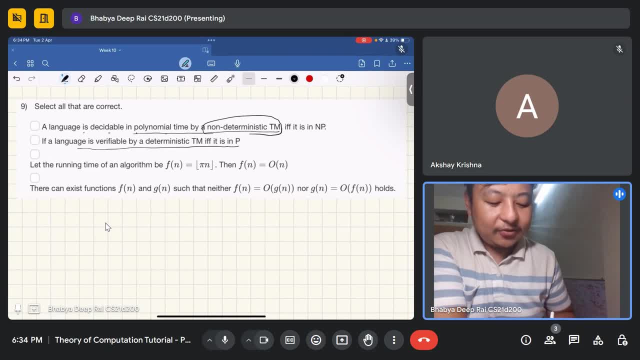 Yes, because we are talking about non-deterministic Turing machine. This is exactly the definition of the NP class. This is correct If a language is verifiable by a deterministic Turing machine, if, and only if, it is NP First of all. Yes, 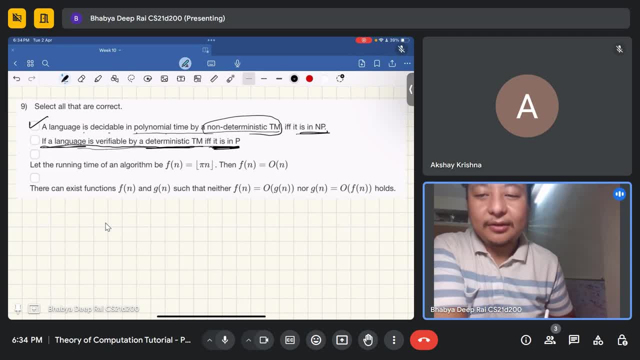 Yes, Verifiable by a deterministic Turing machine. This does not make sense. Deterministic Turing machine taking how much time? Deterministic Turing machine taking exponential time or polynomial time or so on. It does not say If the answer was polynomial. let's say this: 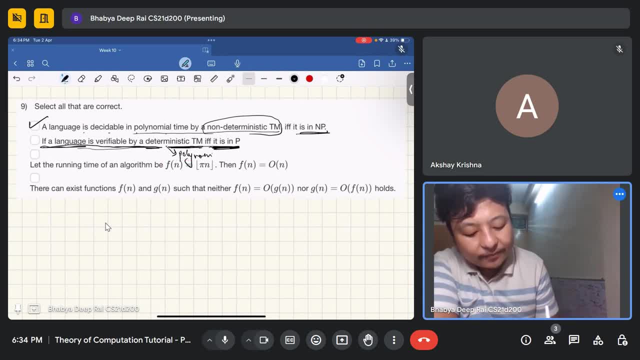 was polynomial, This said, polynomial verifiable by a polynomial time deterministic time Turing machine, then it is NP. Yes, Yes, Yes, Yes, Yes. Then what? the definition of NP is exactly this. That is the language: is verifiable by a polynomial time deterministic Turing machine. But that would mean, if this were, 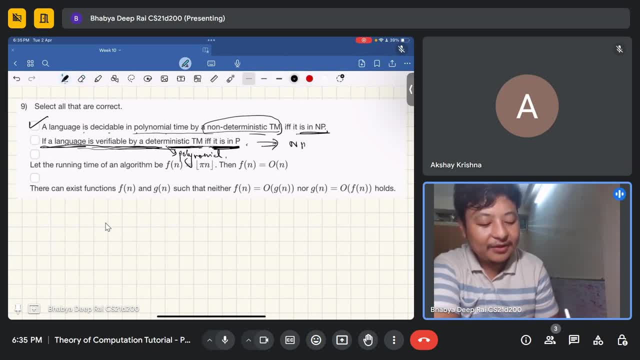 true, then this would mean: if this was true, then this would mean P equals NP. Then this would resolve the P versus NP conjecture, Because the left left half is definitely the definition of NP. So we are saying: a language is in NP if, and only if, it is in P. So it. 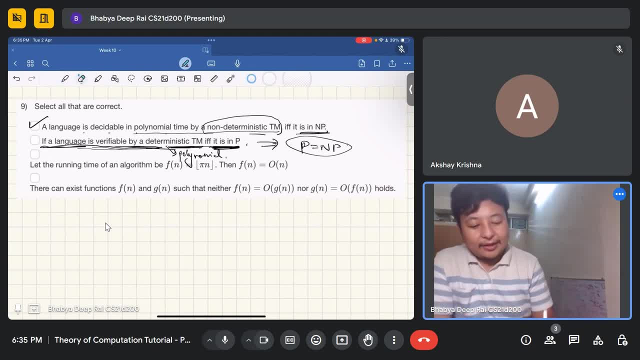 means P equals NP. it would imply P equals NP, But that is not true. So as soon as I, but not that it is not true. it is not known And it is not even given what the time is, what the time taken is, which will determine this question. So obviously this is not true. 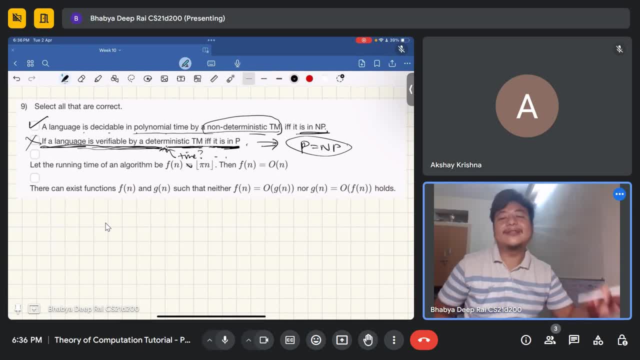 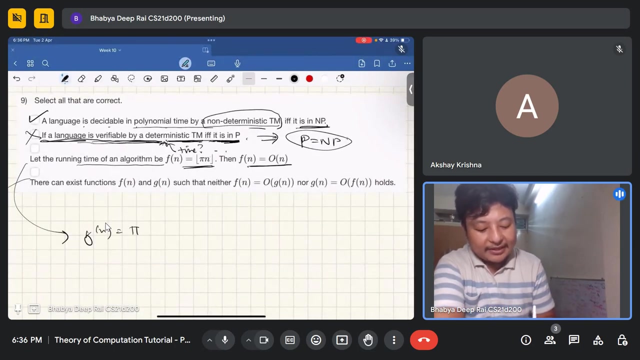 It is not known in the case of polynomial, and it is obviously false in the case of exponential verifier, and so on. Another question: Let the running time of an algorithm, fn, be pi n, then fn equals order n. And so let us see this question: fn equals pi n? floor of pi. 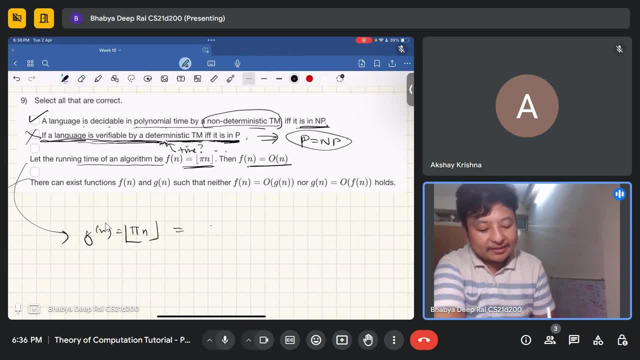 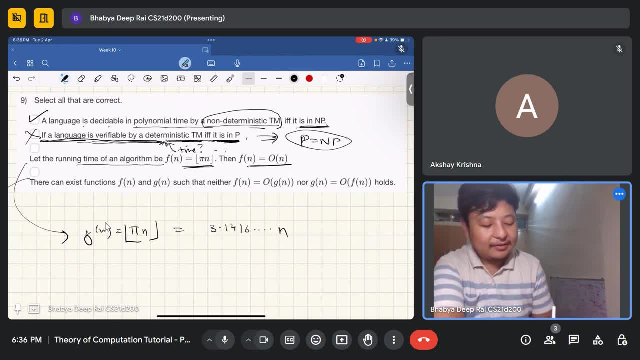 it is 3.5.. So it is 2.5.. So it is 3.5.. So it is 3.5.. So it is 4.5.. So it is 2.5.. So it is 3.5. So it is 2.5. So it is 3.5.. So it is 2.5.So it is 6.4, and so on times. 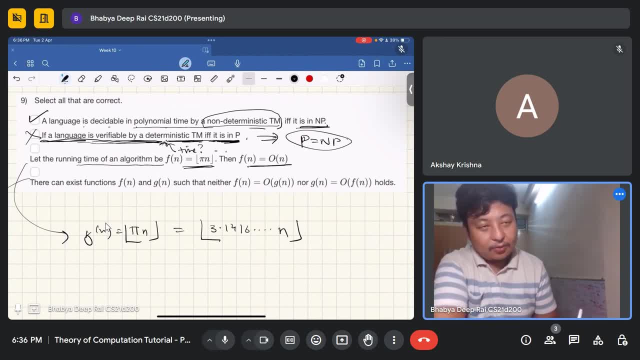 n floor of that. And now what I can do is let me look at Gn, which is 4 times n. Gn is 4 times n, 4 times n, which implies Fn is equal to order of n. So this is the constant, this is the 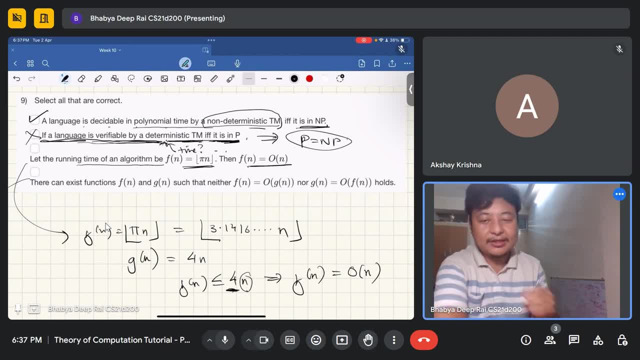 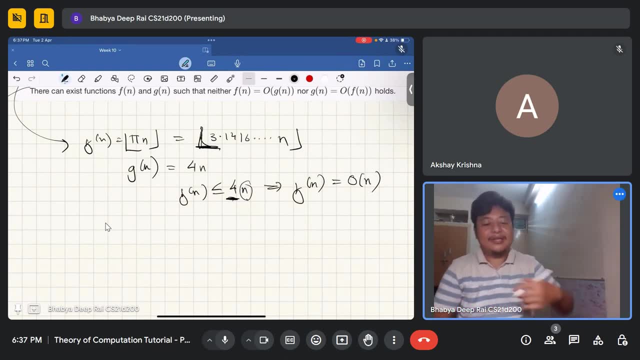 function. Function is n. this is the constant. It is bounded by some upper bounded constant because this floor, actually 3.14, will actually, even if this floor was not there, if the answer would still be the same. Even if this floor was not there, the answer would still be the 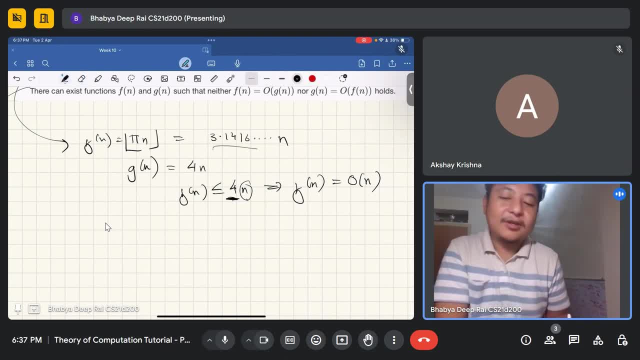 same, because 3.1416 is still bounded by 4.. Now that I have added the floor, I will only get a lesser value. By the way, floor means I am bringing down to the nearest integer, so 3.1.. 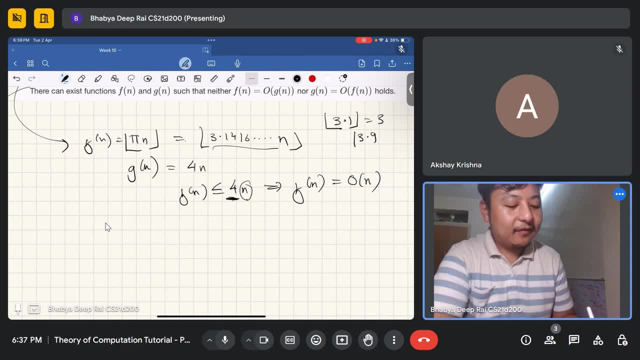 The floor is 3 and 3.9,. the floor is 3.. But if I do 3.9 and seal, this is called the sealing function. If I do 3.9 and the sealing, it means I round up to the nearest integer, The. 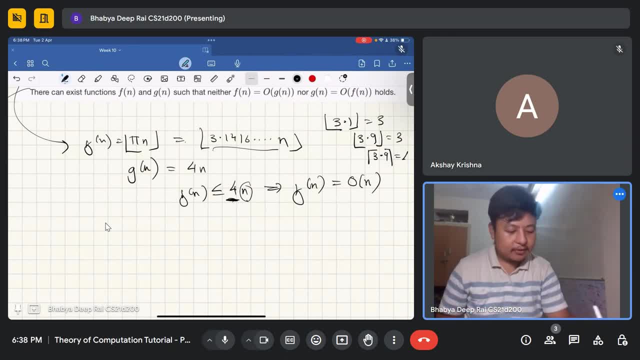 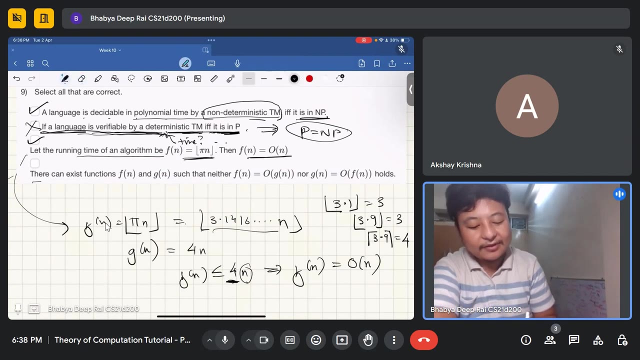 nearest integer above it is 4.. So you see where the difference is. So floor will give a 3 and the ceiling will give a 4.. So anyway, this is true. So the question is: there can exist functions fn and gn such that neither fn is equal to. 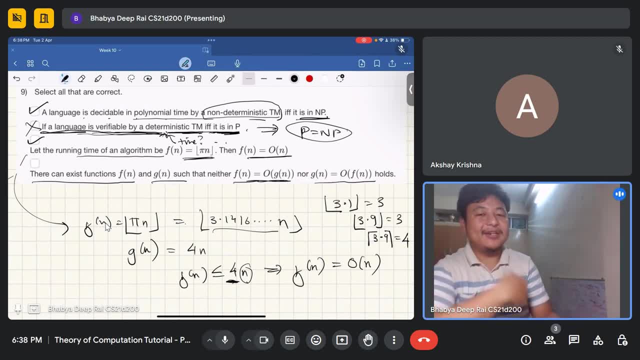 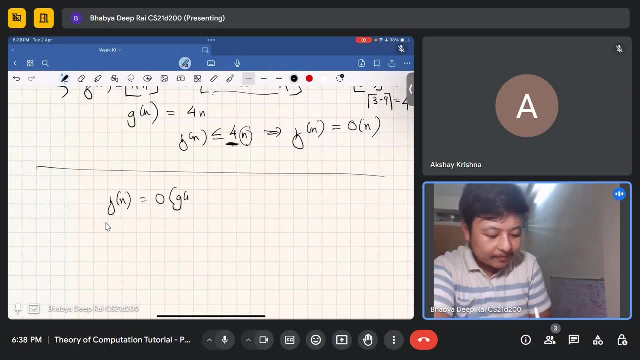 order of gn and gn is equal to order of fn. So this is interesting. So fn is equal to order of gn means in some sense it means that gn is always growing more than fn. So what does the graph look like if we remember, like, from algorithms and so on? 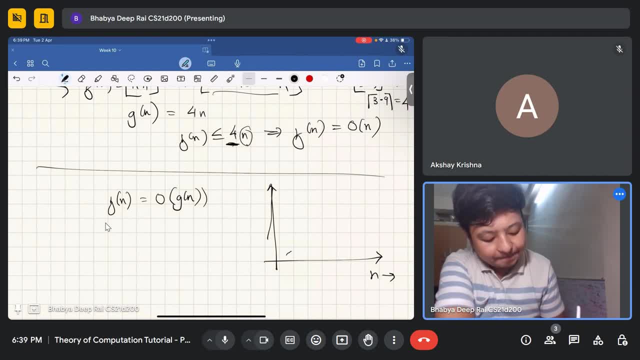 So this is like if we remember, like from a table. so, for instance, if we remember fn as in 1 side, so fn will always be equal to node 1, but gn will be equal to the node of fn, And this will take a lot if we will remember which is always 0 to 1.. So fn is always like. 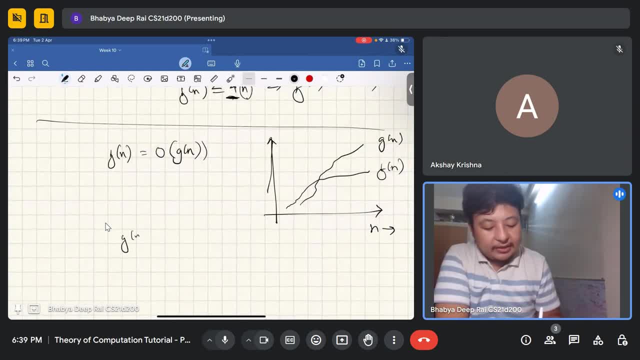 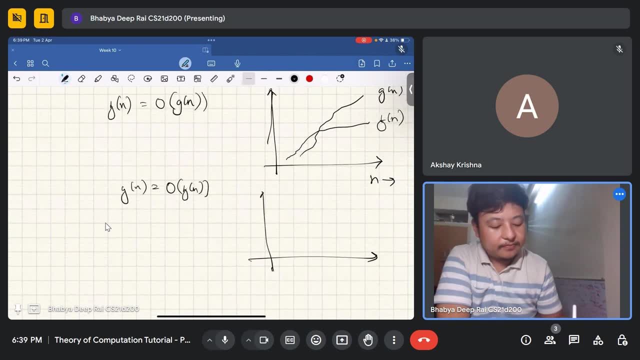 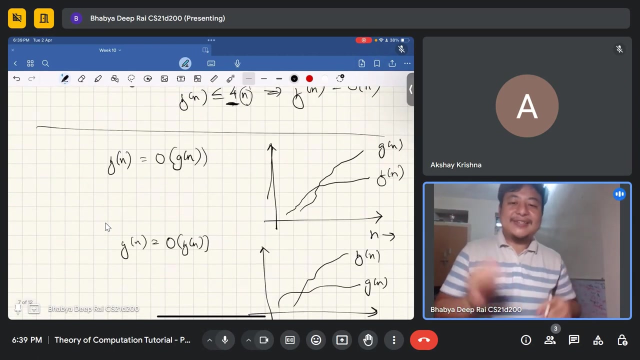 0 to 1, right, You can also guess. gn will growing down to over the edge of fn. So this is angle point. So for instance, that angle is 1.. Fn means Fn is always growing faster than G. Now can it be that both are growing faster? 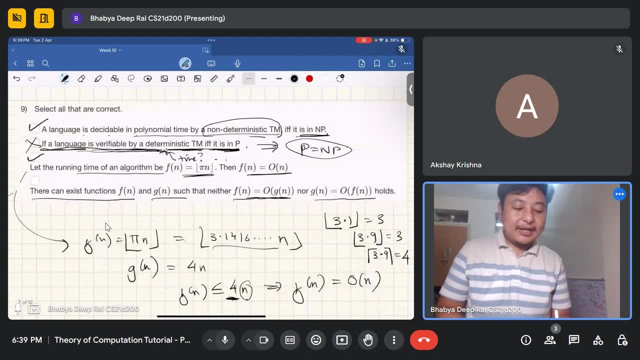 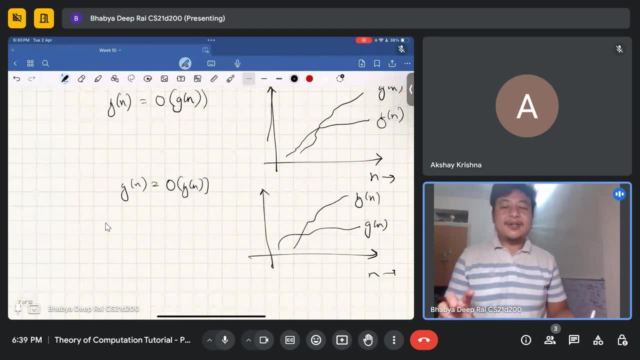 than each other. That is, neither Fn is equal to order Gn and Gn is equal to order Fn. Can we have something like this? It may seem kind of absurd, right, Something like that should not happen, we would think. But we can actually construct a function that actually satisfies. 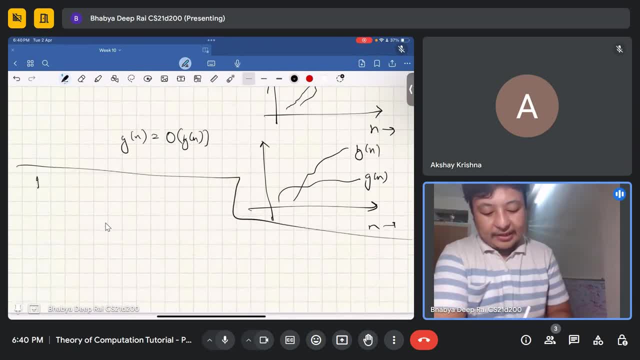 this. The idea is as follows: We want the function to be constantly changing in its behavior. We want Fn, Gn, Fn, And then Fn grows. Gn grows. At this point Gn grows faster than Fn. Then this: Now Fn is growing, Gn is. 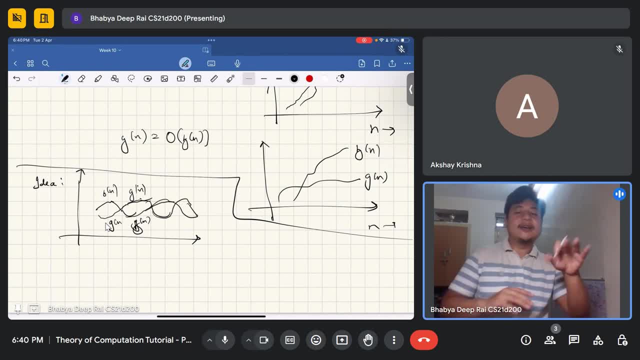 waving toward, and so on. So this is the idea that we would want to construct. We can simply do the following. So: 1, 2,, 3,, 4,, 5,, 6,, 7,, 8,, 9,, 10,, 11,, 12,, 13,, 14,, 15,, 16,, 17,, 18,, 19,, 20,, 21,, 22,, 23,, 24,. 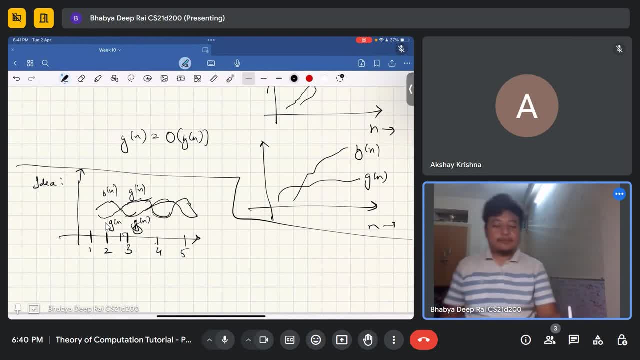 25 and so on. So this is n. So we notice that whenever we can construct a function, whenever that n is equal- n is 2,, 4 and so on- Fn is always above Gn, And if n is lower. 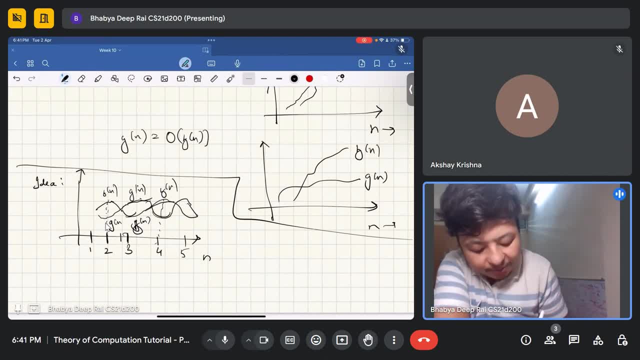 sorry, n is odd. for example, 1,, 3,, 5 and so on. There Fn is always lower than Gn. So this is the idea. So here we can define Fn as to be equal, to say n okay when n is even okay. 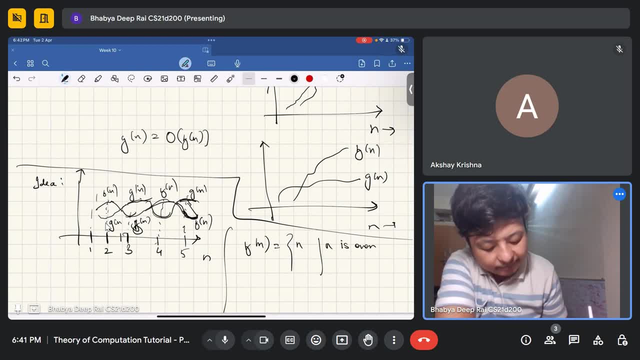 okay, and n minus 1 when n is odd, and g n is n minus 1 when n is even and n when n is odd. So whenever n is at even intervals- 2,, 4,, 6 and so on- f will always be above g n. So 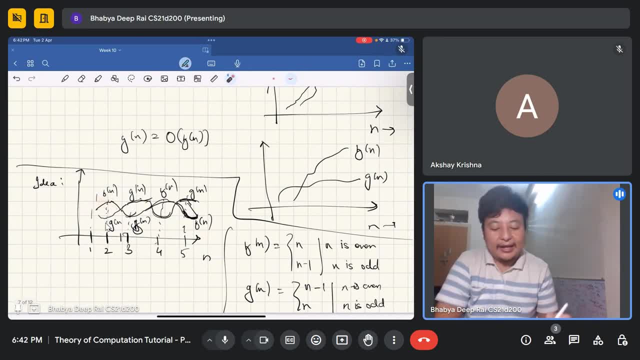 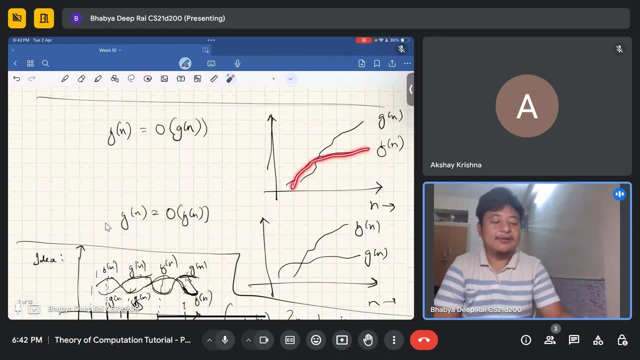 here, what do you see above g n? and if it is odd, then f will always be below g n. So you can never characterize it with this order notation. you can never say that, oh, f is equal to g n. You can never say this, that: 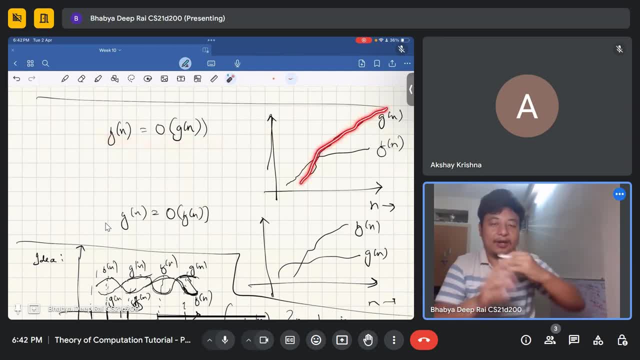 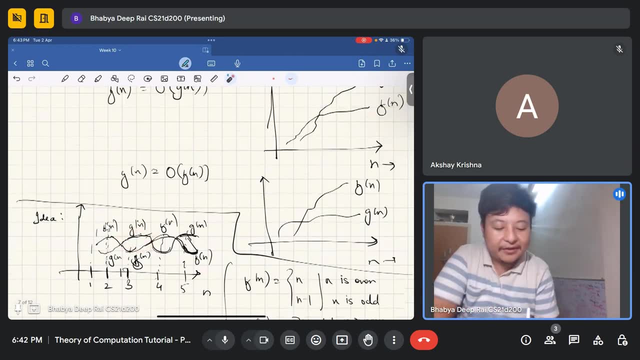 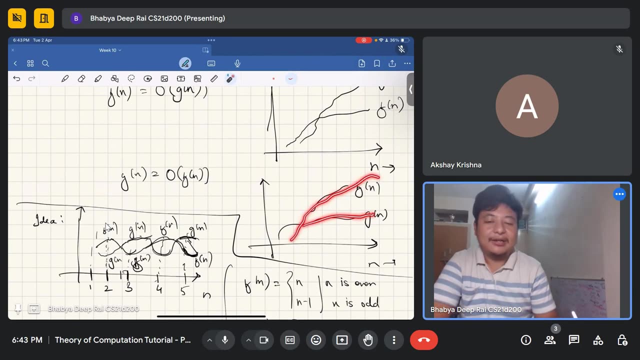 So f equals order g n, meaning that g n will forever and ever be above f? n. You cannot say: because f n, g n are changing positions, and you cannot say f g n is equal to order f n. that means f? n is always growing above g n after some point. 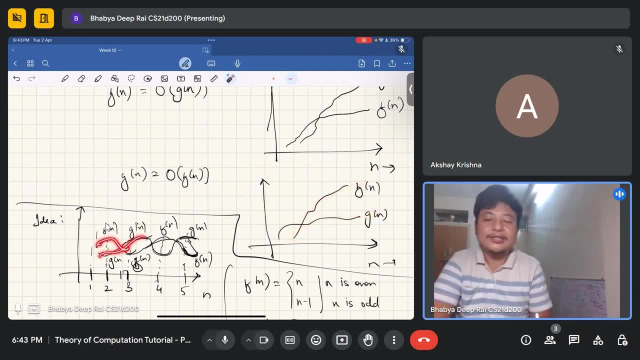 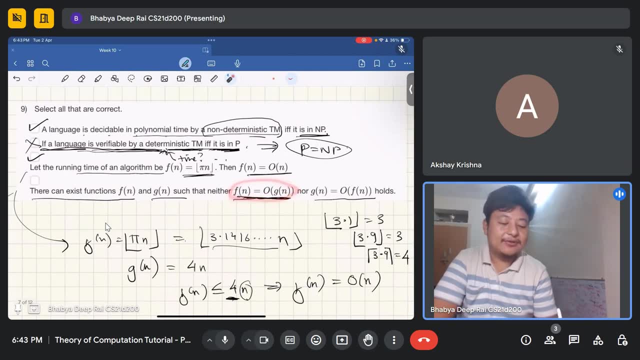 You can never say that because, again here, it is constantly changing. So this is an example of two functions that you can never put in this basket. f? n is equal to order g? n And g? n is equal to order f? n. both of them cannot be true. 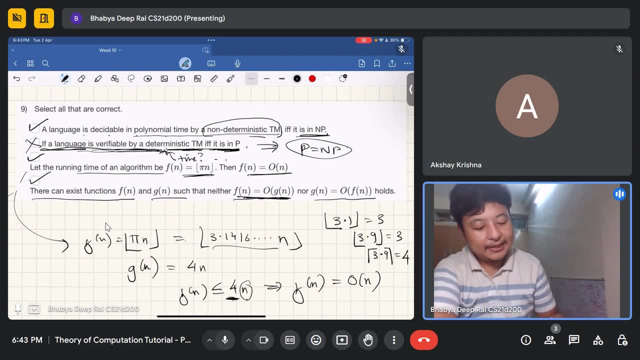 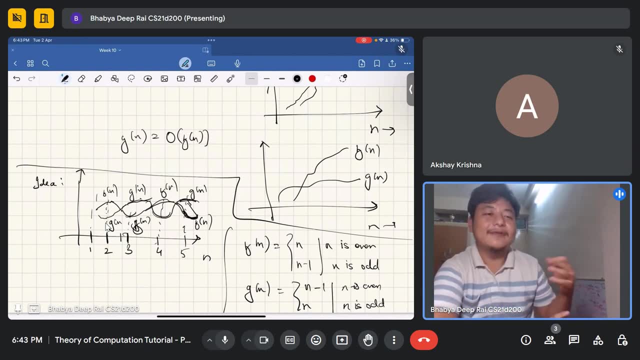 So this is correct. So another nice, a small by a small change. you can do this. but you can say like see, sir, this kind of function cannot even, we cannot never even hope to characterize it by order notation. So both of these cannot happen. so can you, because each of them are growing, decreasing. 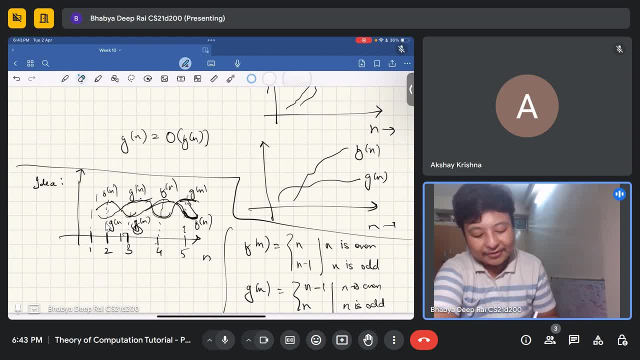 growing, decreasing and so on. So question is: can you make a function that is always growing and yet this property holds? So that is an exercise I would like to give you. The answer is yes and try. you can try it yourself. the I will show you diagrammatically, you want. 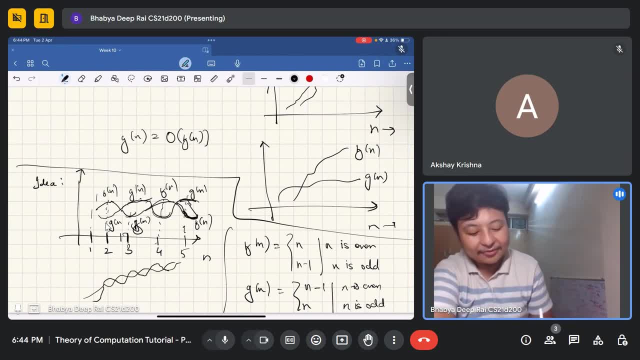 to do something like this. As you can see, the function is constantly growing also and it is, you know, above and below each other each time also. So it is a hybrid of growing function And this kind of idea, this flipping kind of idea. okay, yeah, so that is the end of question. 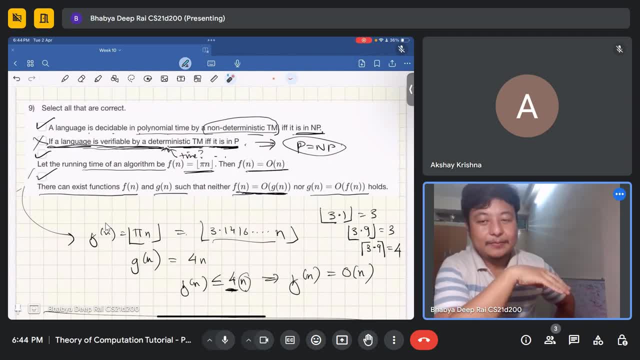 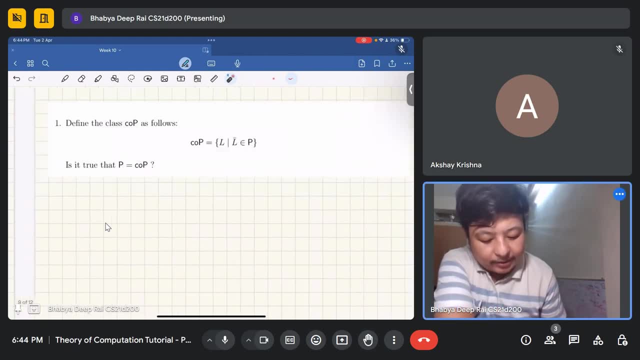 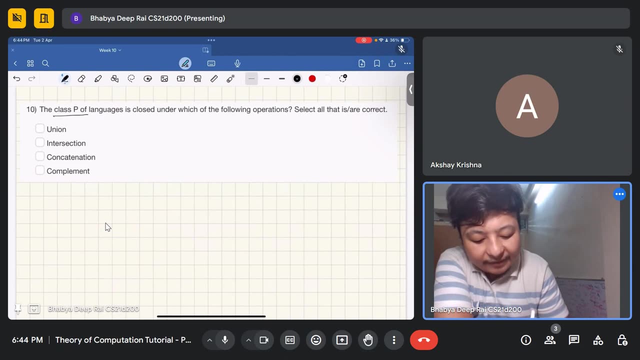 9. So any questions? is this clear? Yes, sir. Okay, let me know if there are any questions. So here is another question. this is the last question from the assignment, the class P of languages. It is closed. under which of the following operations select all that are correct. 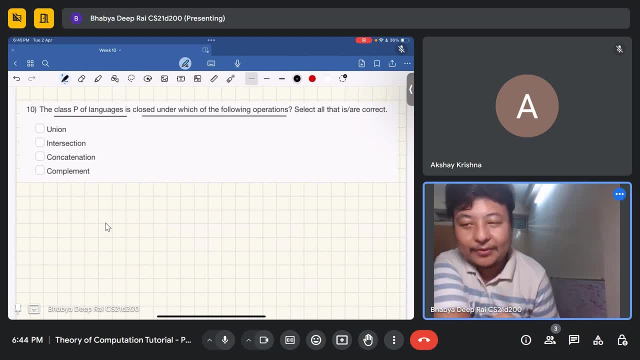 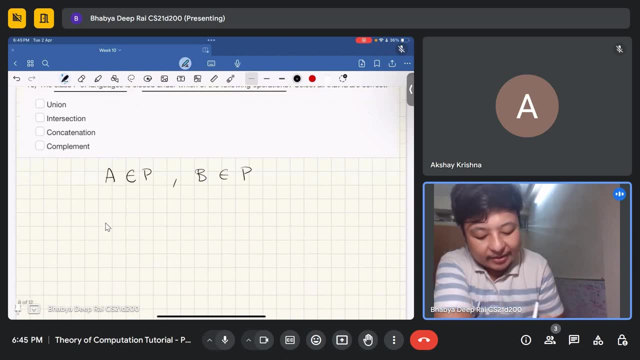 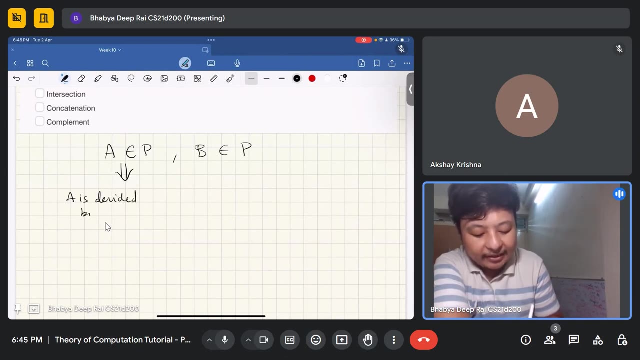 Now this is quite simple, actually. okay, so take any two languages: A is in P and B is in P. So what does it mean that A is in P? A is decided by polynomial time deterministic Turing machine Mx- Let me call it MA- and B is B is decided by poly time deterministic Turing machine MB. 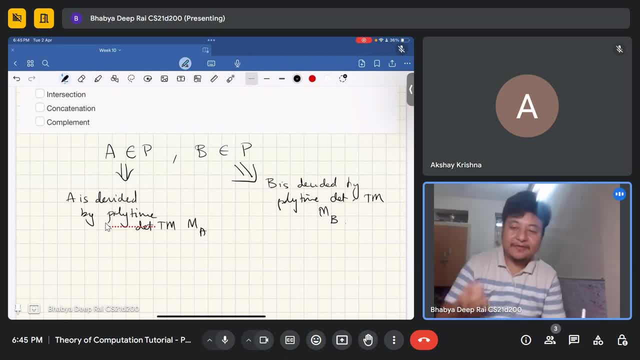 Okay, MA, the language of MA is A and language of MB is B, and each of them take polynomial time and they are deterministic, they are not non-deterministic. So the question is: is the union of the two? So the question is: is the union of the two? 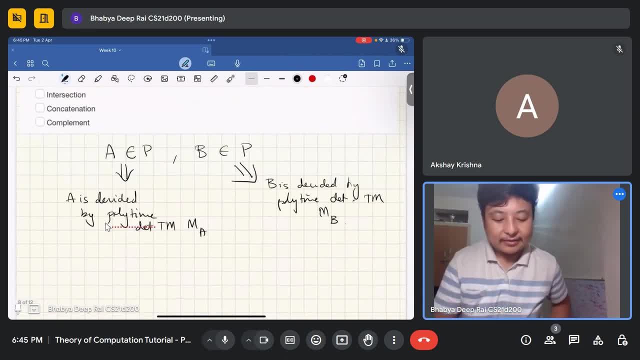 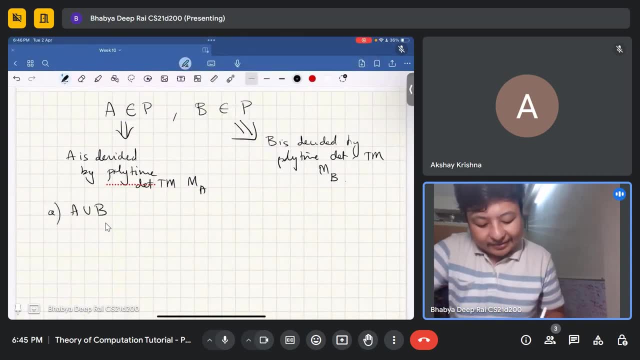 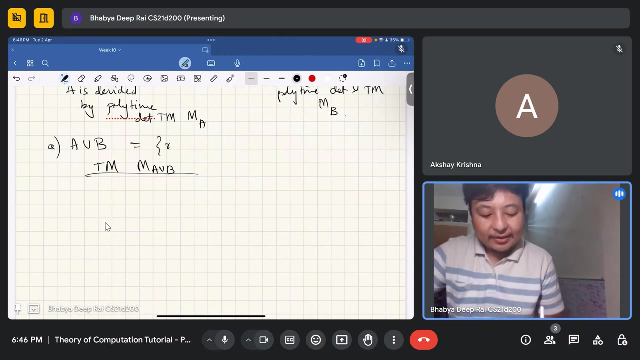 Is the union of these languages, is A union B? is this in P? answer is yes, okay, so I will call it M Turing machine, MA union B. okay, what I will do is: what is A union B? A union B means all the x, such that x in A or x in B. 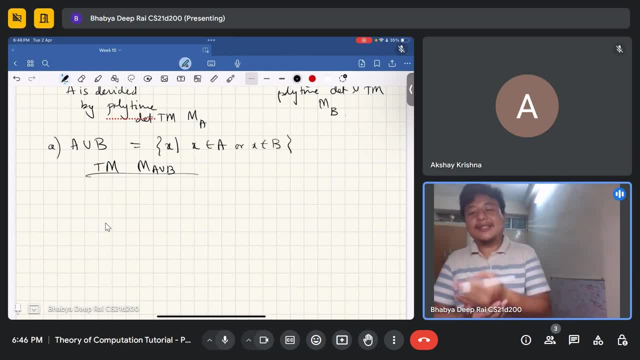 So what I can do. Okay, So what I can do, I can first check whether it's in A and then check whether it's in B. if, in either case, okay, run input is x. okay, run MA on x. if it accepts, then accept. if no, 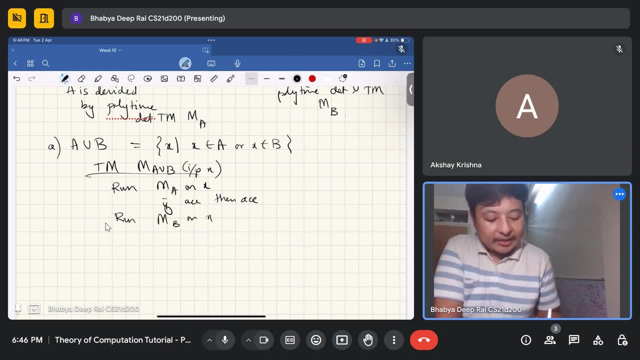 then run MB on x. if it accepts, then accept, otherwise reject. So if it is in A, then it will be accepted here. if it is in B, will be accepted here. if it is in neither, then it will not be accepted. but anyway, A union B will not contain those. 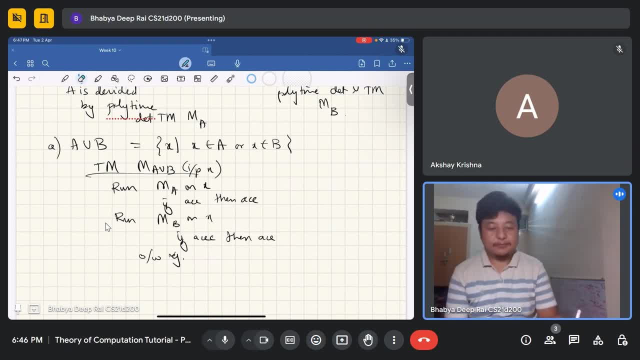 kind of strings. Okay so, and this guy takes polynomial time on N and this guy also takes polynomial time on N. total polynomial plus polynomial is always a polynomial, so it will only take polynomial time. So total, it will take polynomial time, and this is a deterministic simulation. so A union. 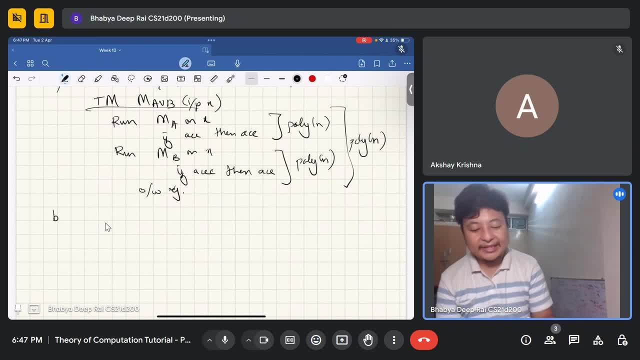 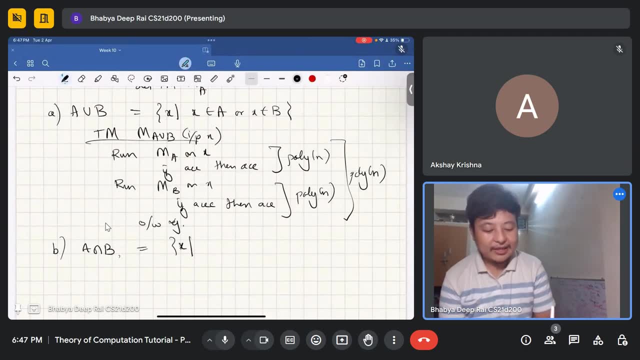 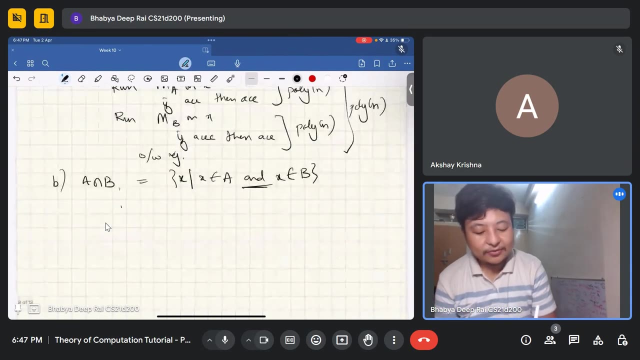 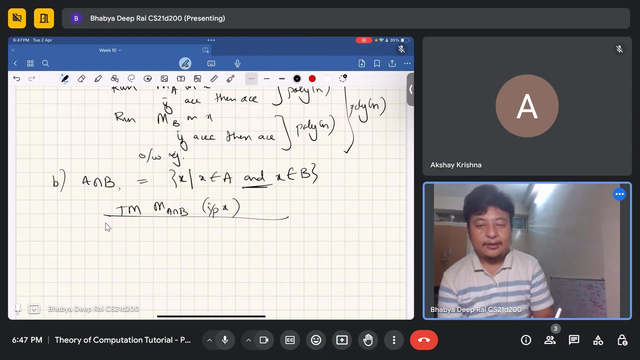 B is in P. Next is A intersection B. What is A intersection B? all the strings that are in A as well as in B and in B. So what is the Turing machine? look like the Turing machine. MA intersection B on input x. it's simple, it's similar. okay, we run on A. 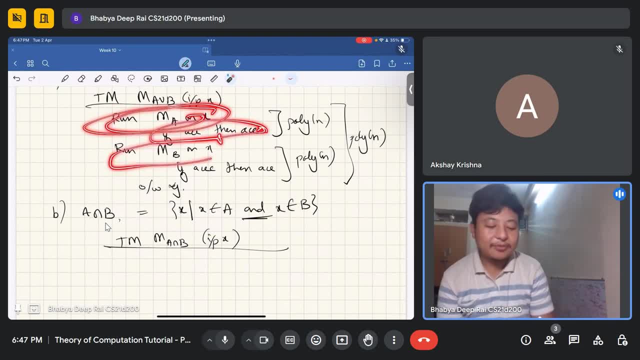 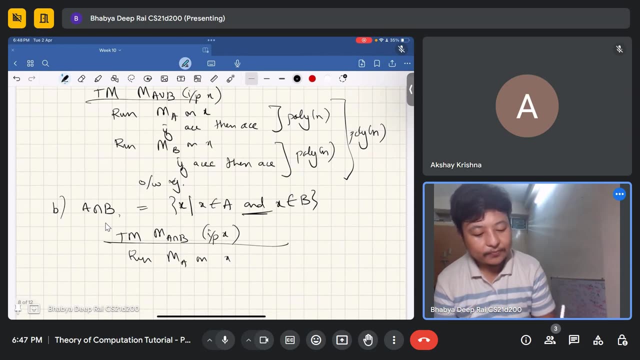 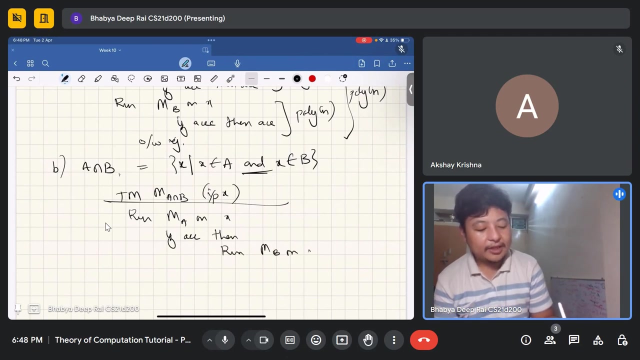 Okay. Okay, If it accepts, then we'll run on B also, and if it accepts, then I'll accept: come here, because it needs to go through both the checks. so run MA on x. if it accepts, then run MB on x. if it accepts, then accept x. 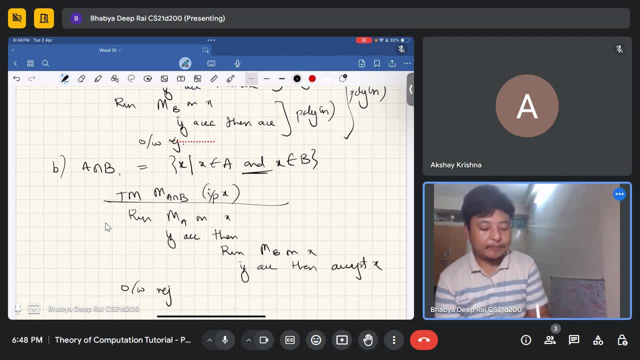 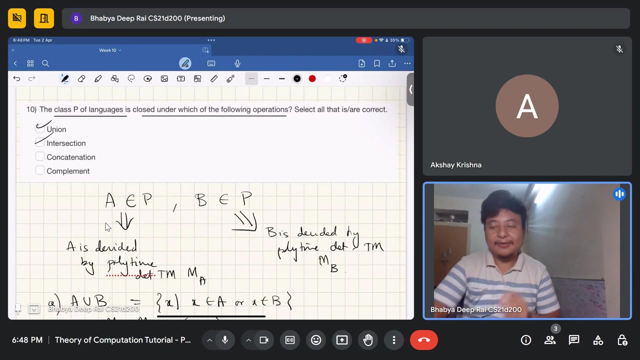 Okay, Otherwise reject because of the fact that it needs to be both in A and B. it needs to be accepted by both machines, MA and MB. So this guy takes polynomial time and this guy also takes polynomial time. So total will take polynomial time. it's in P, it is decided it is in the class P, concatenation. 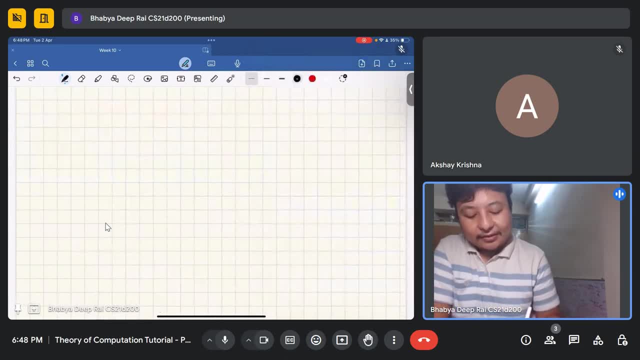 is the same approach, Okay, Concatenation. so A concat B is x, y, such that x is in A, y is in B. so here it's slightly more, or x, okay, Right, Okay, Okay. So it's x equals x equals u, v, such that u is in A, v is in B. it's a concatenation of: 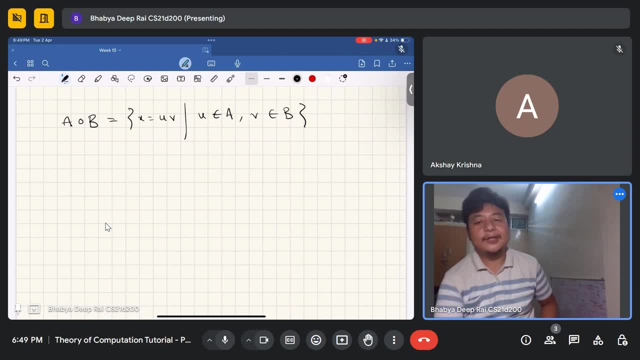 two languages, right, two strings in different languages. Now here, now the concatenation could have happened at any point. say 0 1 1 0 1 0. say 0 1 1 belongs to A. Okay, 0 1 0 belongs to B. so this should be accepted in A concat B. but we don't know where to draw. 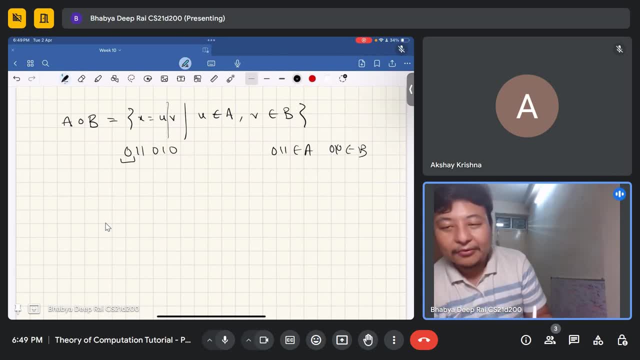 the line: Okay, We don't know, we need to. then. then what do we need to do? we need to check whether this is in A. this is in B. this is in A. this part is in B. this is in A. this part is in B. this: 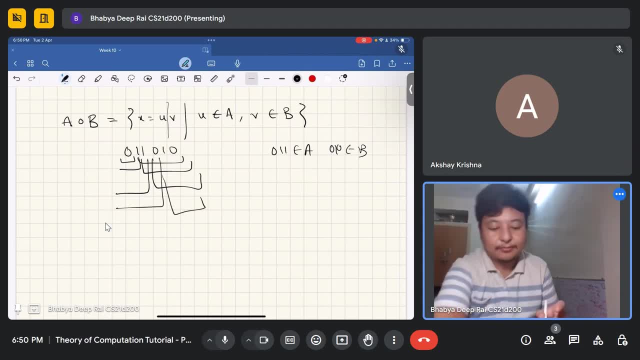 is in A and this part is in B, and so on. Okay, I won't write the algorithm might get a bit complicated, but the idea is that if you have x, Okay, Then I'll check whether this part is in A and this part is in B. then I'll check whether. 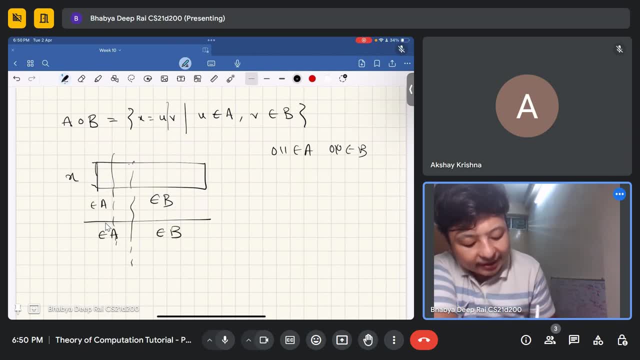 this part is in A and this part is in B, then I'll check whether this part is so. how many parts do I need to check? I need to check 1 n minus 1, 2 n minus 2, and so on. I need to check x 1.. 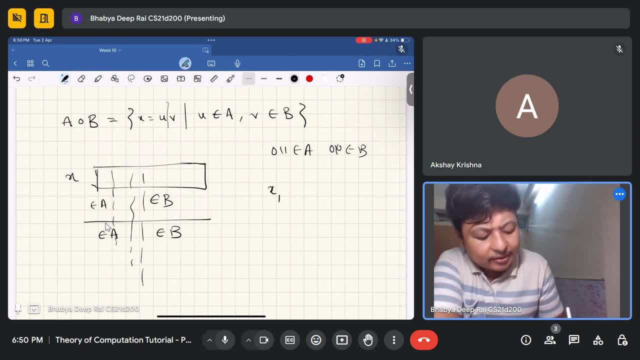 Okay, Okay, x 1 to x x 1 and x 2, so on till x n minus 1 and x 1 x 2, x 2, x 3 till n minus x n minus 1, x 1, x 2, x 3, x 4 till x n minus 1.. 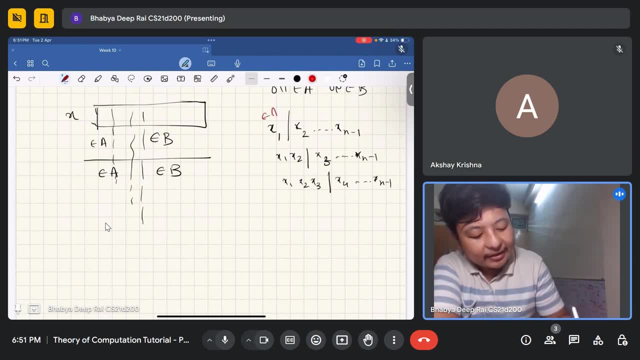 And check whether this is in A and this is in B. this is in A, This is in This. Oh god, okay, This is in A, this is in B. this is in A. this is in B. i need to keep checking and if it so happens that in both the cases that is in a and it is in b, it 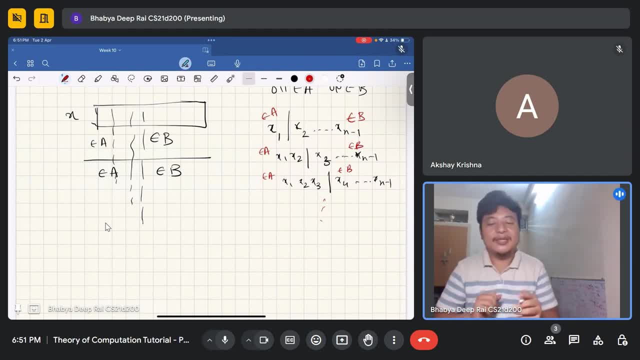 means it is a concatenation of two strings that are in a and b and therefore it should be accepted. but how many times do i need to do this? i need to do it only n many times, right? how many times? n times? because first i need to check for x1, then x1, x2, then x1, x3. 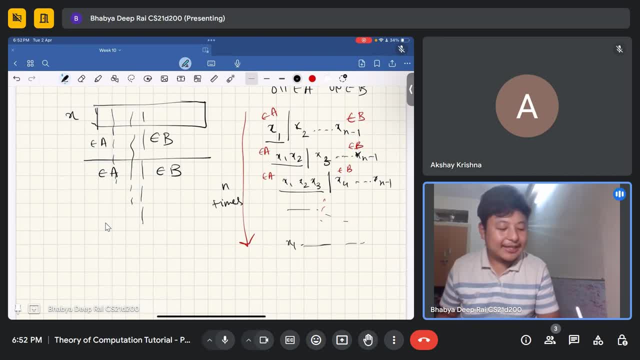 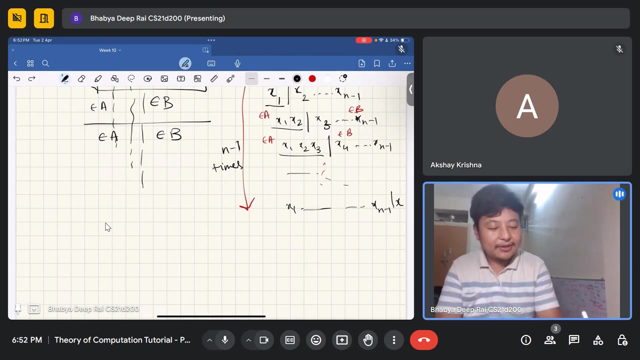 and so on, till x1, till xn minus 1 x, so it's not n times, it's n minus 1 times, and each of these n minus 1 times. i'm running machine a to check whether it's in the. i'm rushing running machine ma and to check whether it's in b. i'm. 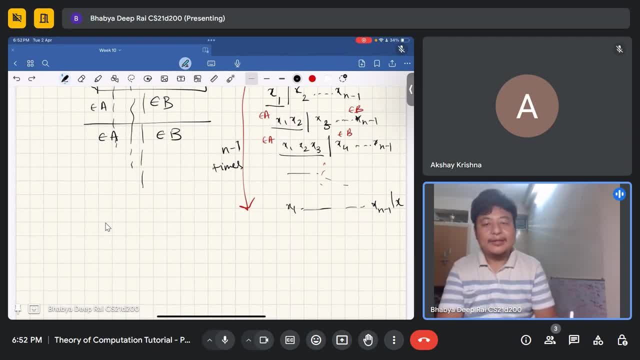 running machine mb, right? so i'm doing n minus 1 times. what am i doing? i'm running machine a plus time taken by machine a plus time taken by machine b, which is some n minus 1 times polynomial, which is also polynomial, right? so this also takes polynomial time. 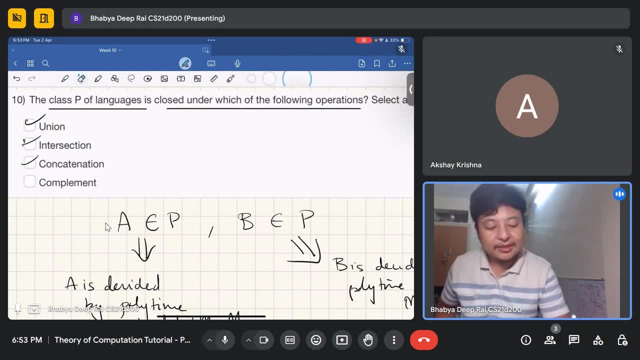 is even simpler. complement is much simpler. complement, just what you do is you just simply run the machine a and if it says yes, say no. if it says no, then say yes. the time taken is only polynomial right, because you are running the machine once and you are not doing any. 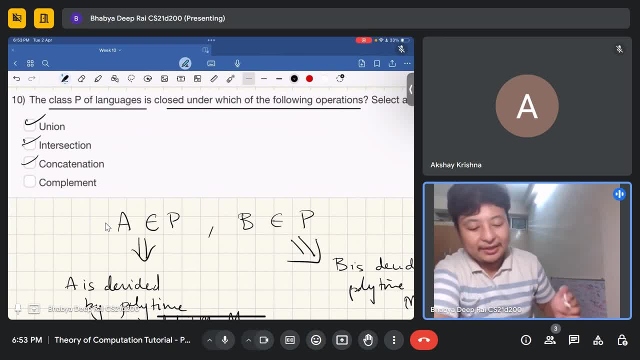 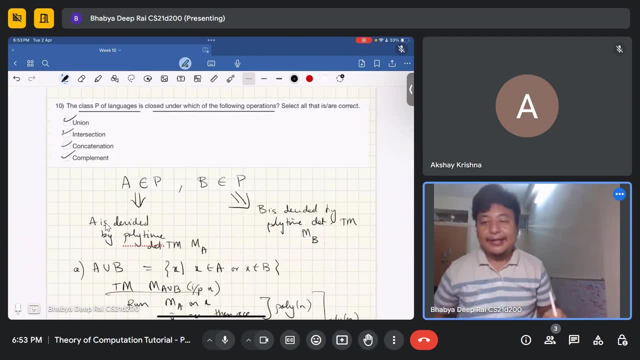 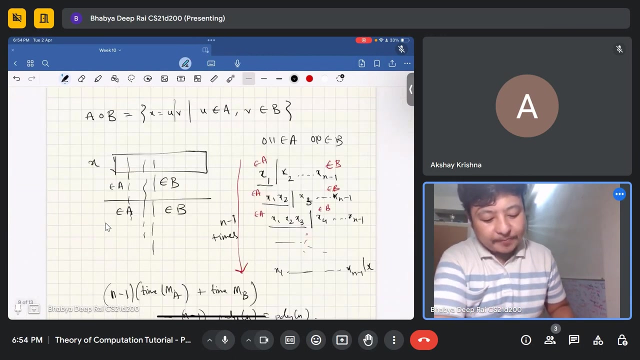 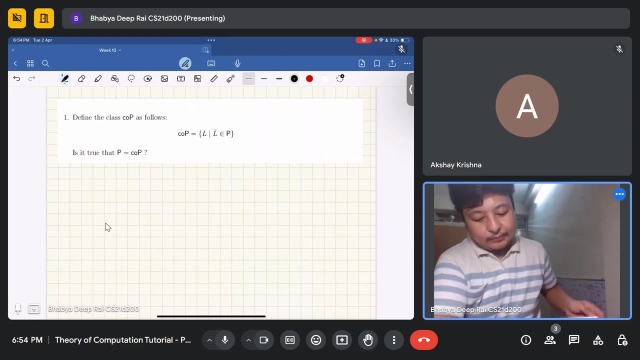 extra function. the yes and no will only take some constant time, and so complement will also be there. so this is: this means that the class p is closed under union intersection. complement and concatenation. okay, so clear, right. okay, now let's move on to this week's topic. so yeah, i have a few questions here. 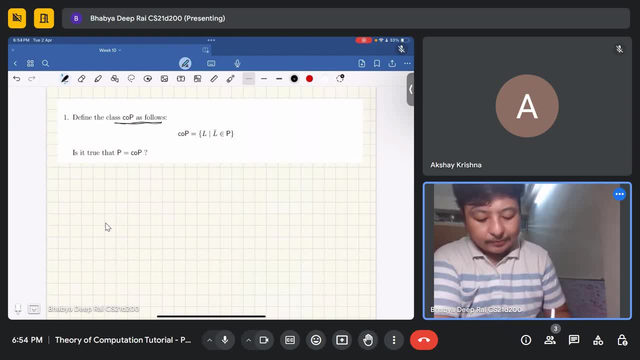 so define the class copy as follows: okay, copy is just the set of complements, that of the languages that are in p. it is the set of all languages such that its complement is in p. question is: is p in copy? okay, i just realized that the answer is in the previous question. 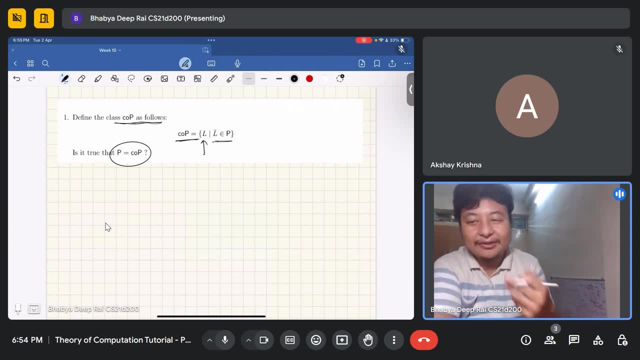 that we solved, okay. the question is: is p equal to copy? but what does it mean that p is equal to copy? let's look at that, okay, that is, p is contained in copy and copy is contained in p. this is the question. this is the meaning. okay, so what i mean by this is, if i have a machine for p, okay, or in other. 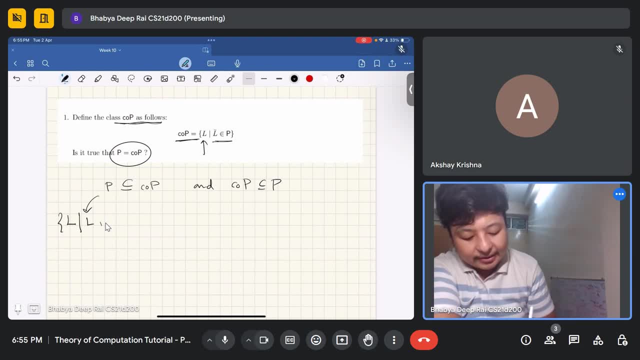 words. i have a set of languages such that l and cp- okay, so in this case- is decidable in polynomial type. then I can decide in co, P also. so, which means that the complements- okay, the complements- of these languages are also in P, and we've already seen that that is true, but I will explain it again, okay. 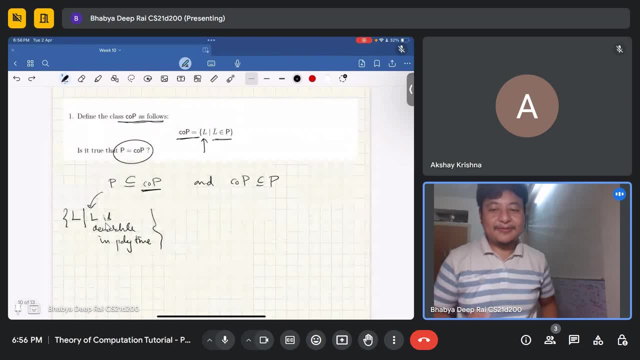 and I'll all these terms seems, but what it actually means is: let's let's look at this: is co P contained in P? but is co P all the languages such that L bar is contained in P? now what does it mean to say that it is contained? co P is contained in P. it means that all this entire set is 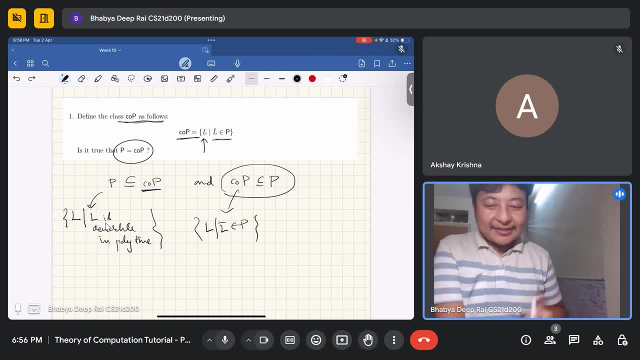 contained in P. if it means this entire set is contained in P, it means each of the languages is in P, and I'm going to describe the terms that these terms P. So what does this mean? This means L bar is in P, then L is in P. This is what the 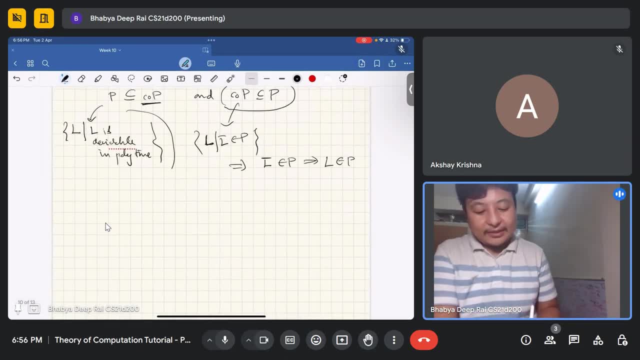 statement would mean: Similarly, if you look at this, if you look at this copy, you want to show that P is contained in L such that L bar is in P, Which means that any language in P- what is this? P? L such that L is in P, Any language in P, and we are seeing both. 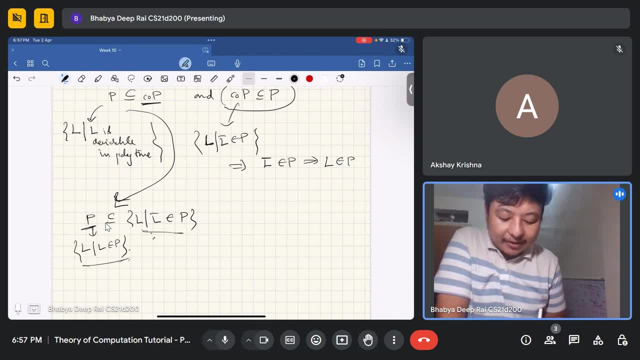 of these are equal. both these left hand side and right hand side are equal, which means that any L here, its complement, is also in P, Which means L is in P. then L bar is in copy. L bar is in P or L is in P means that L is in copy, which means that L bar is in P Together. 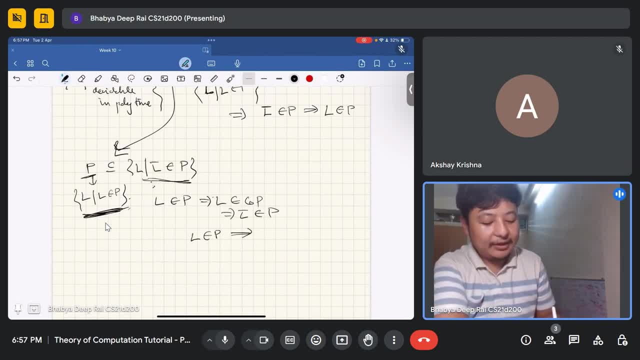 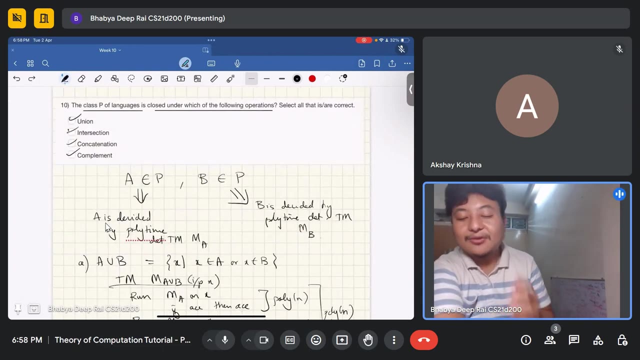 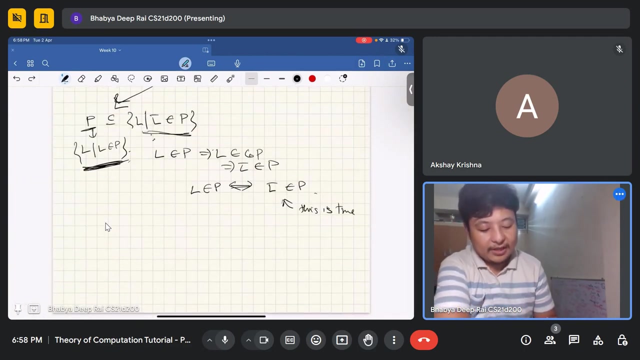 what does it mean? L is in P if, and only if, L bar is in P? Is this correct? Answer is yes. This is true. Why? This is this part of this question. P is closed under complementation. This is true Why? Because if L is in P, then there. 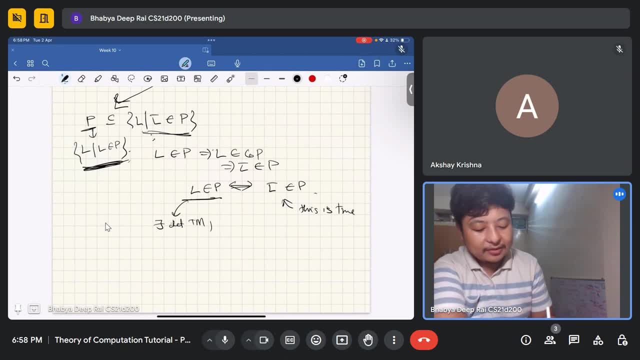 exists a deterministic Turing machine, polytime Turing machine, and if i want to decide l bar, l complement, okay, all i need to do is the run machine m, if it says yes, then i give a no, if it says no, then i give a yes, and this procedure takes polynomial time. so even the complement i can decide in p. 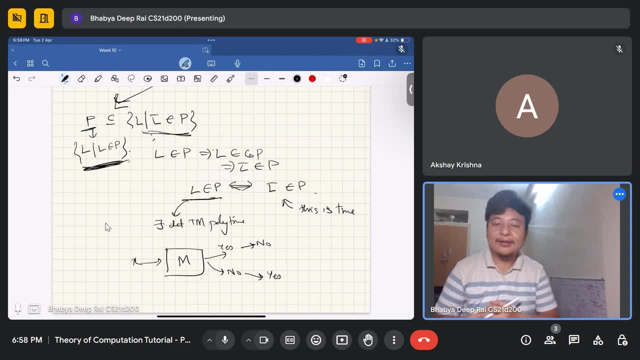 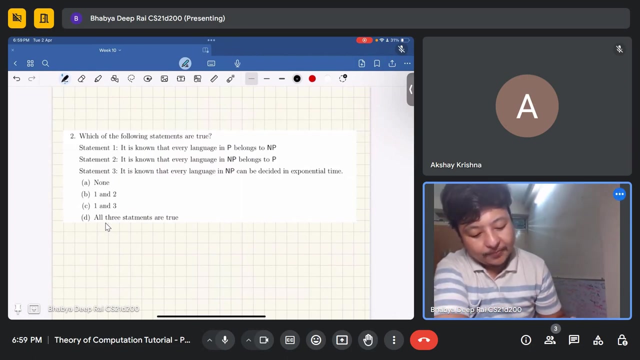 if the complement i can decide in p, it is contained in copy, right, and therefore, uh, copy is exactly the languages of complement can be decided. therefore, p is equal to okay, yes, sir, okay, so now, uh, yeah, here is a nice warm-up on p and p and so on. 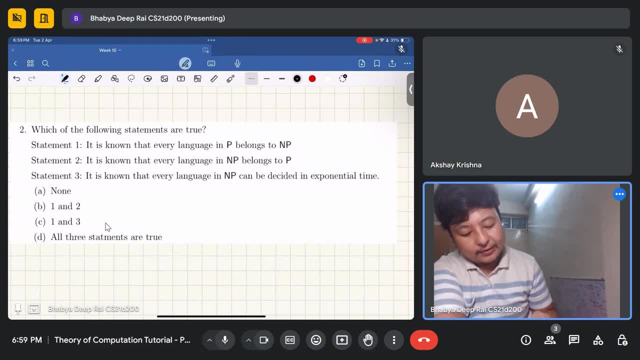 so, uh, the question says: uh, it is known that every language in p belongs to np. okay, okay. so which of the following are true? that is a question, so statement one says it is known that every language in p belongs to np. two says: it is known that every language in np belongs to p. 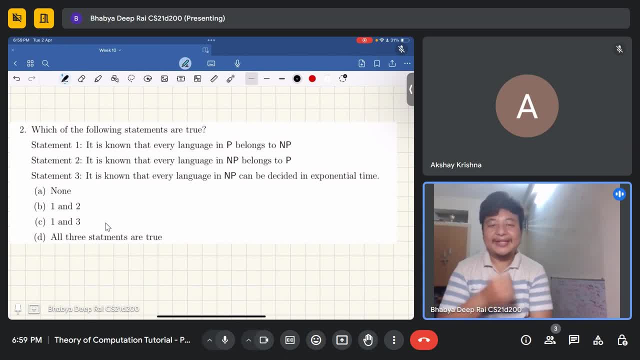 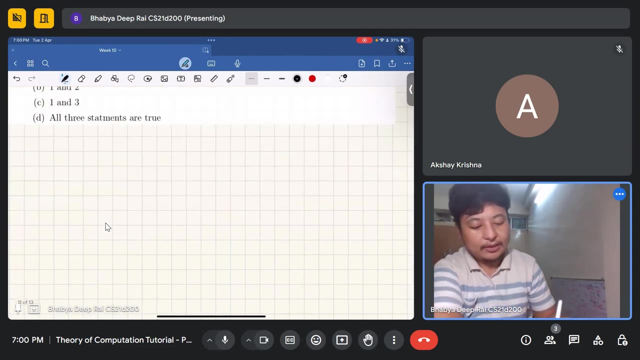 and statement three says: it is known that every language in np can be decided in exponential time. so which of these are true? let's look at the first one. uh, every language in p belongs to np. this is true. we know that. this is true. we know that p. 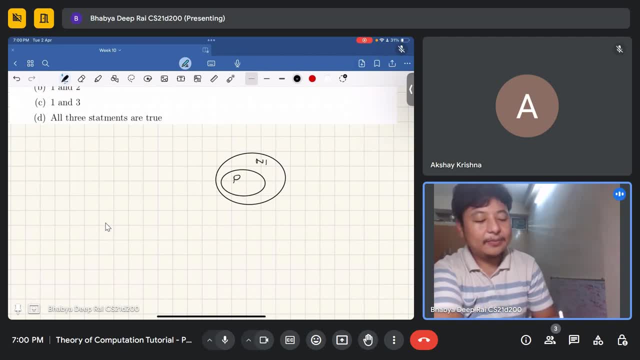 we know that p sits inside of p. why? because, i mean, there are various ways you can explain this. one way is that p has a deterministic time turing machine that runs in polynomial time- okay. deterministic poly time turing machine: okay, m runs in. uh, okay, any language here. l okay has a. 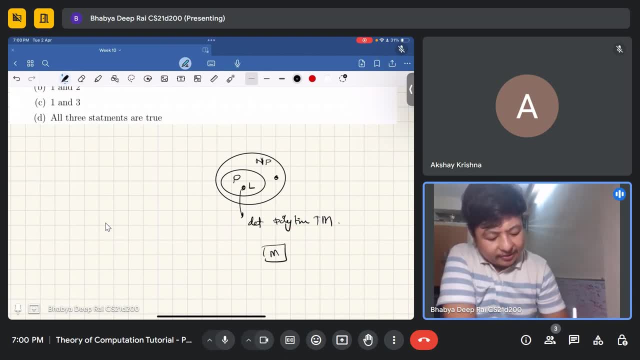 deterministic polynomial time turing machine And any language. here L prime has a non-deterministic polynomial time Turing machine. Now any non-deterministic Turing machine. let us say I do not make use of my non-deterministic power at all. 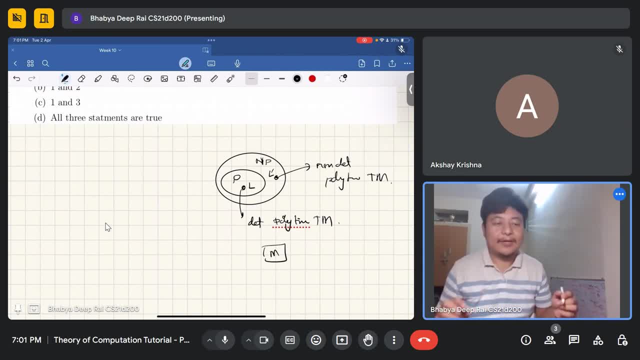 I do not make any non-deterministic choices on the way. What is a non-determinism? Non-determinism means I have the power of guessing. I can move into several states, several configurations, at the same time. Let us say I do not use my power. 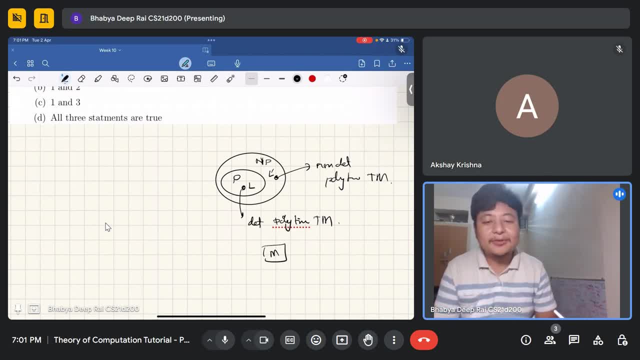 I just go one by, one by one, I form a deterministic polynomial time Turing machine. So a deterministic Turing machine, polynomial time Turing machine, is just a weaker version of non-deterministic polynomial time Turing machine. It is still a non-determinism. 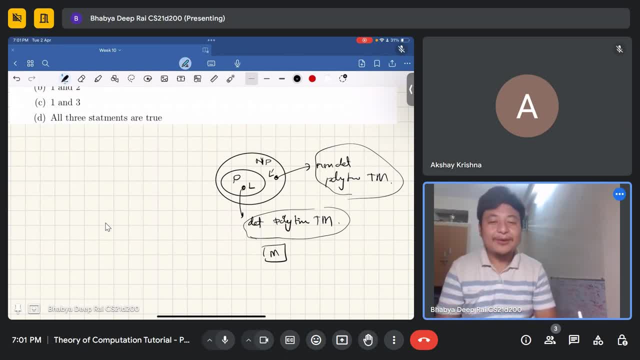 It is still a non-deterministic polynomial time Turing machine where I do not use non-determinism at all. So any language in P Is therefore trivially in NP that way. This is the first way to answer this question. 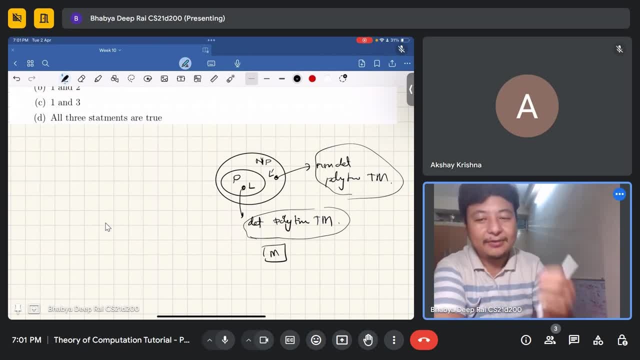 Second way to answer this question is by the second definition of NP. Remember, NP has two definitions, two standard definitions. One is obviously: it has a non-deterministic polynomial time Turing machine. The second definition is that: Yeah, the second definition is that. 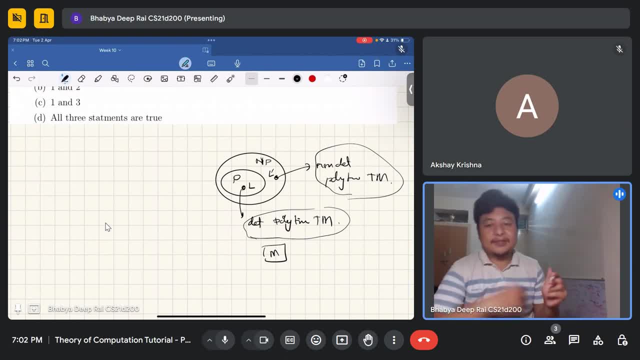 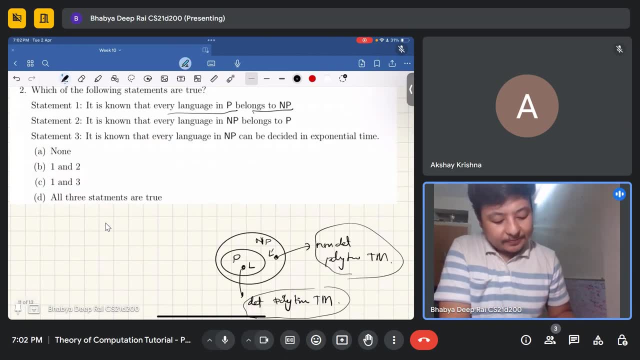 It can be verified in polynomial. There is a small size certificate which can be verified in polynomial time. OK, so that is what the second definition is, And any P language can be verified in polynomial time because you can give the input itself as a certificate. 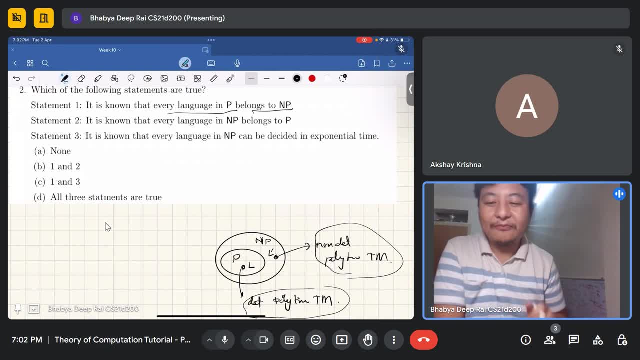 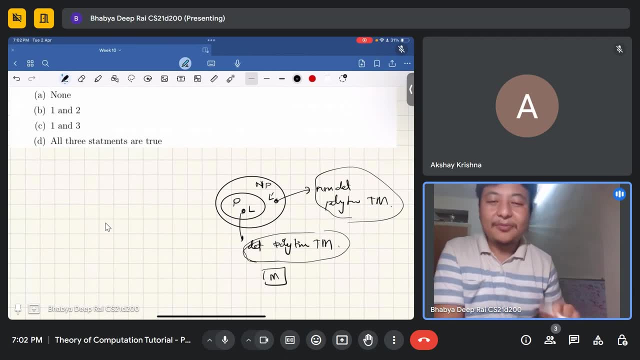 But I will, I won't. I won't go very deep into it, Just remember this much by this trivial logic. OK, that didn't any deterministic Turing machine is actually a non-deterministic Turing machine also, but it's slightly weaker. 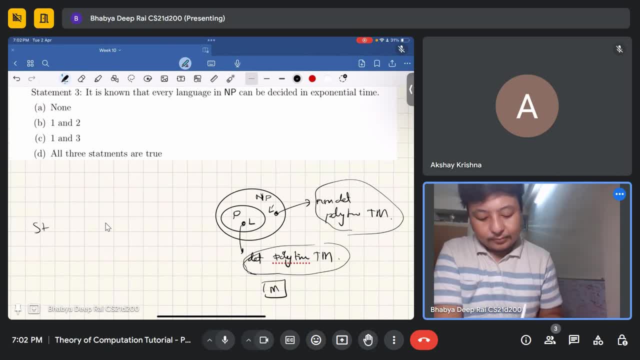 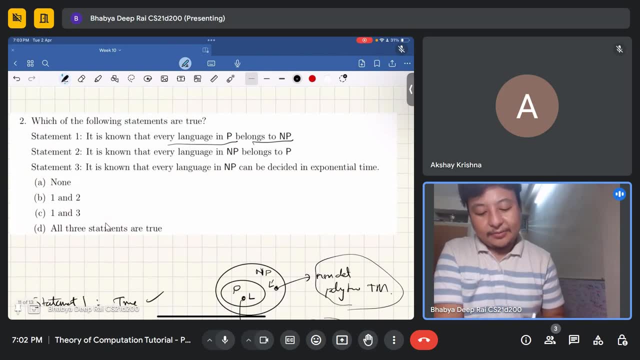 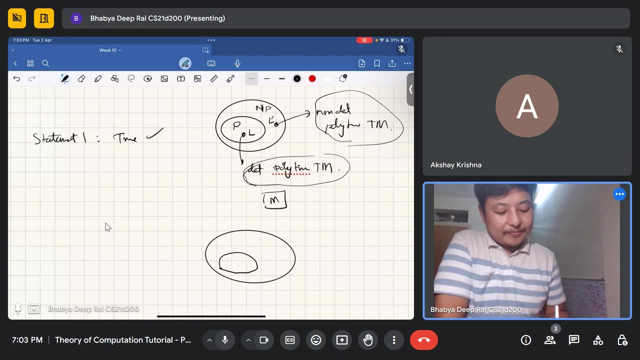 So say that one is true. True. Let's look at the other statement. It is known that every language in NP belongs to P. Now, this, Every language in NP, That is, NP, is a subset of P. they are saying. but we already said, said that P is a subset of NP. right now, state meant to. let's look at two. 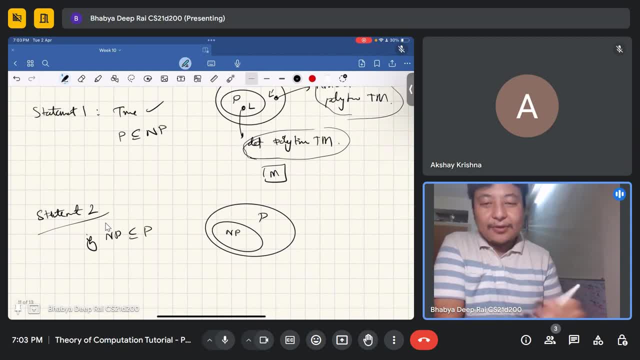 If NP is a subset of P and it is already known that P is contained in NP, then it would mean that only this is possible, right? P is equal to N. How can two sets be subsets of each other, even only if they are equal right? 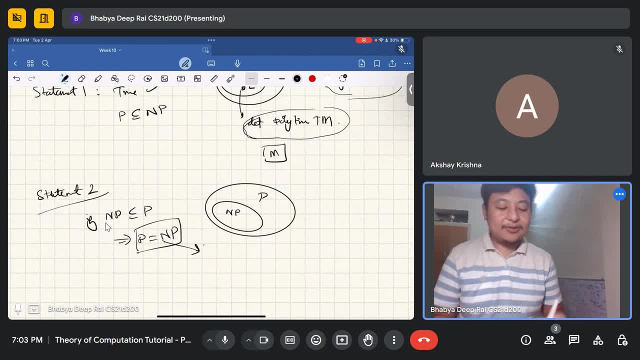 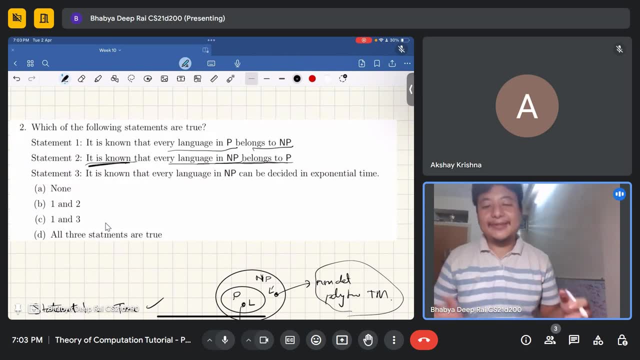 So P is equal to NP, then this conjecture would be solved. So it is known that every language in NP belongs to P. It's not saying that it's incorrect, because it may be correct We don't know, But the fact that it is known we are saying. the statement two becomes false. 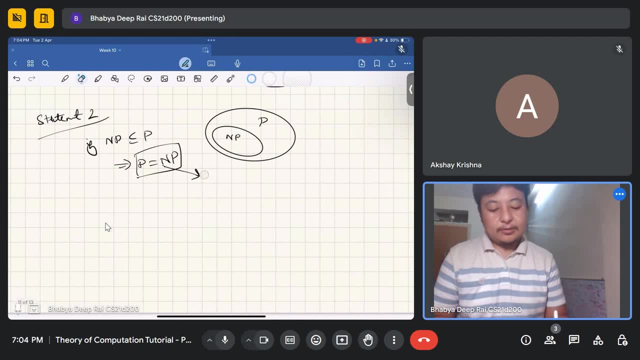 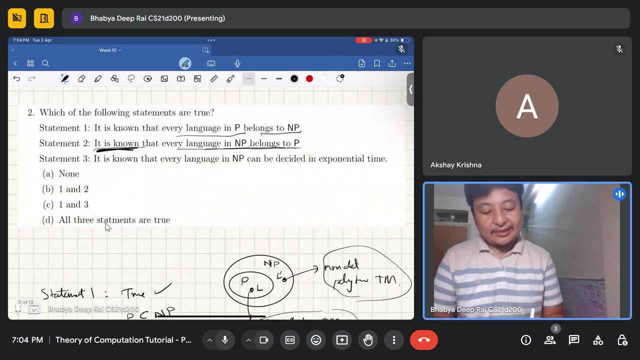 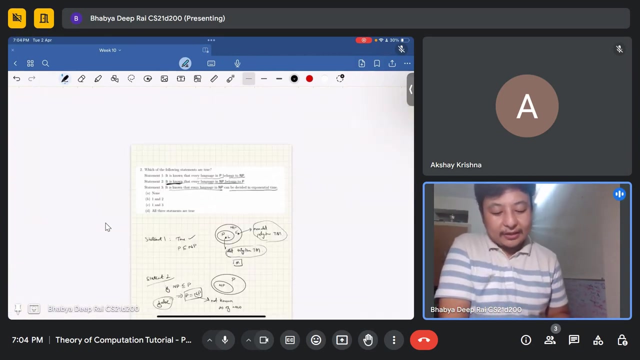 It is not known. Not known as of now. Okay, So statement two is false. Finally, statement three says it is known that every language in NP can be decided in exponential time. This is true. We saw this already Here. 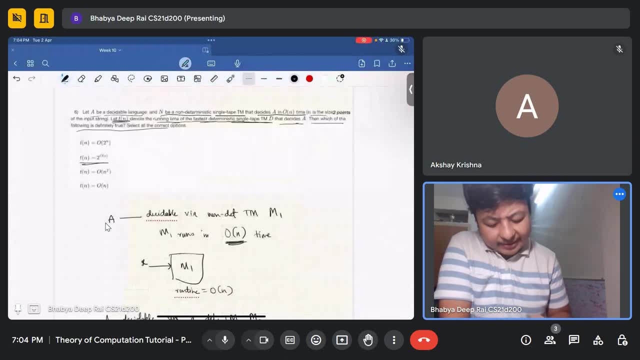 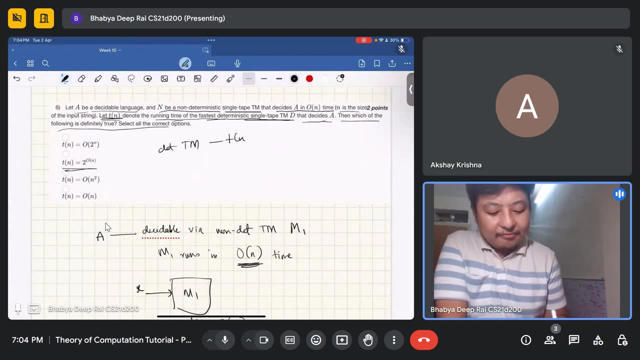 Here In this question it says a deterministic Turing machine takes T and time. Okay, Then there is a non-deterministic Turing machine that takes 2 to the order n time. Sorry, not T and time. order n time. 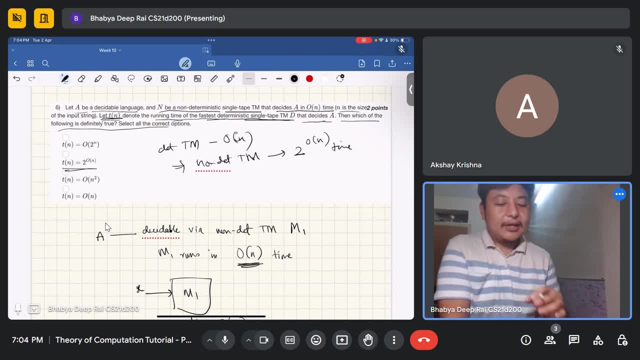 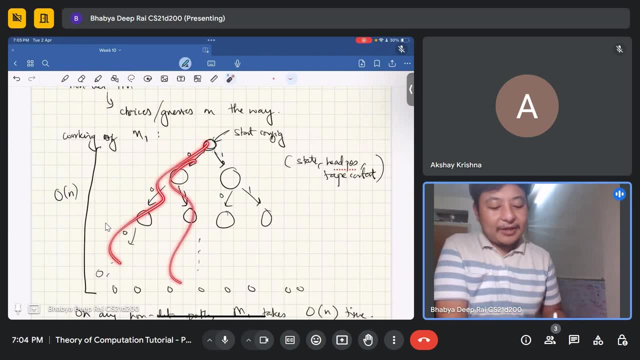 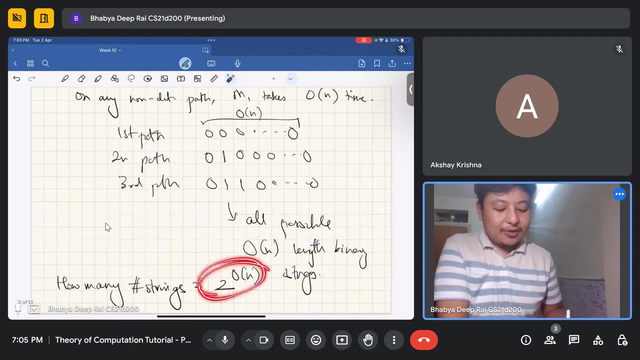 2 to the order n time. So using the same simulation. okay, using this approach that I explore every path. If, instead of order n it was taking some polynomial time, then I need to explore 2 to the polynomial many paths. 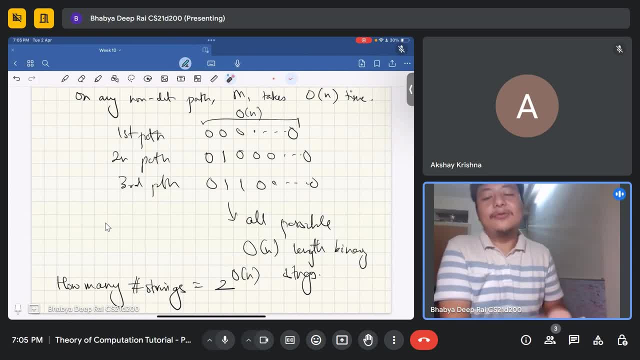 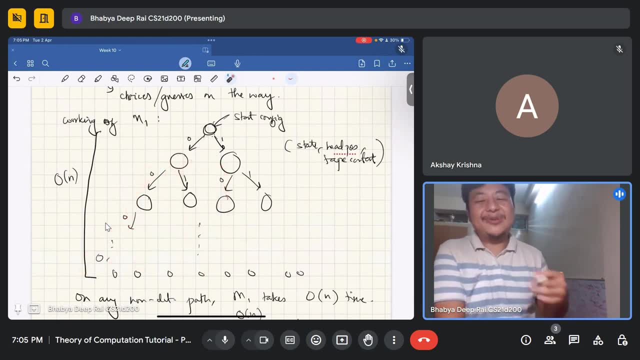 Okay. 2 to the polynomial many certificates, in other words. or 2 to the polynomial many paths. And because it can make so many non-deterministic choices, right, I am just exploring each one of them. I am going brute force. 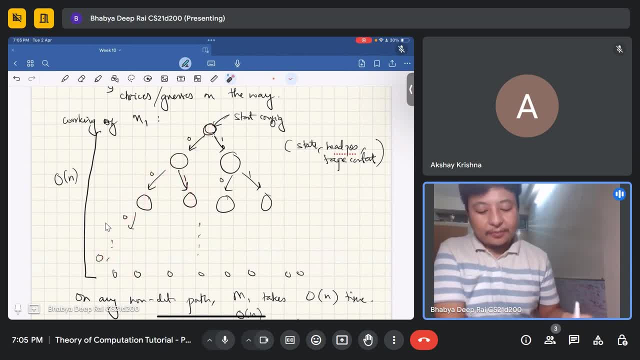 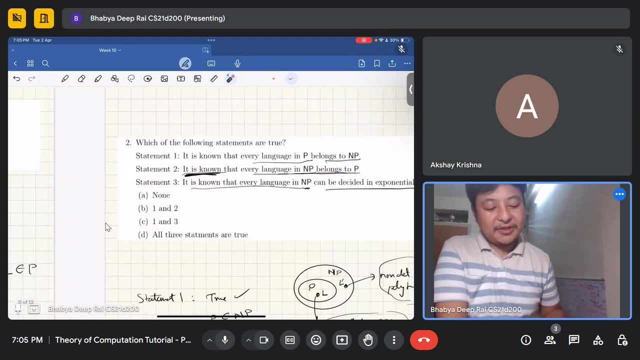 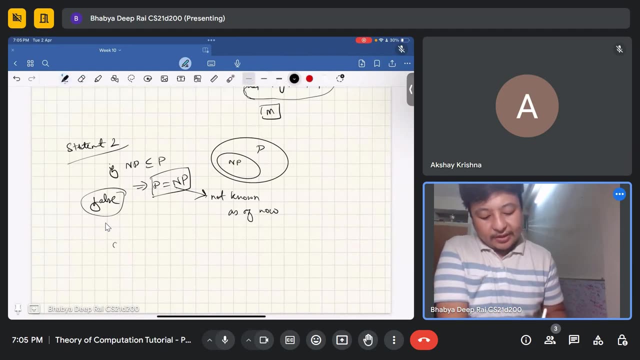 How many of these paths are possible? 2 to the polynomial. in our case Here, if instead of order n add polynomial, So this takes exponential time, Exponential time, Okay. So statement 3. If say, Turing machine m takes polynomial time, then Turing there exists a non-deterministic 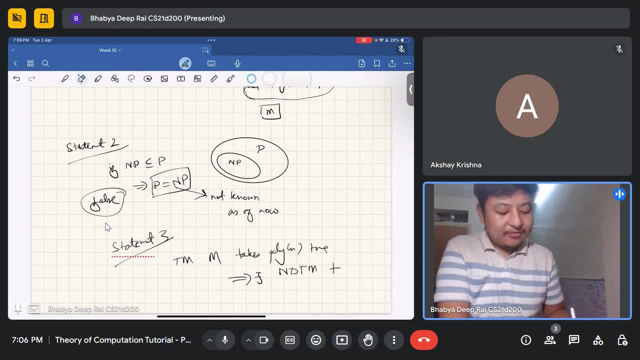 Turing machine, Oh, not non-deterministic Turing machine, Oh, okay, okay, okay, sorry, There exists a non-deterministic Turing machine that takes polynomial time. Sorry, I explore each path. Okay, And that takes. there exists a deterministic Turing machine that takes 2 to the polynomial. 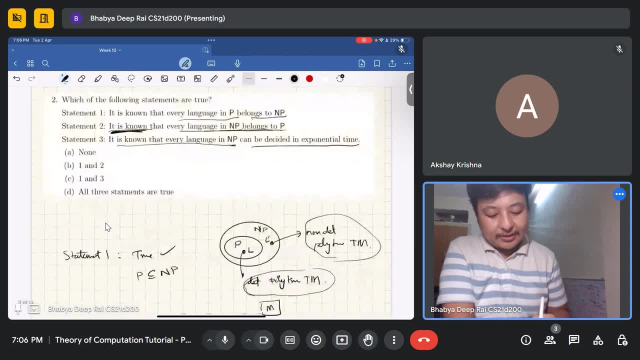 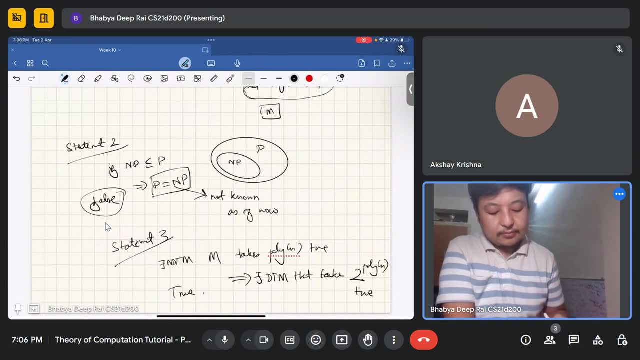 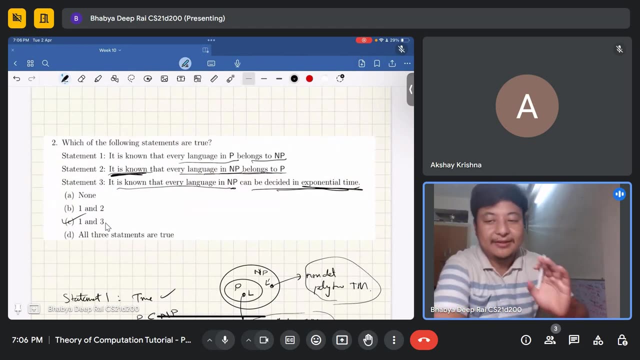 time, which is exponential. Okay, So this is true. Statement 3 is true. So 1 and 3 is the answer. Okay, Is this clear? Yes, sir, Okay. Okay, So this question, is it correct? 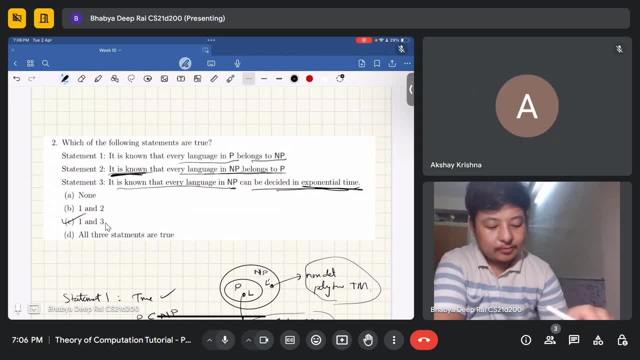 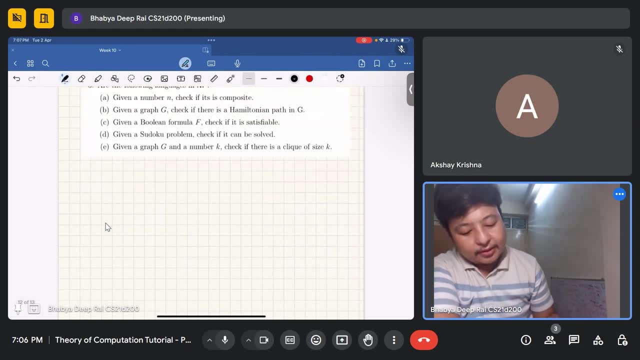 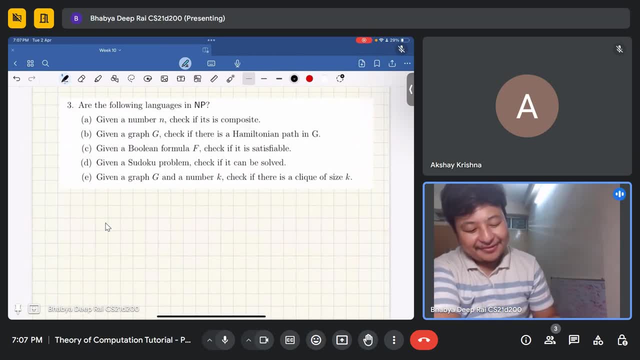 Okay, I forgot to include one question. I can include it right now, so no problem. But this question I'm not doing because I think you were also there when we did this right- Finding certificates, finding small site certificates. So it was done in the previous session. 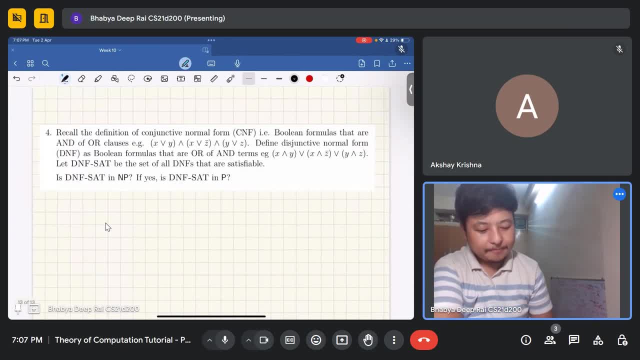 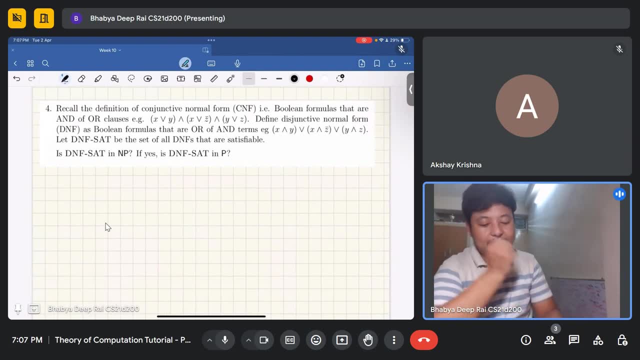 So, yeah, this I'm not doing. Okay, there's one important question I need to add here. Okay, but before that I'll jump on to this question. So recall the definition of conjunctive normal form, CNF, Boolean formulas that are AND of OR clauses. 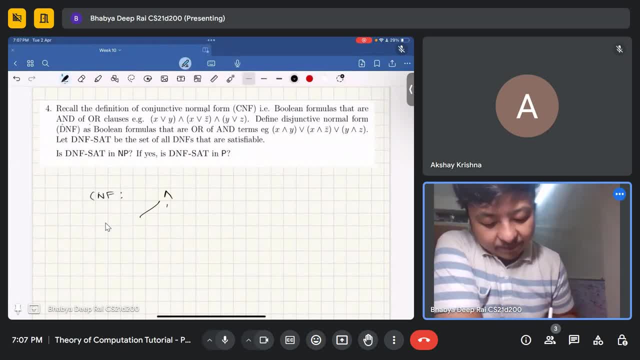 So CNF is of this form AND of ORs, For example. this is an example of a CNF. So this, we did it in the lectures, Okay, and you can see that it's the same thing. right, We are doing ORs first. 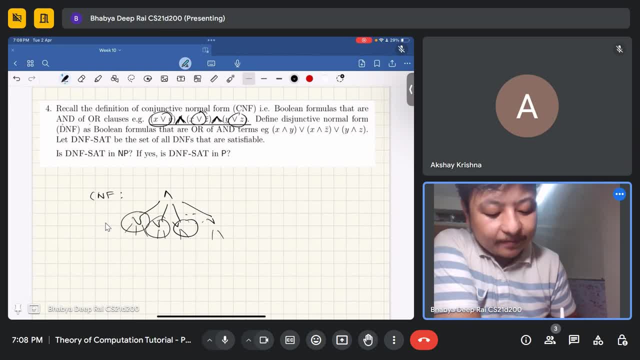 So each of these are ORs and then we are doing ANDs Right, so it can be seen as this expression can be seen as OR, x or y, x or z, complement and y or z. After finding this, it will be fed to the top AND gate and we have the same expression. 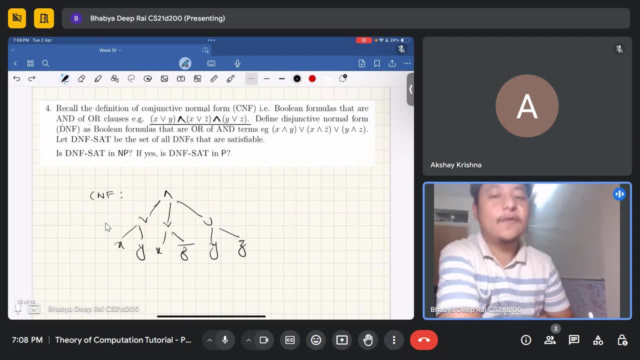 What is a DNF? A DNF is the opposite disjunct. in normal form, Top gate is the OR gate and the bottom gates are the AND gates. Okay, in other words. in other words, I'll do, AND first, then I'll do, OR. 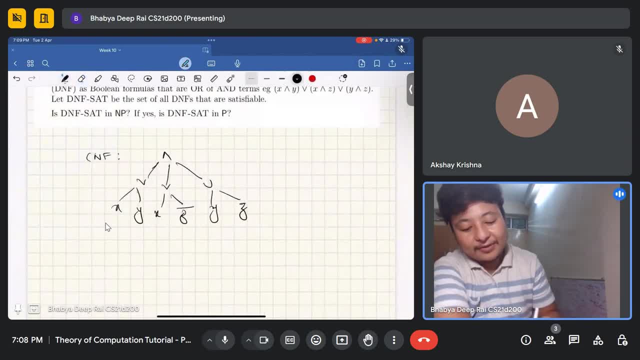 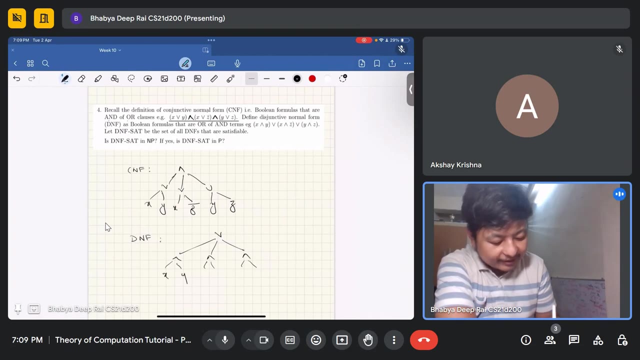 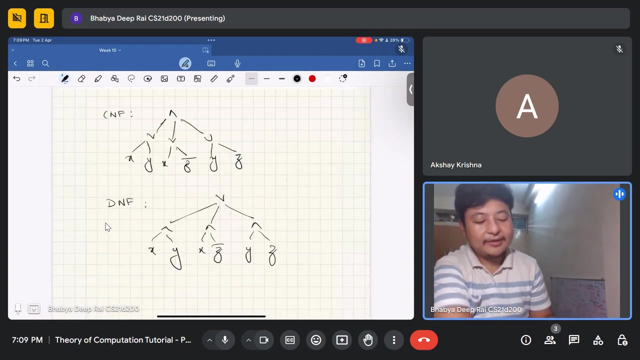 Before we are doing, OR first, then we will do. AND For example here DNF is OR, AND top gate is OR. bottom gates are AND. So this expression is X AND Y, X AND Y. X AND Z complement Y AND Z. So this is DNF. 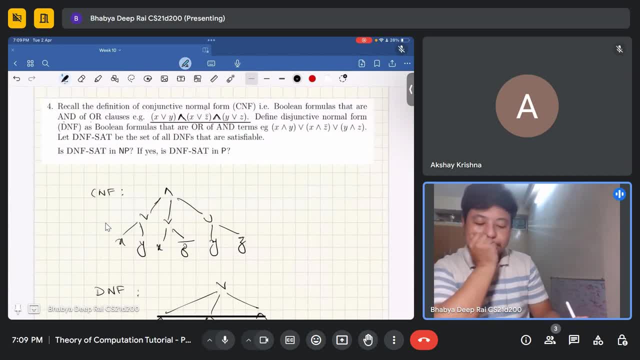 Now, what do you know about these? what do you know about CNF? We know that CNFs are actually very difficult to solve. What do I mean by solve? I mean satisfy. Satisfy means what is meant by formula is satisfiable. 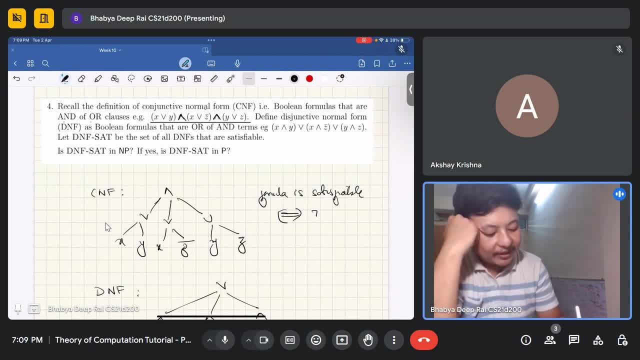 if, and only if, A formula is satisfiable. if, and only if, there is a set of inputs X, a formula F is satisfied, a set of inputs X, such that F of X is equal to 1.. Now we know that CNFsat, which is also called SAT, 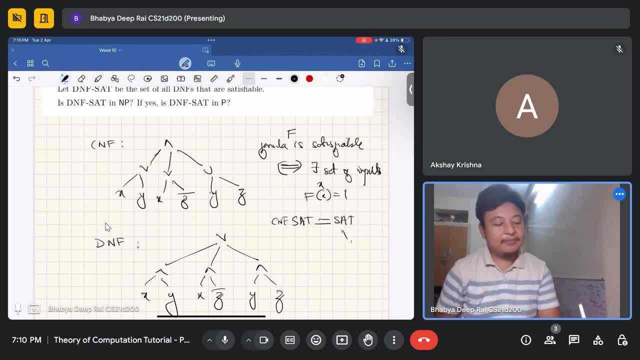 is very, very difficult to solve. This is NP complete. CNFsat, which is also called SAT, is actually NP complete. Okay, And this is very difficult to solve and it is not clear whether it is NP or not. It is in NP, clearly, because I can give you a short certificate. The certificate is: remember the exercise we did last time. 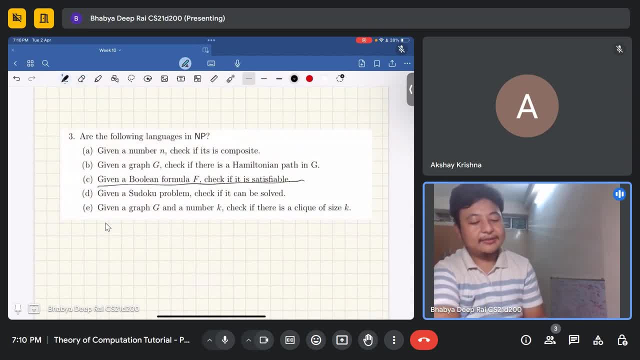 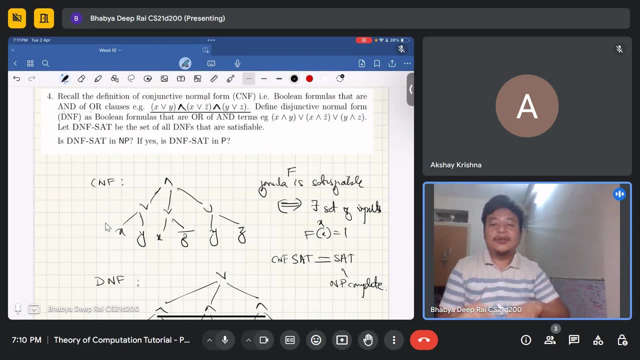 okay, this particular exercise, okay, the certificate is just the set of inputs. if i give you the set of inputs, you can just do the evaluation, you can do the or, and and so on and then say: okay, yes, this input satisfies it. so therefore, the formula is in np, sorry, the, the language is in np, so the 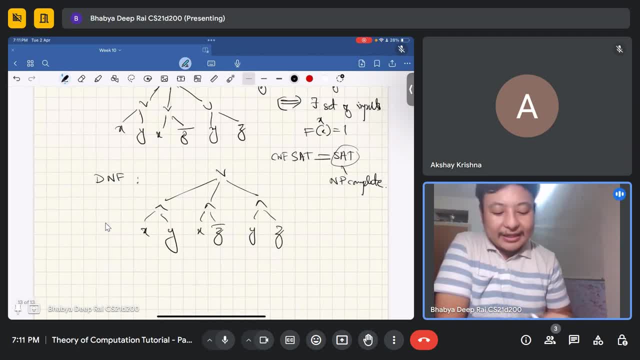 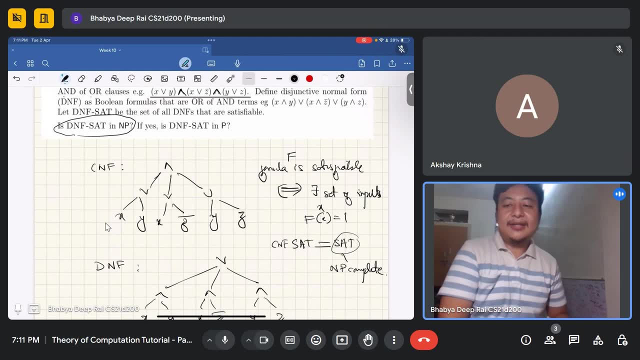 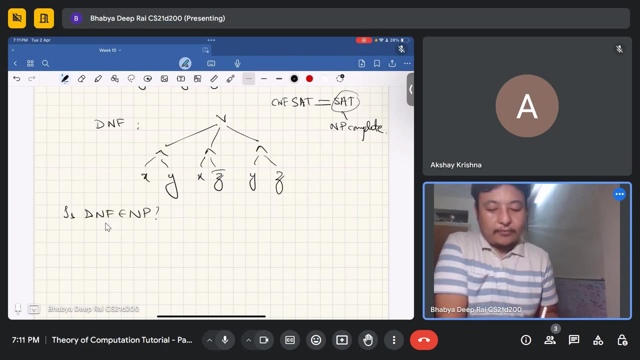 sat is in np. that is easily done. let's look at dnf sat, a close cousin. okay, in dnf sat is dnf sat is in np. that is the question. answer is yes. why is it in np? why is it in np? it is in np because 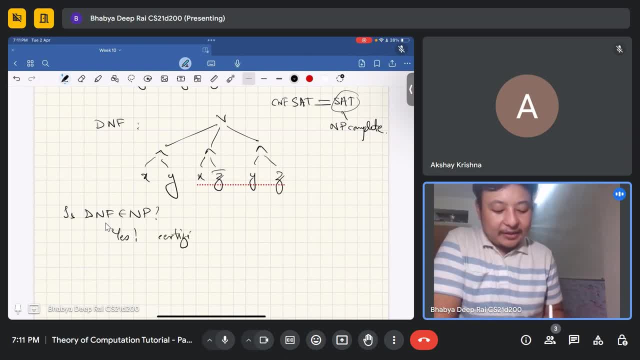 i can give you a small size certificate. certificate is nothing but the satisfying inputs, inputs that satisfy the circuit formula, the dnf, for example. here, if i give a 1, 1, 1, 0, 1, 1, okay and uh, 1 and 1 is 1, 1 and 0 is 0, 1, sorry, 1 and uh, 0, 1 and 0 complementing. 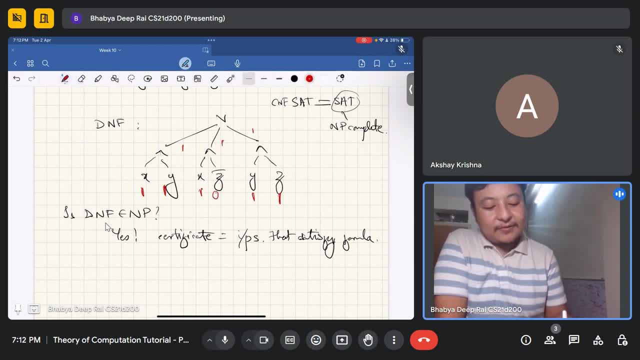 is 1 and this also gives one and the whole circuit gives one. so this itself is a certificate giving. i can give you this and you say, okay, i i'll run the circuit here because it takes it does not take much time. the entire circuit is of polynomial size and you'll run the circuit. 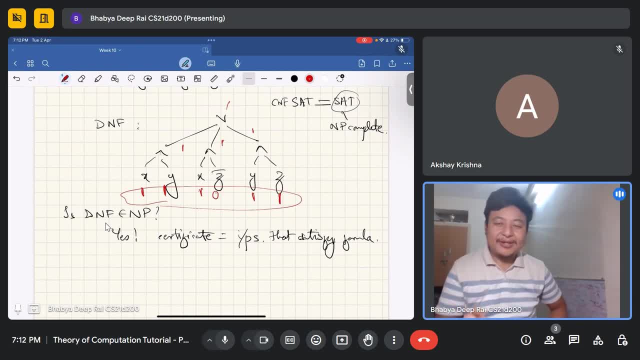 the formula- sorry, i'm keep saying so- the formula on uh, the inputs, okay, and i'm getting the output of the formula as one, which means that the circuit is satisfiable, and this is a valid certificate. right, a certificate that satisfies my formula is a valid certificate for certifying that uh, this language, whether my uh formula is satisfiable or not, is in. 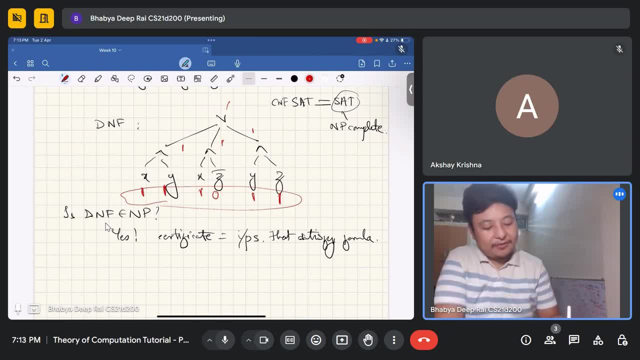 np because of the definition of np. therefore, uh, if i okay again to explain it, to check whether uh, dnf or formula is satisfiable or not, it is enough for me to give you a satisfying assignment. okay, so now the satisfying assignment i can easily give you. this is a small size certificate. what is the length of the certificate n, which is polynomial? 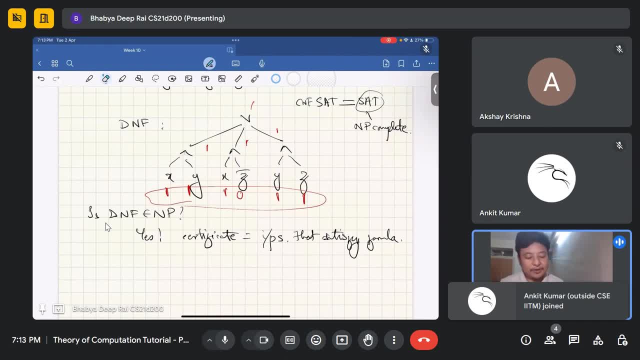 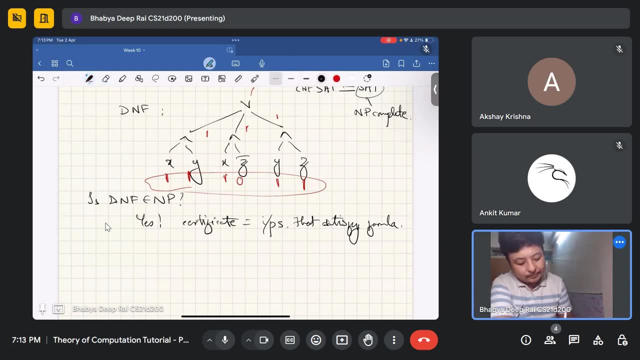 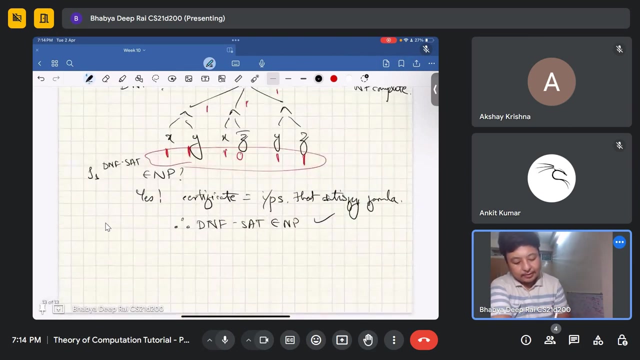 size, okay, uh, which is polynomial size and therefore circuit. therefore, dnf sat- okay, sorry, not dnf. dnf set is in np because it follows the. now, uh, the question says: if yes, is dnf sat in p? this is the question. now, let's see. let's see. okay, here is the. 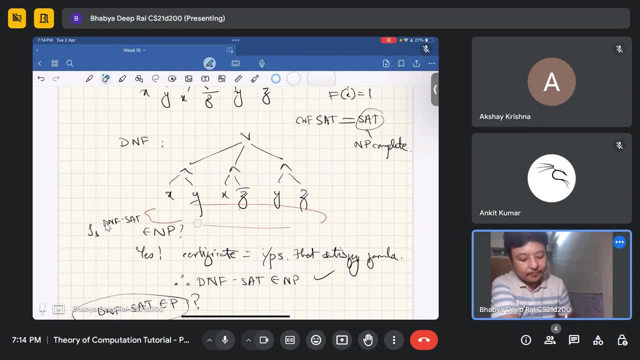 um formula we are given okay. so i i ask you, give me any uh input that satisfies this formula. give me any input that satisfies this formula. so, uh, you can give me. suppose say you say okay, sir, 1 and 1 and 0100 will satisfy this. 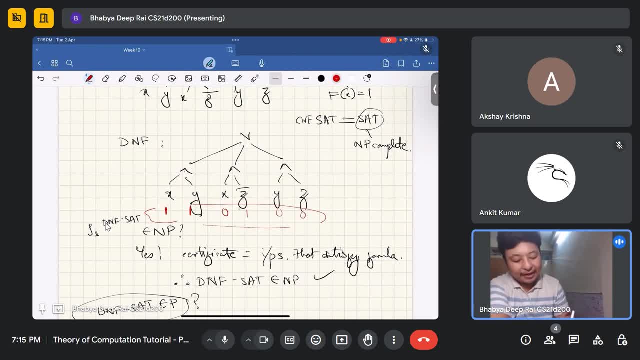 and then i evaluate this: okay, one and one will give one, and then, because of this, or i'll get a one and uh, someone else. okay, may also say, uh, one and y as one, z as one and the other as different. okay, some other cases will give. 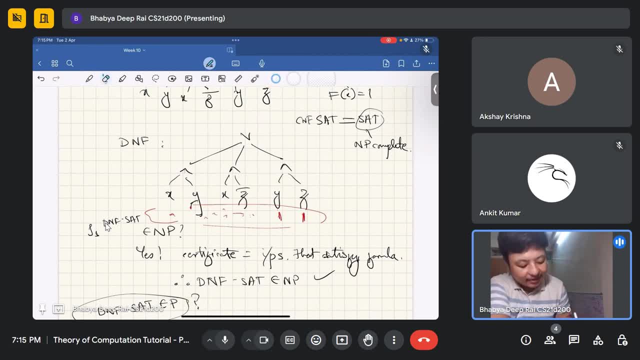 me one and i'll still say yes, that is true, because and evaluates one one and one is one, and then, or okay, as long as there is at least one one, then i'll give an output one. so what is my observation here? my observation is: as far as i can satisfy any one of these small clauses, any one of these small 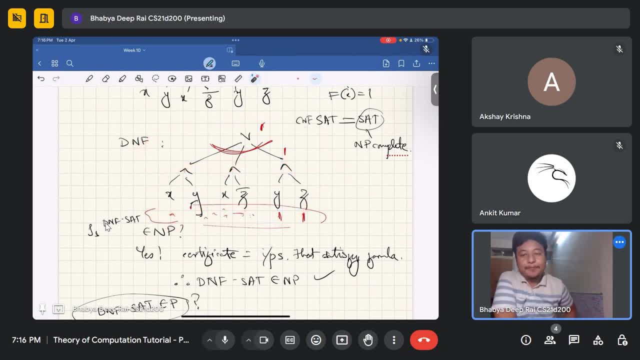 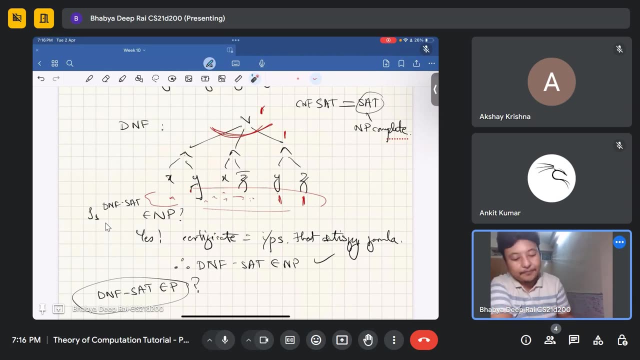 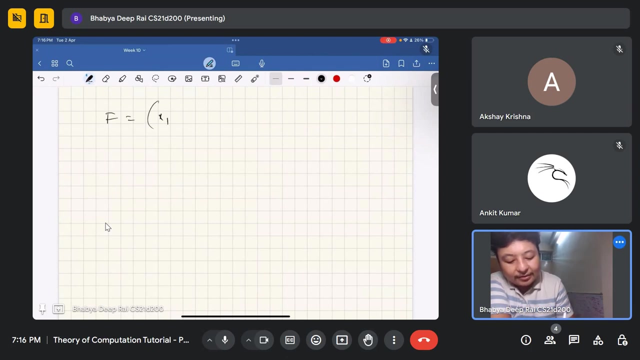 hands, i can satisfy the entire circuit. that is the observation here. okay, so what? i'll call the each of these as are clauses. they are technically, they are called as clauses. okay, so, uh, f is of this form, you know, x1, okay, i clause 1, and clause 2, and clause 3, and so on, and each of. 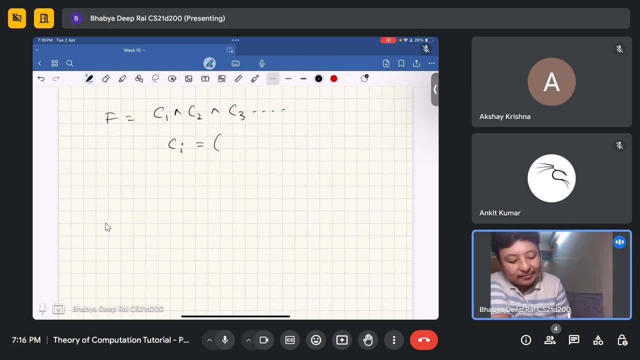 the clauses. clauses are of the form x1 and or x2 or x3 and so on. this is what each of the clauses are. these are called clauses. okay, each of them are of the form wars. my observation is that any clause satisfied, then if, and only if, entire formula f satisfied. 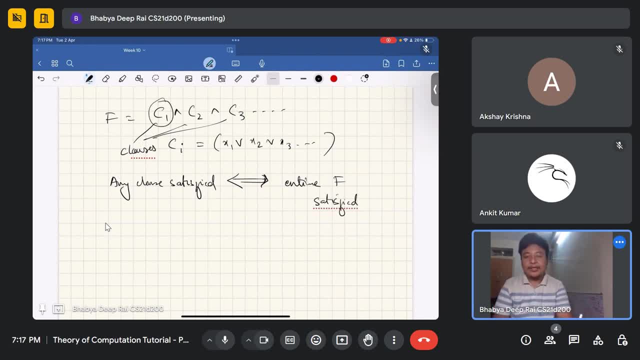 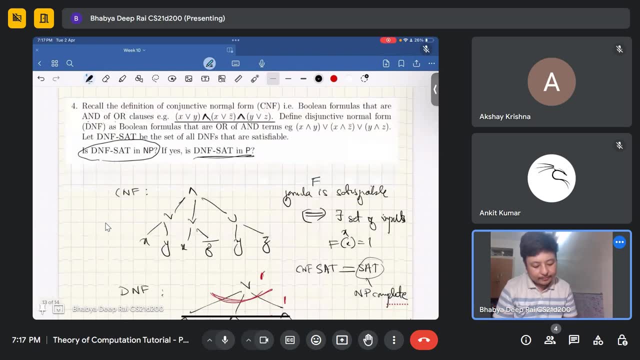 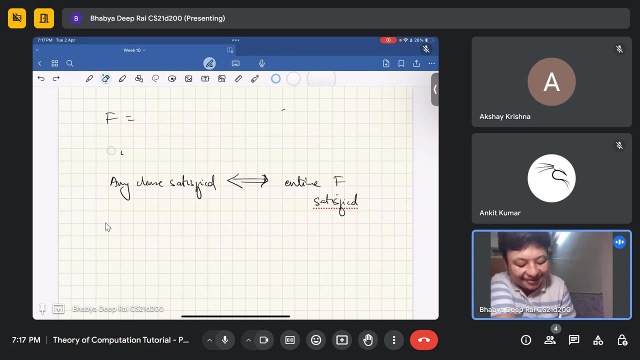 because if i satisfy a single clause, okay, then okay, what did i do? okay, sorry, sorry, sorry. it's not a clause, it's a term. i'm sorry, really sorry. we are doing and of course we are doing or gate at the top, so i'm not going to call it clause. these are called as terms, okay, not clauses. 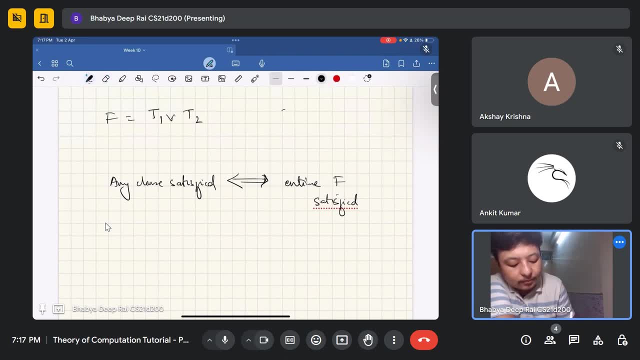 these are called as terms and these are called terms. each of these terms, okay, if, and each term is of the form uh, x1 and x2 and x3 and and so on, and if i satisfy any of these terms, my entire formula is satisfied, right, because of the property of r, even if one of these t i's. 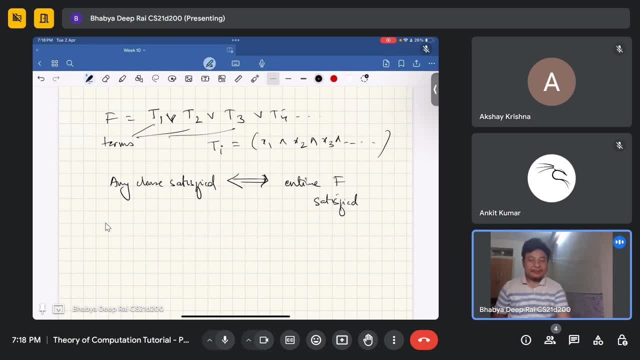 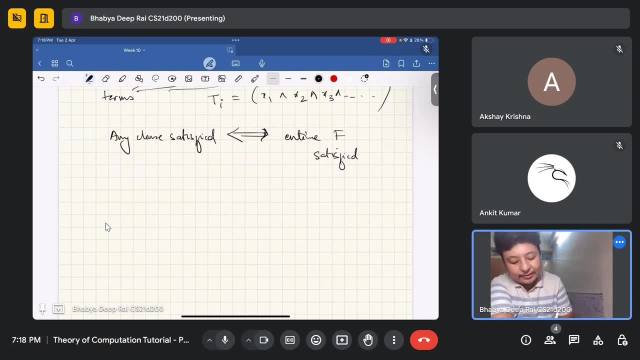 are satisfied, then my entire formula is satisfied. so that is my aim. now i want to satisfy one of these, any one of these, so what i'll just do is i, my algorithm or my deterministic polynomial time turing machine? okay, interchangeable is as follows: pick a term, any term- t, i, which is of the form x1. okay, i'll write it as l1 and l2 and l3, and so on. 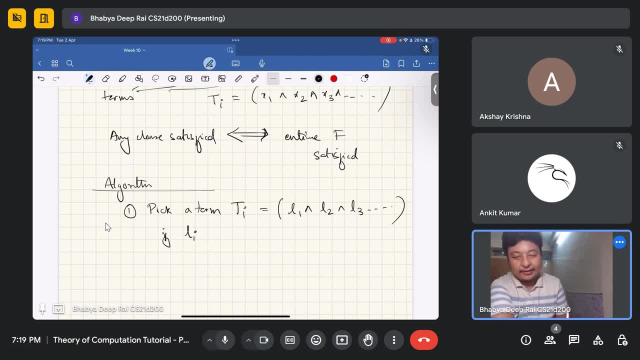 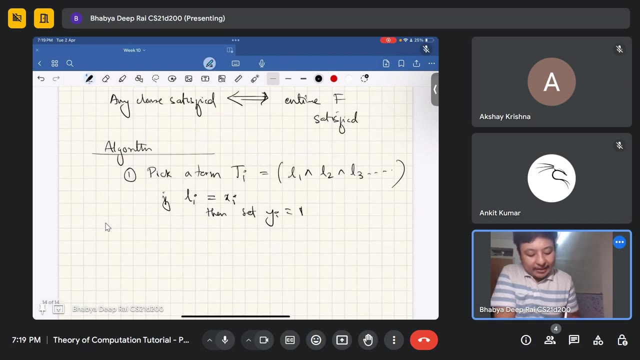 if li equals xi, okay, it is a positive literal, it is not negated, no negation gates. then set y i equals one. and if it is a negative literal, li equals not of xi, xi bar. okay, then set y i equals zero, then my y1, y2, and so on till yn satisfies. 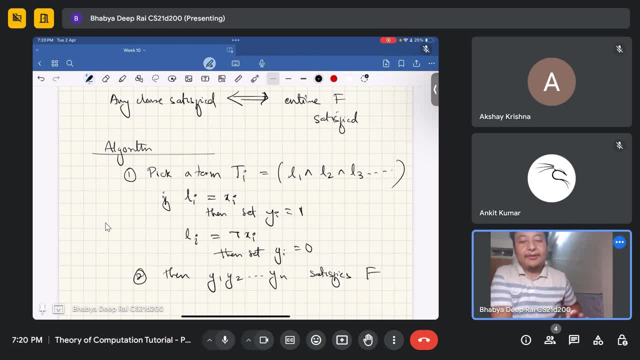 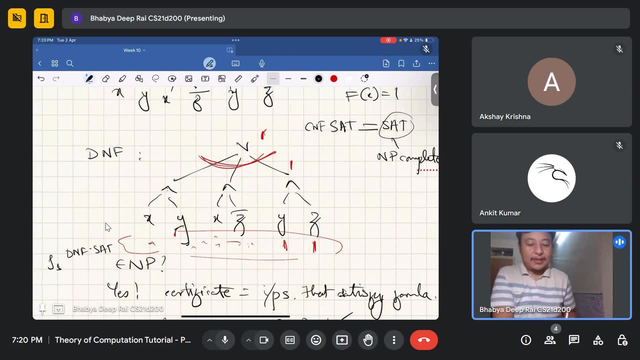 f. okay, this is not entirely correct. okay, but what? what? what? the logic was here is: i want to satisfy any of these terms. okay, i want to satisfy any of these terms. and how do i achieve that? well, i, i want to satisfy this term. what i'll do is: i'll set. 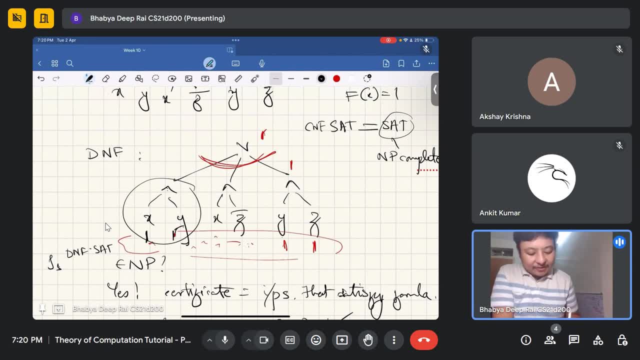 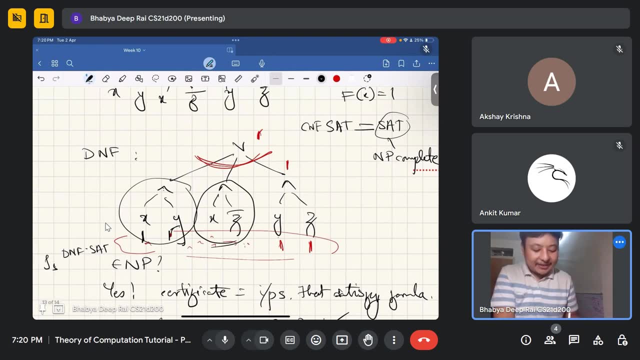 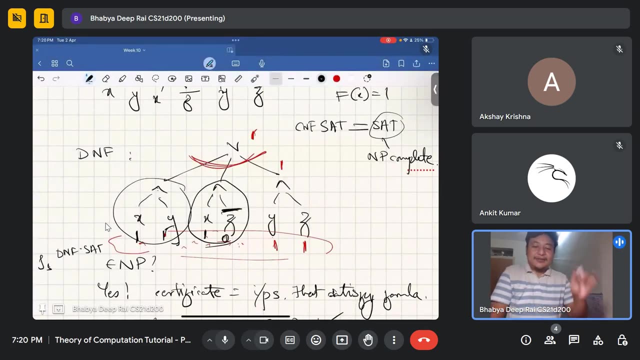 x to one, y is one good. if i want to satisfy, say, this term, what do i do? if it is a positive literal that is no negation gate is there, then i'll set it as one. if it is a negative literal that there is a not gate here, then i'll set it as zero. then this term is satisfied, right. 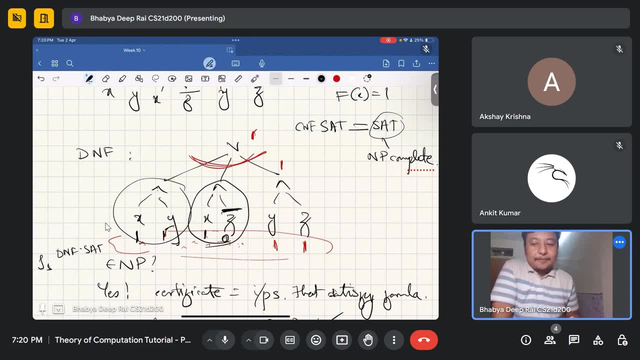 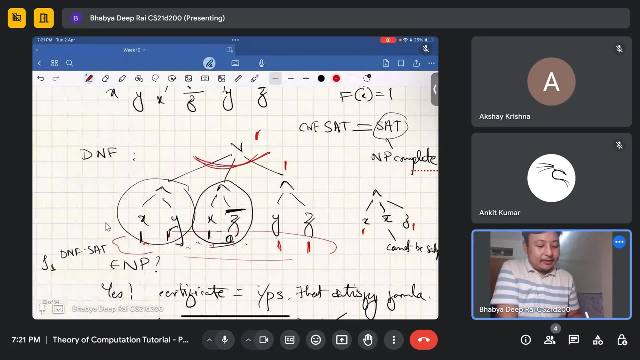 that is the logic here. and what kind of terms can i not satisfy? i cannot satisfy tomes as follows: x, x bar z. this storm cannot be satisfied. why? because if i give it a give x a 1 and z 1, um, I need to give this a 0. 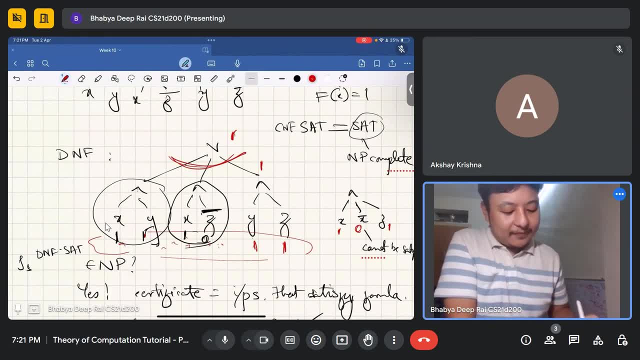 Okay, but this is a problem, right? I cannot have x being 1 and 0 at the same time. I cannot have x being 1, both 1 and 0 at the same time, So this cannot be done. 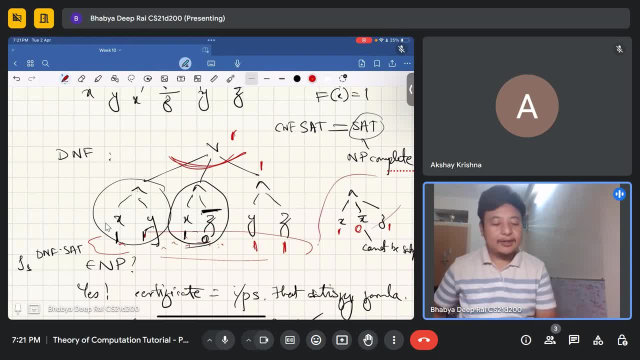 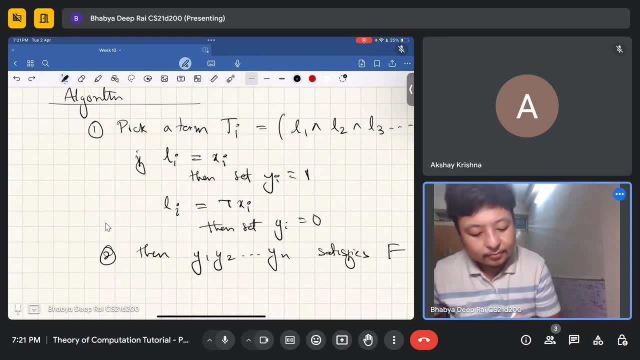 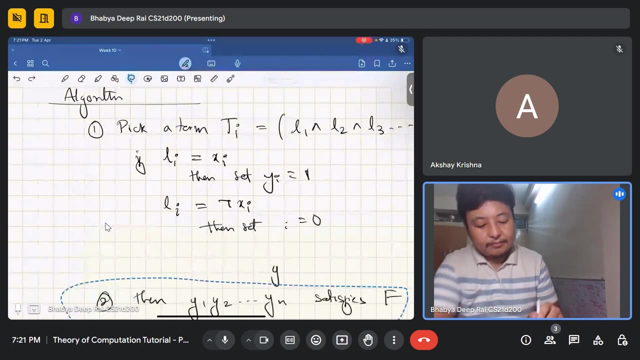 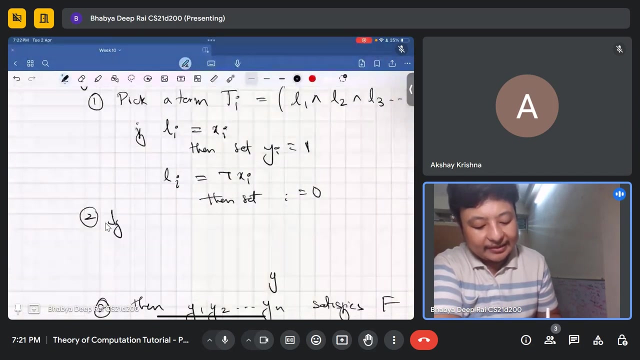 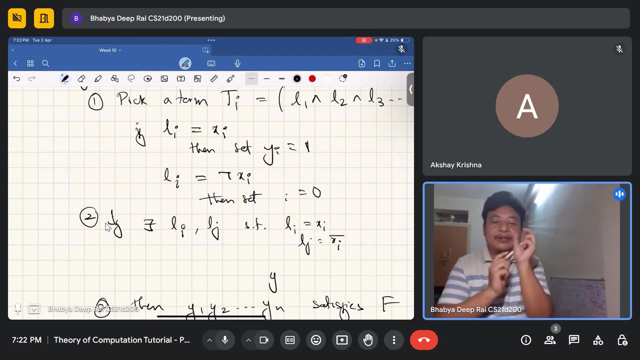 So this is a bad case and this is what we want to avoid. So what I'll do is, finally, if there exists L i, L j, such that L? i equals x i and L? j equals j equals x i, bar if in the term both the positive and negative literals of the same. 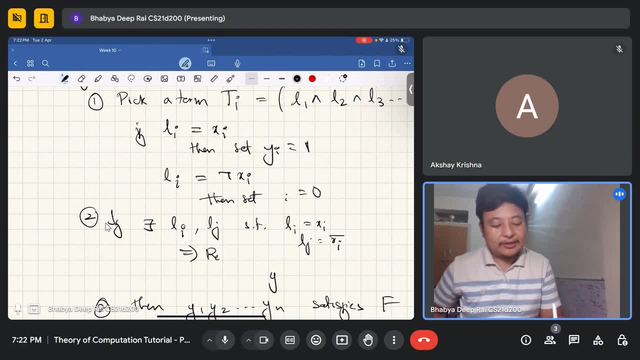 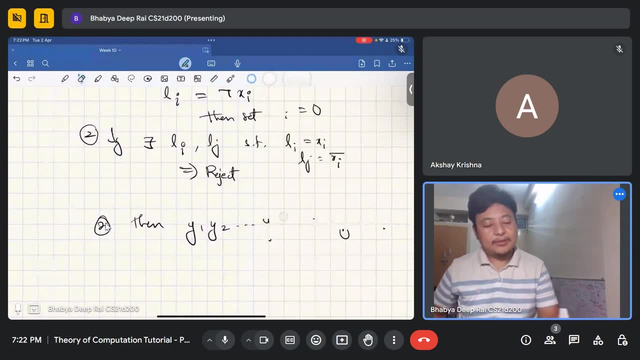 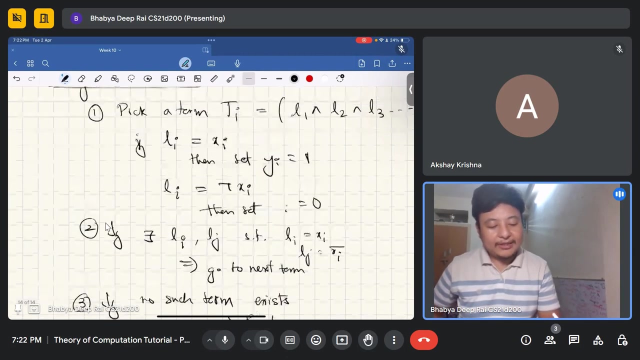 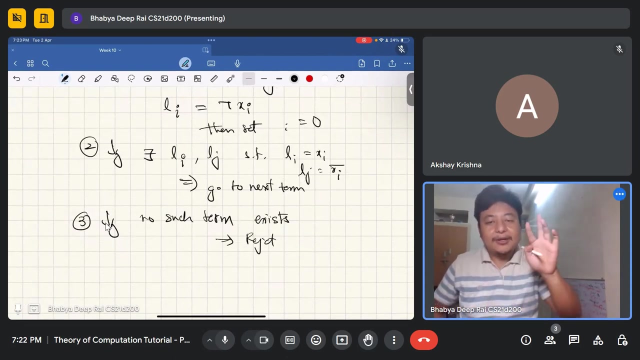 variable exist, then reject Okay. and we don't need this. Oh not reject, sorry, sorry. then go to next term. If no such term, satisfiable term- exists, okay. no such term exists, then reject Okay. otherwise if I had found such a term where you know x, i, x, i bar, this is not. 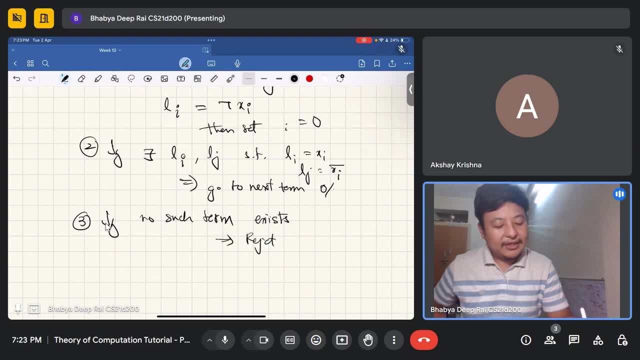 present, then I can always satisfy this term, Otherwise accept Getting it. So this is my final algorithm, Simply to state it. I just go across each term. I try to satisfy that term. If that term is not satisfiable, I'll move to the next term. 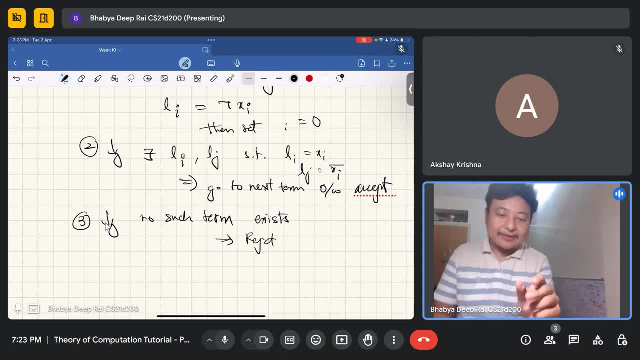 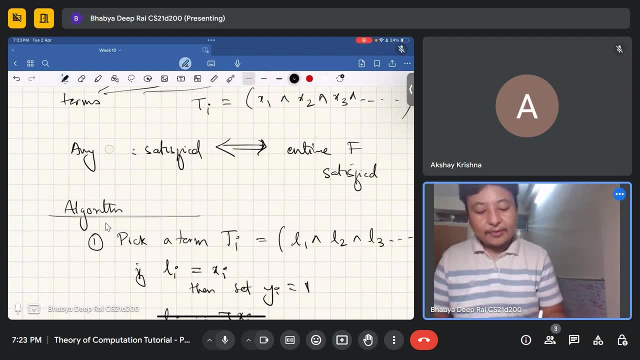 If that term is satisfiable, then I'll simply accept, Because if I satisfy a single term, see if there is any okay not clause, sorry, any term that is satisfiable. If that term is not satisfiable, then the entire f is satisfied getting it. 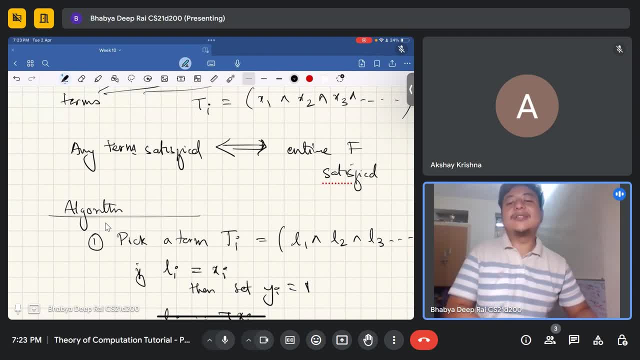 And if I don't find such a term, then I'll just reject it. Because f is not satisfiable, then because I can never satisfy that term. okay, is that clear? Yes, sir, Okay, good, Okay. so there is one question that I wanted to ask you. 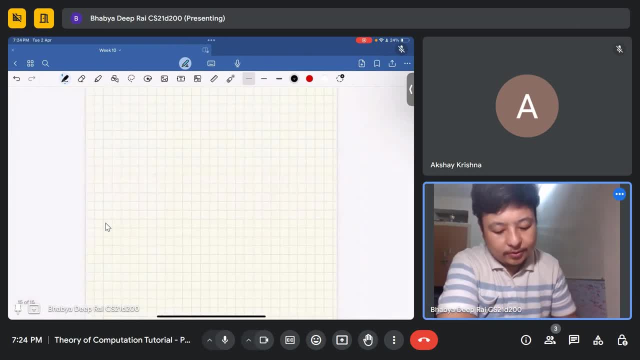 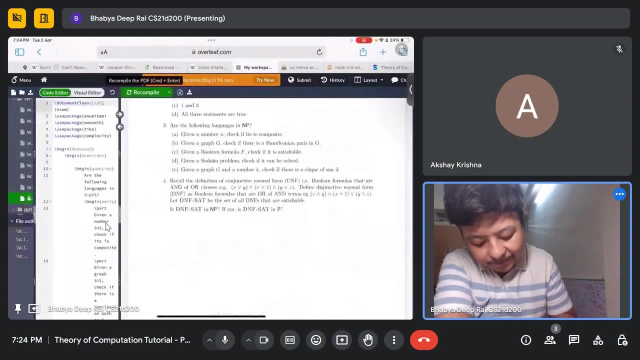 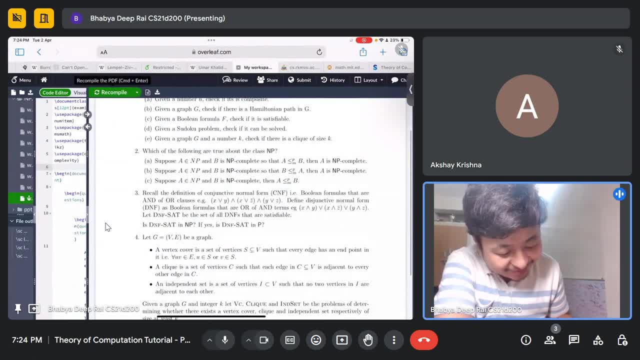 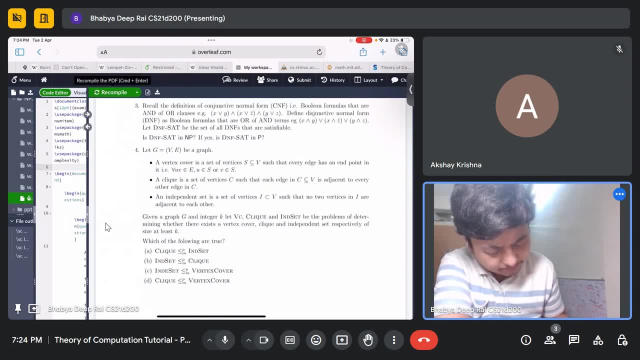 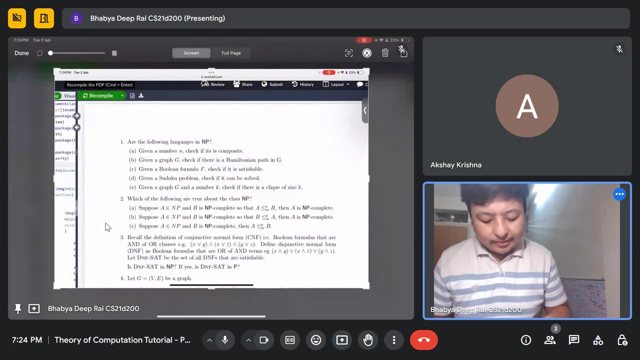 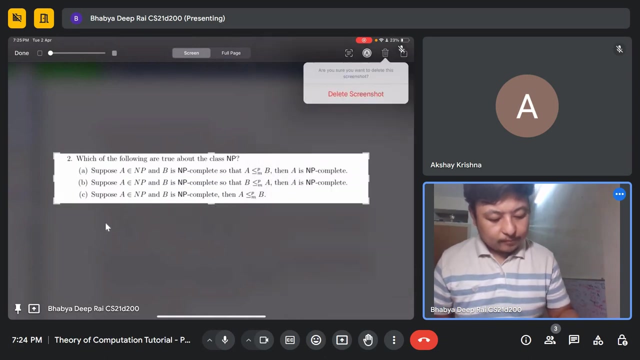 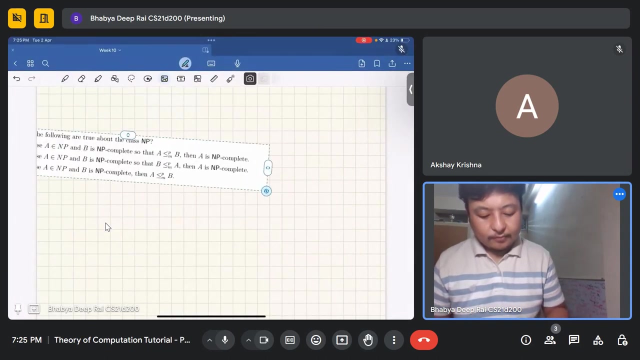 Hmm, Okay, Okay, Okay, Hmm, Mm-hmm. question is: which one do i do? because this will take some time. okay, so i'll do the simpler question. okay, then we can call it a day. so this is about completeness. okay, just a quick question, it's not? 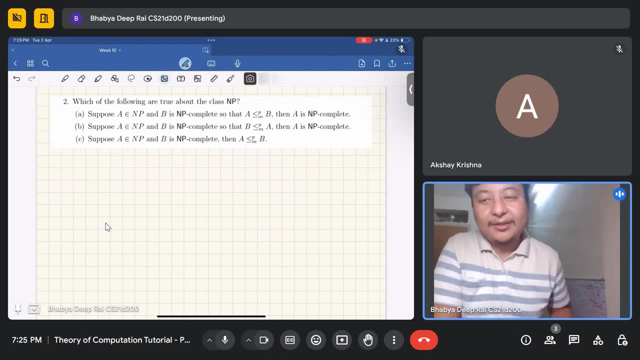 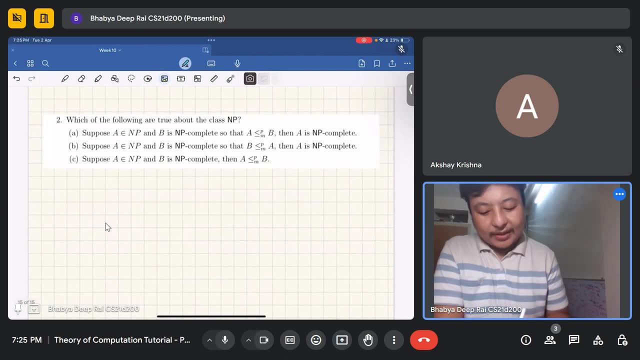 twisted. maybe the next one will take some time, so maybe the next one, i don't know- next one, but here is a question, uh, which of the following are true about the class np. so this is. i just want to make sure that this question is covered. to understand reductions. 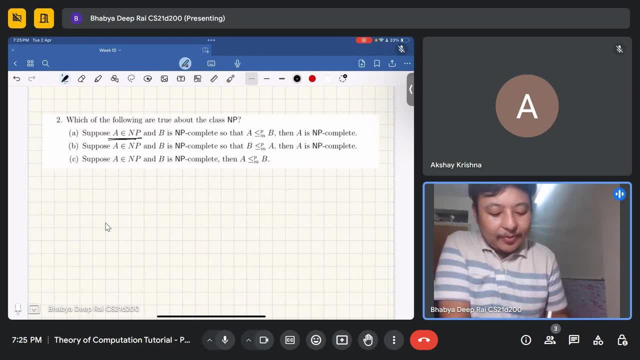 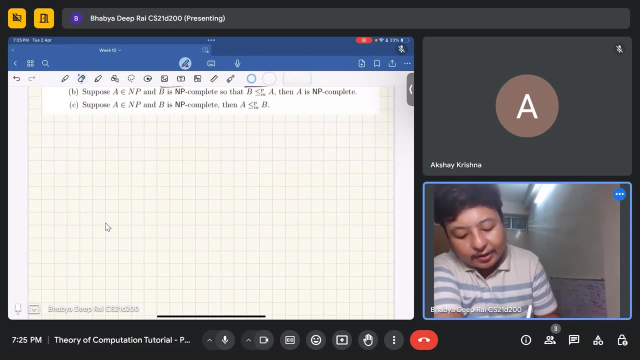 properly suppose a is an np and b is np complete, so that a reduces to b then. So, first, what is NP-completeness? first of all, what is reduction? We say that a polynomial time many one reduces to b if there exists a transformation f such 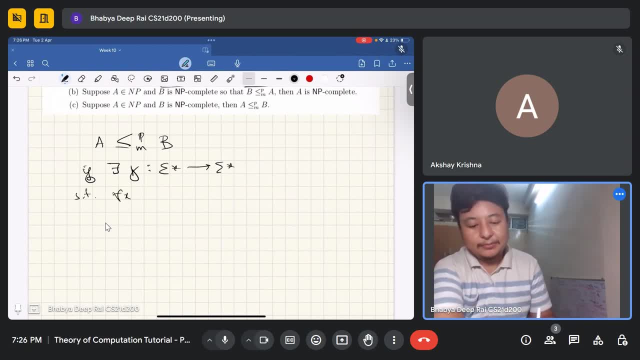 that for any x in sigma star, any input. if I want to check whether x belongs to the first language, it is as good as checking whether f of x belongs to the other language. So I am transforming one language to another and this is called a reduction this f has. 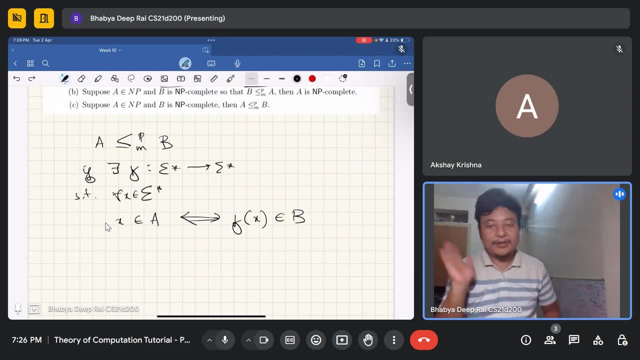 the special property, it is called the reduction. We were doing it before in the computability section also using that halting function problem and so on. So we do this small surgery kind of thing so that if I have an algorithm for a, I can. 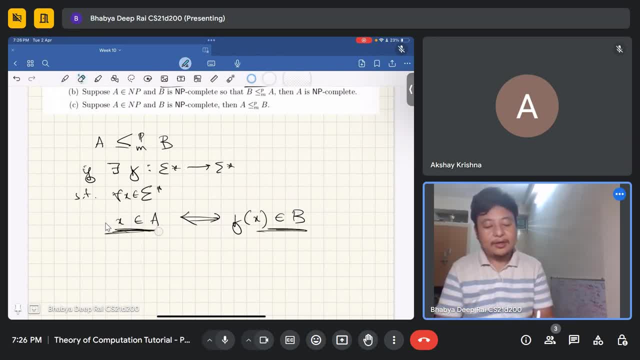 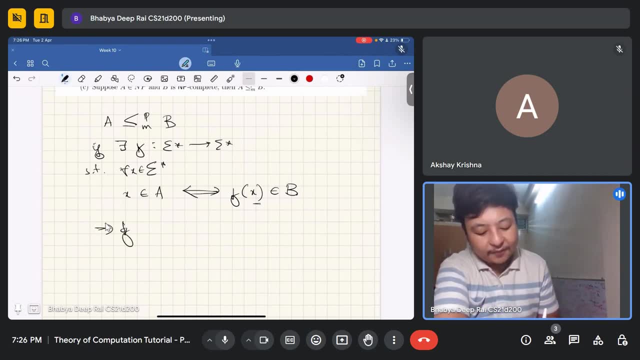 have an algorithm for b also. So this is what it means. now it means. what does this mean If b can be solved easily? furthermore, f of x is computable. So if b can be solved in p time- deterministic polynomial time p- then what I can do is 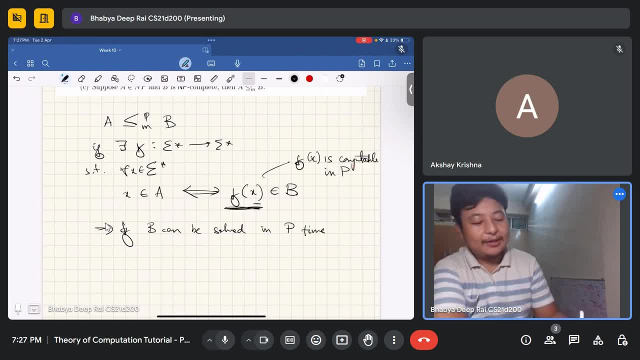 this transformation, I can do it in polynomial time, and then I can decide f of x in p time, and then that would mean that I could answer yes or no even for x- sorry, even for a. So if b can be solved in p time, it means that a can be solved in p time. 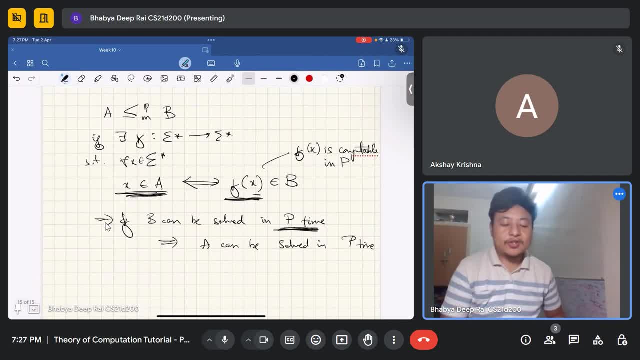 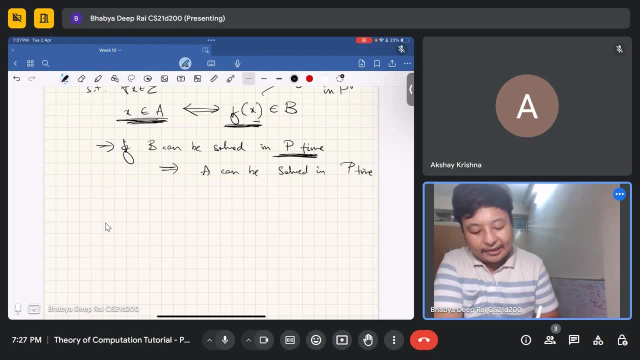 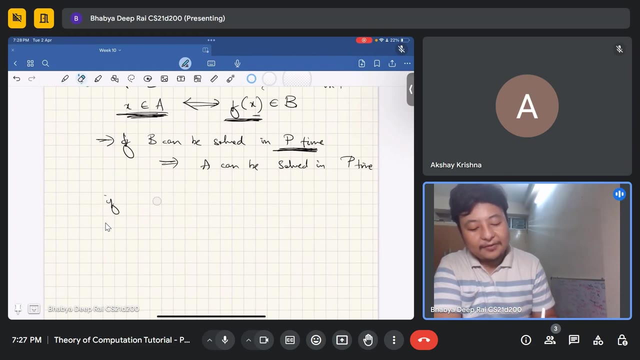 So this has been the go-to approach to check whether p to resolve the p versus np conjunction. The idea is that if I have a very difficult, the most difficult language in np, if I have a b, Suppose b is the most difficult language in np and I show that b actually reduces to. 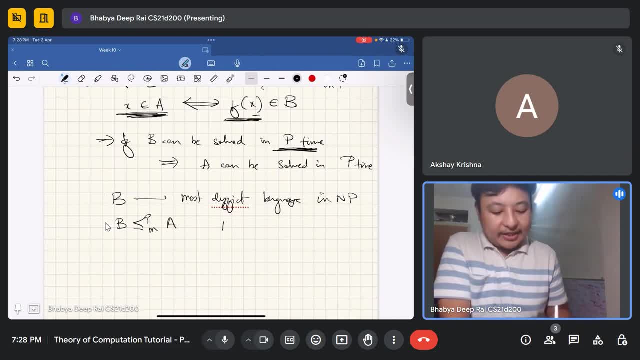 a such that a is in p, Then because of this result, It means that b is in p, but since b is the most difficult language in np, this means that p equals np. I mean kind of hand wavy, but this is the idea. 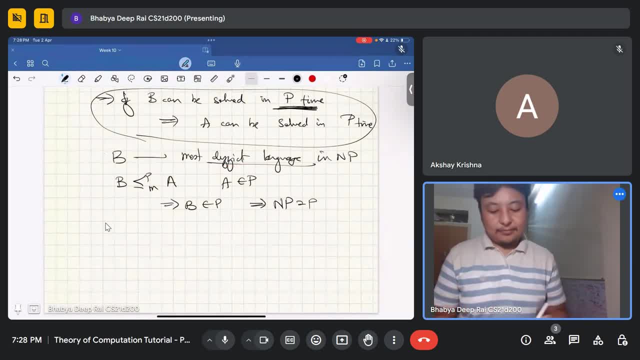 So what? what are the most difficult languages in np? that is the question: What is the most difficult language in np? These are what are called np complete languages. How are they defined? How are they defined? Ok, They are defined as follows. 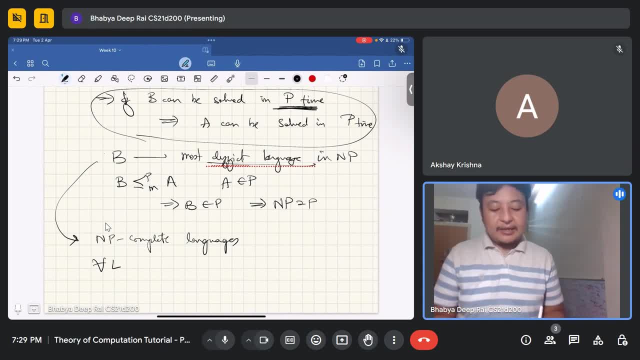 For any language, l in np l many one reduces to b, Then b is np complete If, and only if, b is np complete. So All of the languages in np boil down to this np complete language. Then it is called np complete. 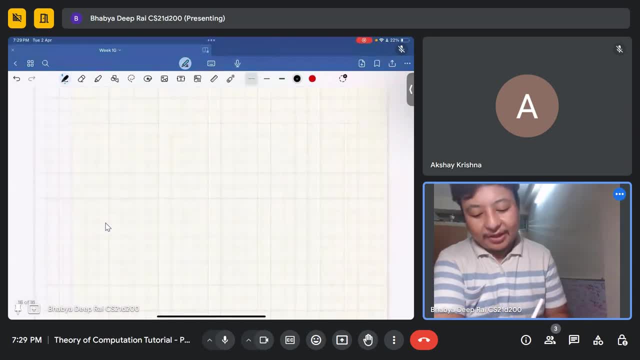 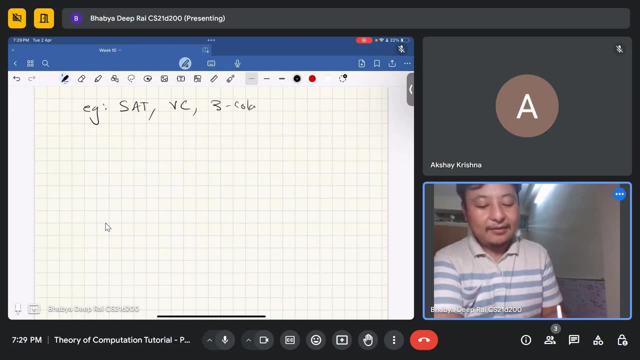 Ok. So, for example, what did we have? example, we had sat vertex cover, some free coloring, and you saw other examples right? So any language in np can be converted to a version of satisfiable. it can be converted to a formula. 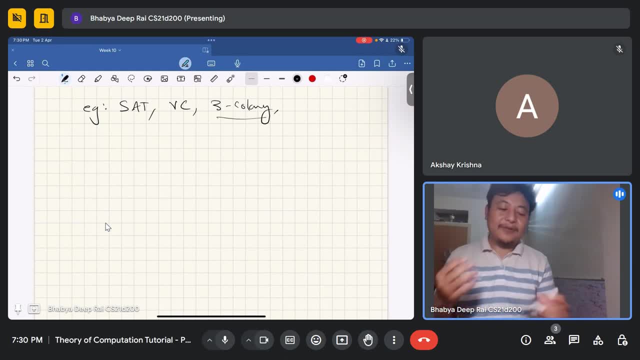 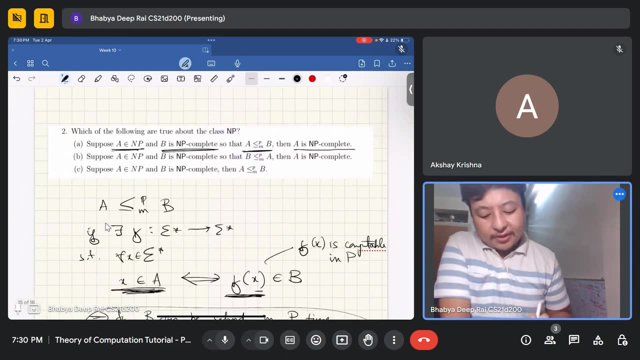 You can check whether it is satisfiable or not. It can be converted to a graph where you can check whether it can be colored by three colors or not, and so on. You can transform it. Ok. Now the question is: suppose a is in np, p is np complete? 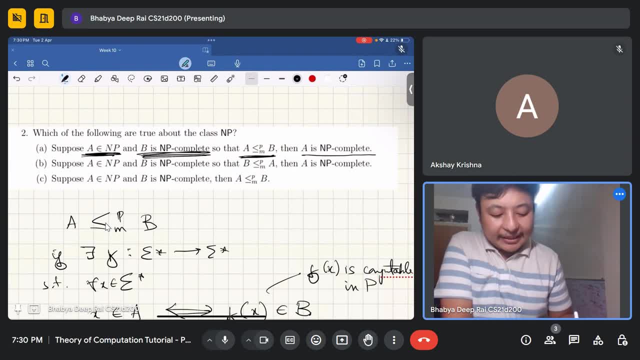 So that a many one reduces to b, then a is np complete. Ok, That is the question. Is this true? This is not true? Ok, Because, oh yeah, sorry, this is true because b is np complete. oh sorry, what am I saying? 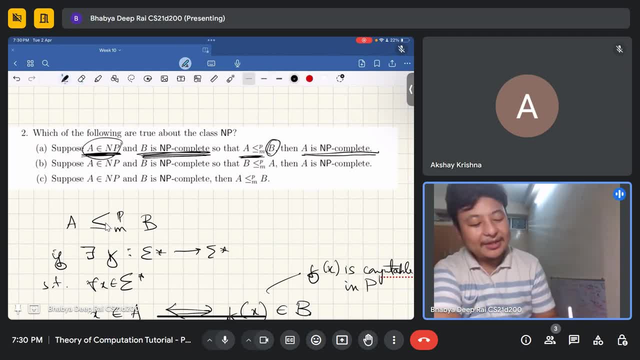 man, b is np complete and a is in np. ok, b is. oh yeah, b is np complete and a is in np. already means that a reduces to b, But this does not mean that a is np complete, right, Because 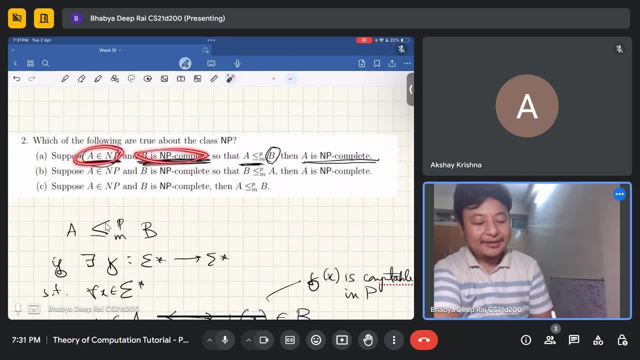 If this is true, ok, b is np complete. a is in np. we already know that this is there. If this were to mean that a is np complete, then this would mean that all the languages in np are np complete, which is not known as of now. 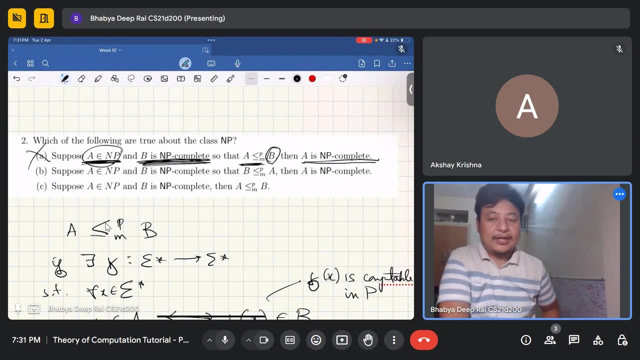 So this is not true. At least it is not known that it is true. Now the next question is: suppose a is in np, b is np complete, so that b reduces to a, then a is np complete. Ok, So b is np complete. a is in np, then is a in np complete. 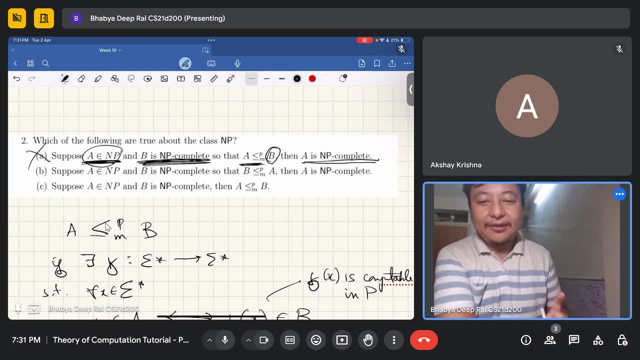 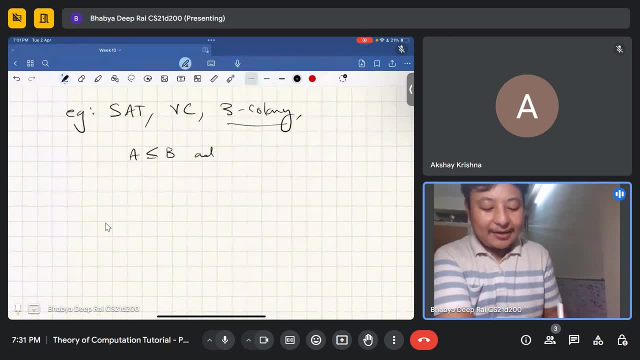 The answer is yes, Because of transitivity, of reductions. ok, because we have that. you know, a reduces to b and b reduces to c, then a reduces to c, kind of thing. no, What we are saying is now. what we are saying is: a is in np, b is in np, a is in np b. 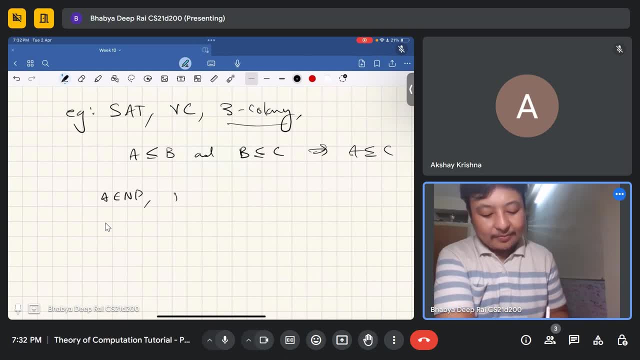 is in np And b is np complete and b reduces to a. ok, b reduces to a. this is a standard result. ok, This is what is done in the lectures. So b reduces to a and b is np complete. 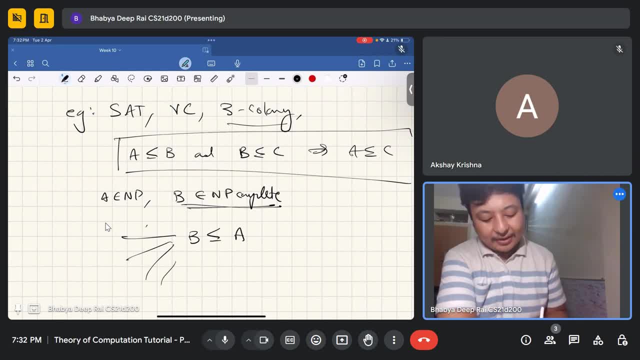 What does this mean? This means all the languages reduces to b, For all li in np. all of them reduces to b. Ok, And now we are saying b reduces to a. This would mean that since l1 reduces to b and b reduces to a, it means l1 reduces to.